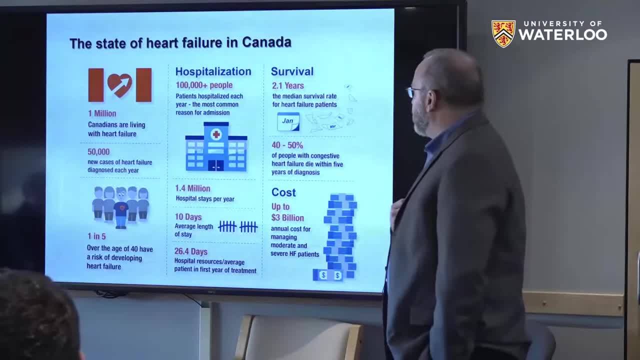 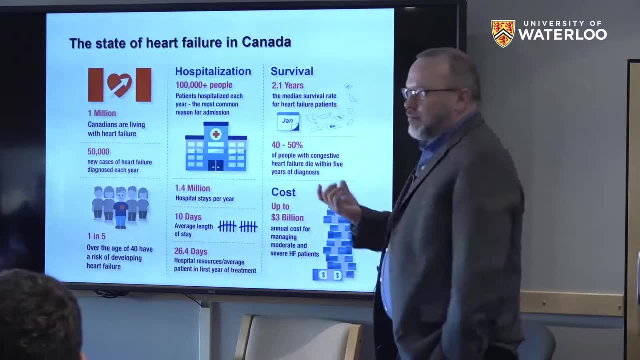 the body. It's really approaching epidemic proportions, both in Canada and worldwide: A million Canadians living with heart failure, 50,000 new cases each year. It's one of the main causes of hospitalization and you can see the days in hospital are very long and 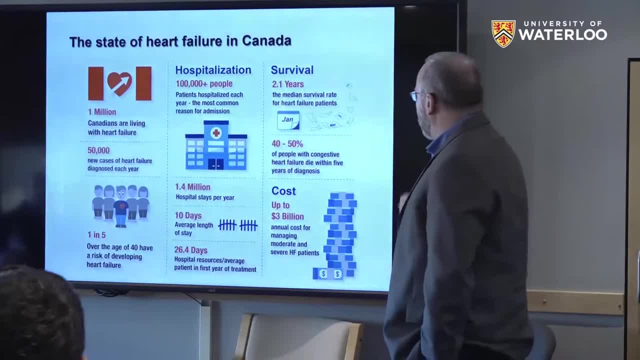 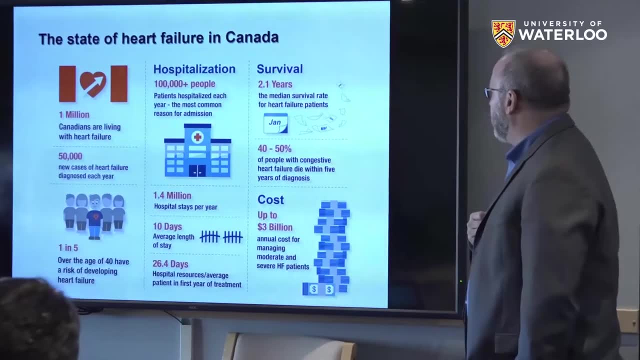 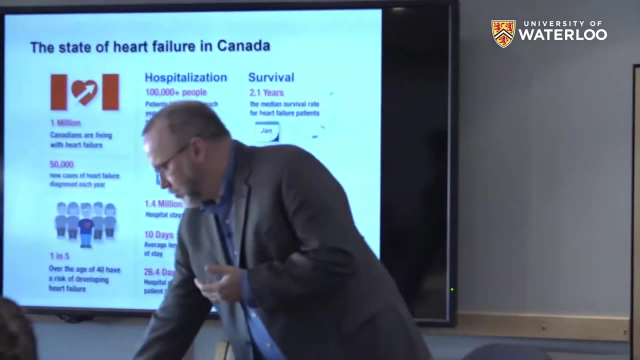 the resources dedicated to this are very high, And if you have heart failure, the survival is much shorter than most cancers, And so it really is an important problem economically, socially and health-wise, and is one that we're entirely focused on, And so TBEP, our mission, is to take a multidisciplinary, collaborative 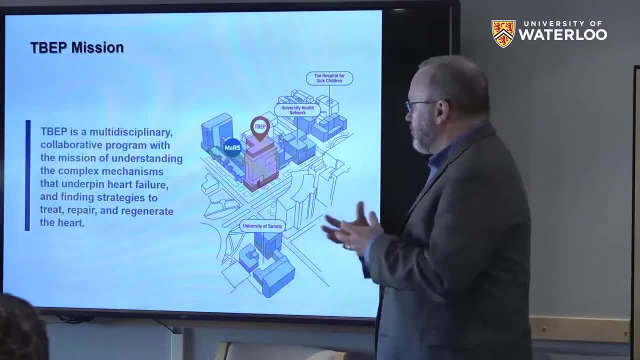 approach to this problem and to really understand first what are the mechanisms that underpin this failure and what are strategies that we can develop to treat, repair and regenerate the heart. And we're located slightly off campus, so main campus in Toronto is here. We're kind. 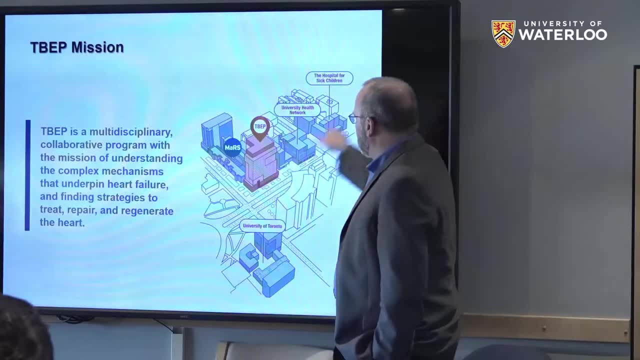 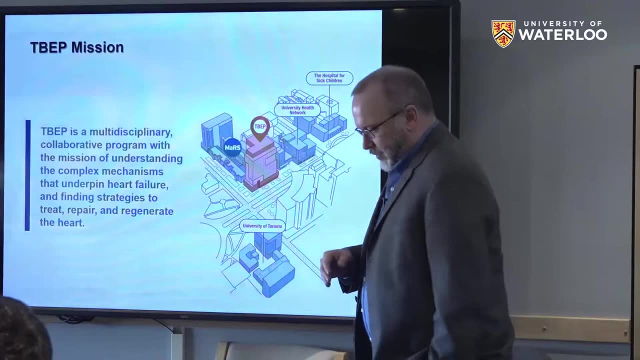 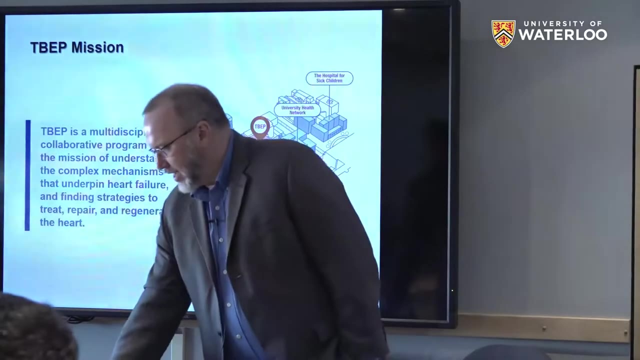 of across the road in a building here, but nicely situated close to our hospital partners, close to a within actually a technology transfer space called Mars, and then close to campus. And we're right now we have eight members in our group, eight labs, that all kind of 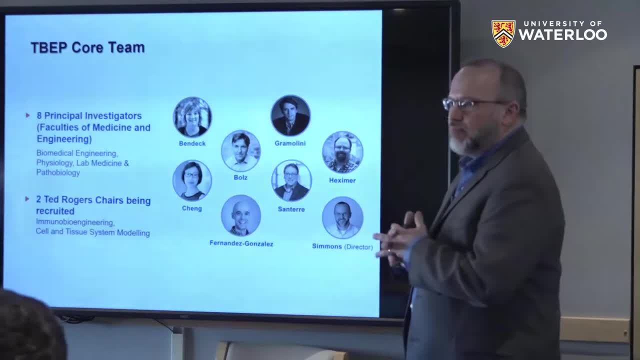 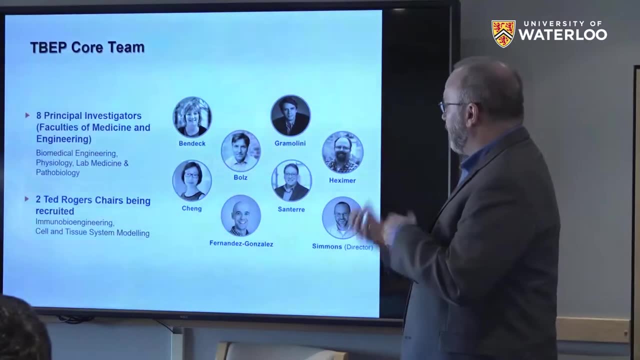 come together. We're split between medicine and engineering, so we're completely embedded together. And this is really, you know, brought new insights for us from hearing the medical perspective and from us to them, And so it really has been eye-opening for us and we 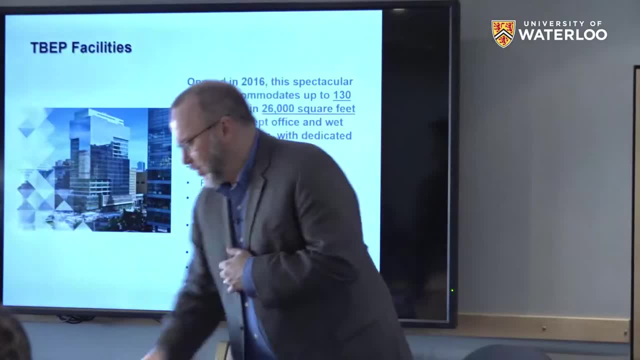 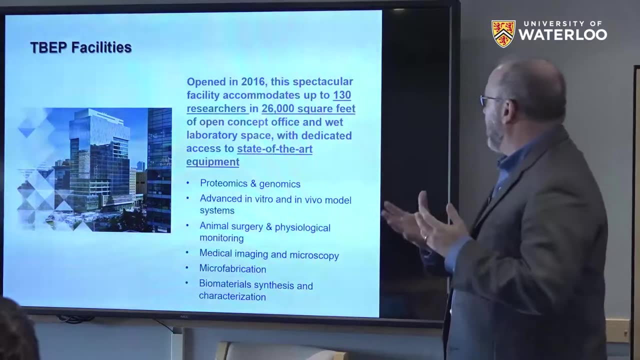 are recruiting two more chairs And, as I mentioned, we sit on the 14th floor of this building. so we're up here. We have a single floor, 26,000 square feet, where we have up to 130 researchers with a broad 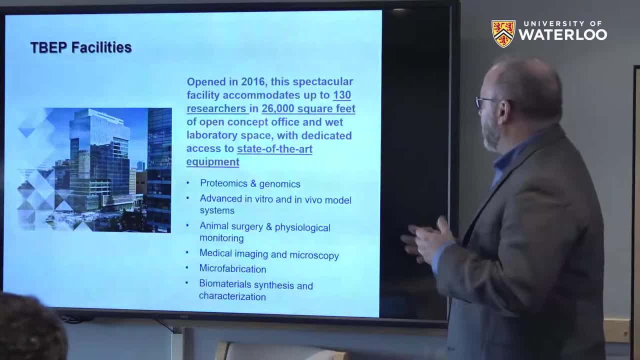 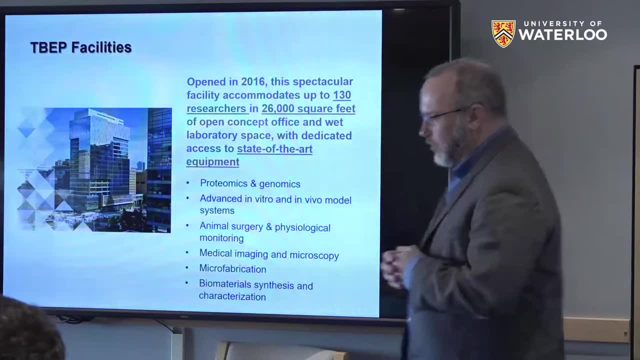 range of facilities and equipment that are all shared, And so this highly collaborative spirit is also in in in how we work, Thank you- And really has enabled us again to do things that we hadn't hadn't been able to do previously. 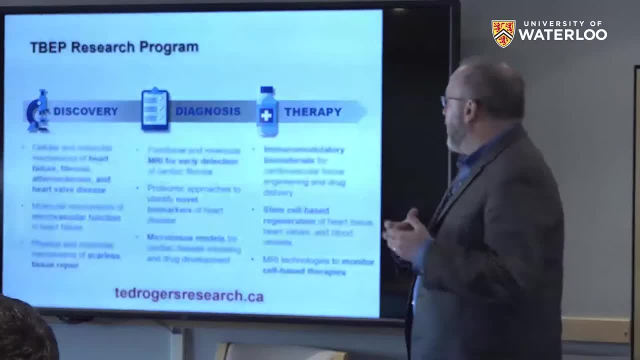 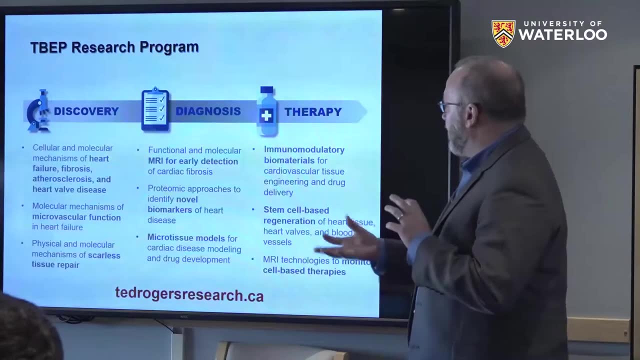 And our program spans all the way from discovery science all the way to therapies, And so you can see the broad range of work that we're doing there. But again, engineers, scientists, basic scientists, applied scientists- all coming together to tackle these problems. 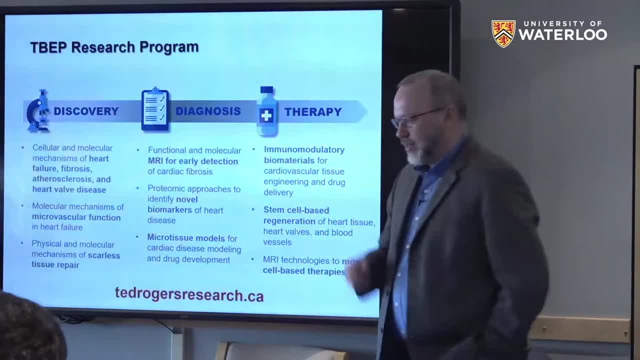 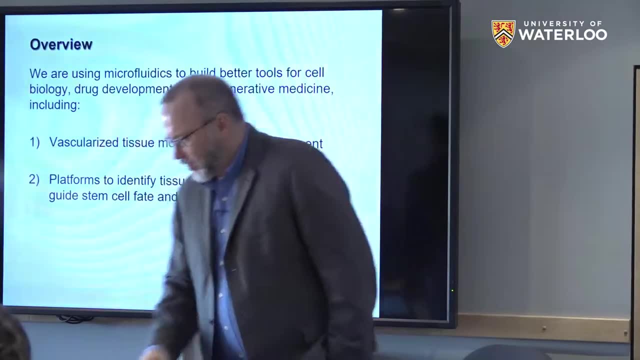 So if you want to know more about the pro program, link is there. We we have lots of students on the pro in the program, post-docs and so on, and always are recruiting. Okay, so what do I want to talk about today? So this is just an overview and kind of summary. 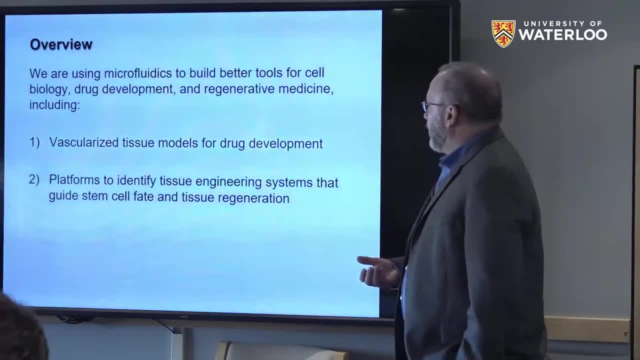 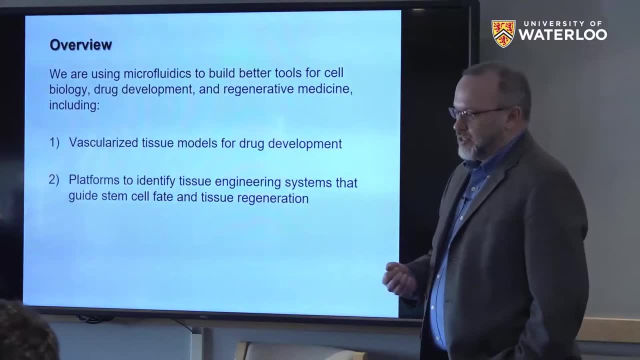 I'm going to talk about our work using microfluidics, that we are hoping to build better tools that allow us to do cell biology investigations, help with drug development and help with regenerative medicine, And I'm going to talk about two areas in particular. one: we're developing vascularized tissue models. 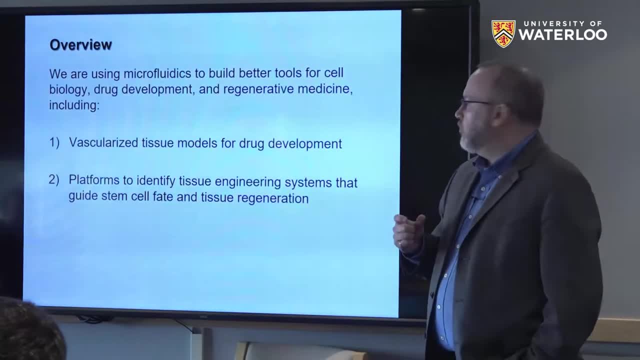 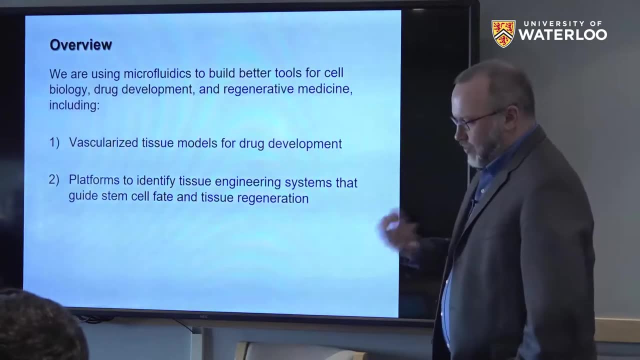 for drug development purposes, and then second platforms that we've been engineering to help understand how stem cells respond to stent. So there is a couple ways we can do that, but first we want to talk about them as a respond to their environment and and result in tissue regeneration In both of 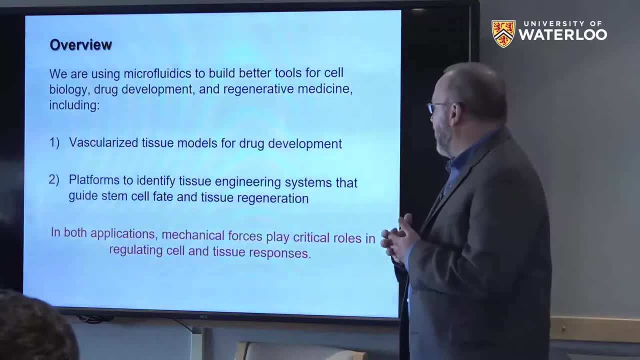 these applications. our focus is really on the fact that mechanical forces play critical roles in regulating cell and tissue properties in the body and in our efforts are kind of our niche in this area is to recapitulate those forces on these microfluidic platforms. So I'll first talk about our work on 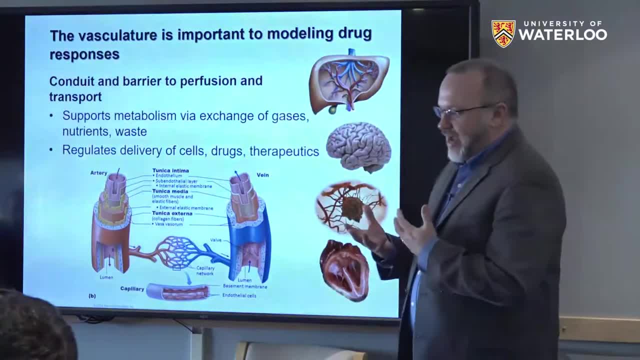 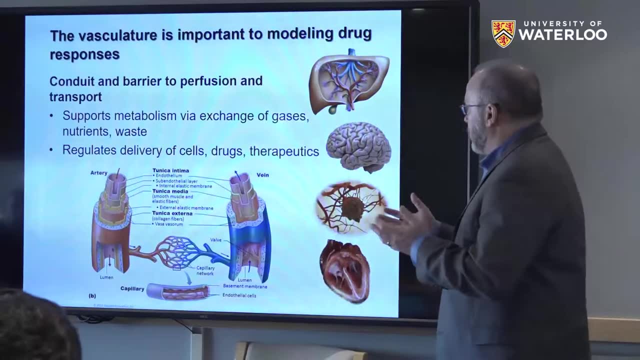 vascularized tissue modeling and so, as you're probably aware, the vasculature is important to model drug responses. First of all, the vasculature is the conduit for the drugs are carried through and it's a barrier to perfusion or transport from the blood to the surrounding tissues. So if you think of tissues or 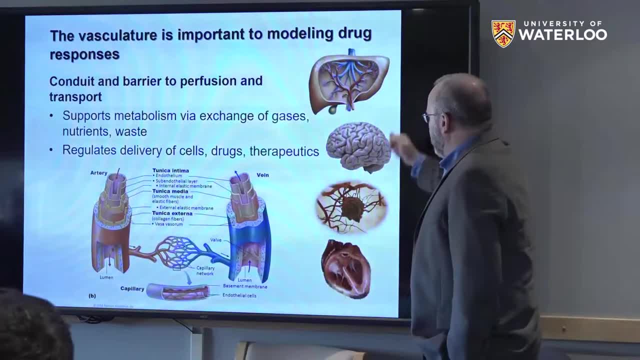 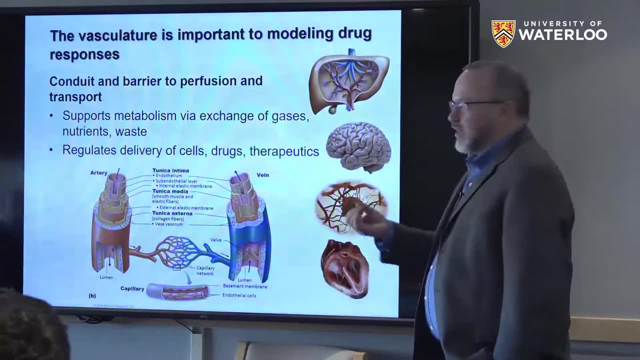 organs like the liver, the brain and the blood-brain barrier, cancer and tumors, and in the heart and other cardiovascular tissues. blood is carries the nutrients and gases to the tissue. waste is carried away through the blood and all those factors, of course, regulate. 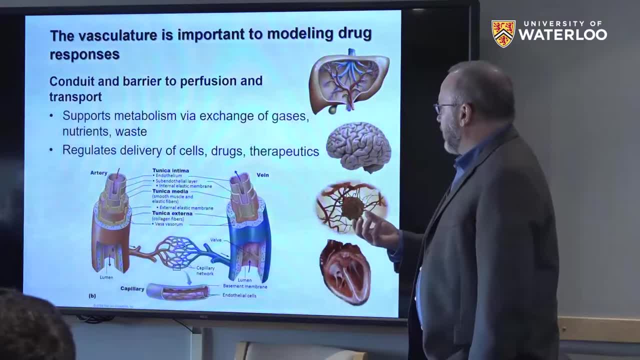 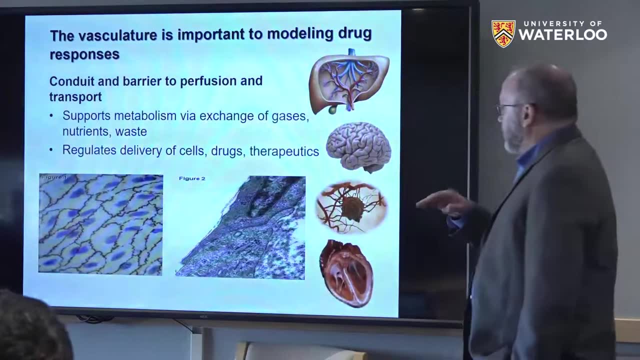 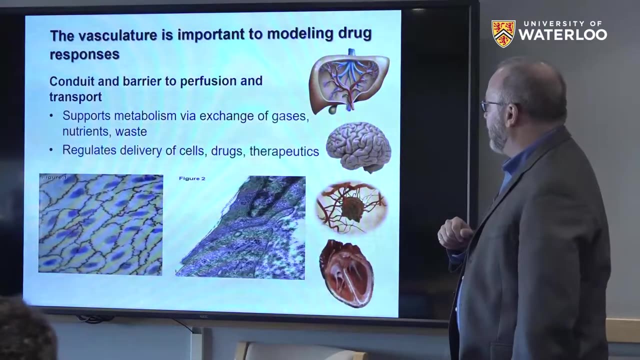 the blood Function, and then the vasculature also regulates delivery of cells, drugs and therapeutics. In addition, the, the vasculature in the endothelium in particular, provides a barrier, is a barrier that regulates how things get across the across the blood vessel wall. So this is a picture of endothelial 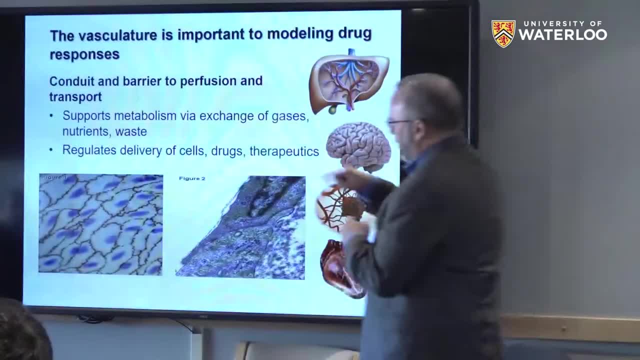 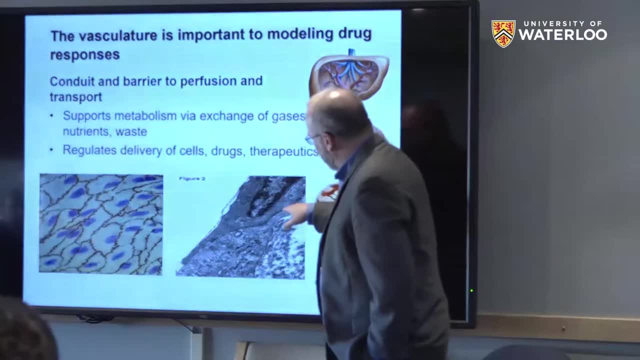 cells. So I have a top-down view and you can see the silver nitrate staining that shows the membrane between the cells and they're really in tight contact and this is a scanning electromyocytes. This is a micrograph that shows it in cross-section and you can see this interface here the two cells are. 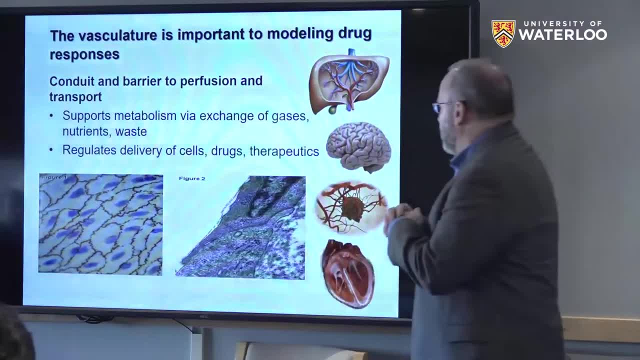 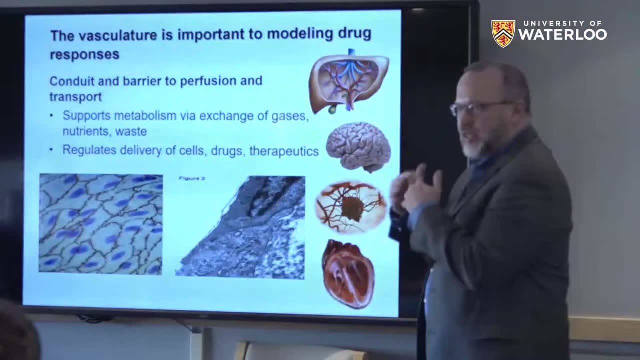 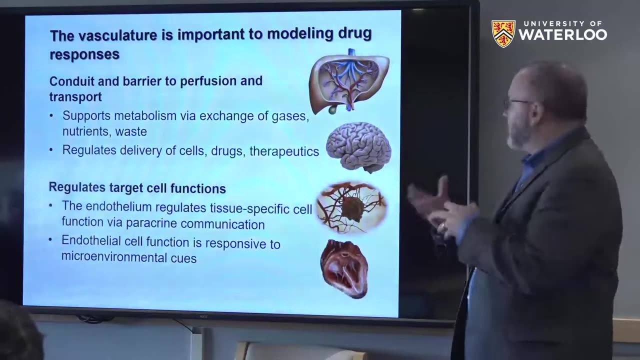 actually physically overlapping and have this tight junction, And so this is the barrier that regulates what gets from the blood into the tissue and vice versa, and recapitulating that in these devices we think is important. The endothelium also regulates the functions of the cells in our target tissues, or 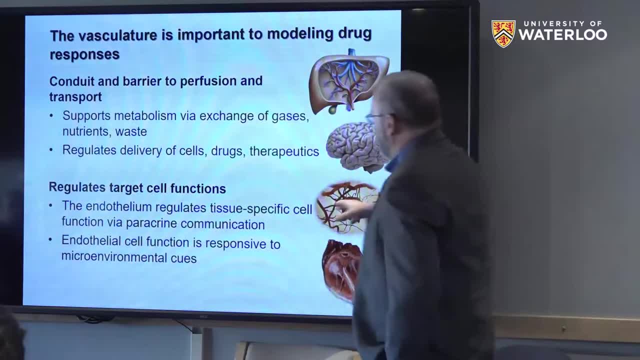 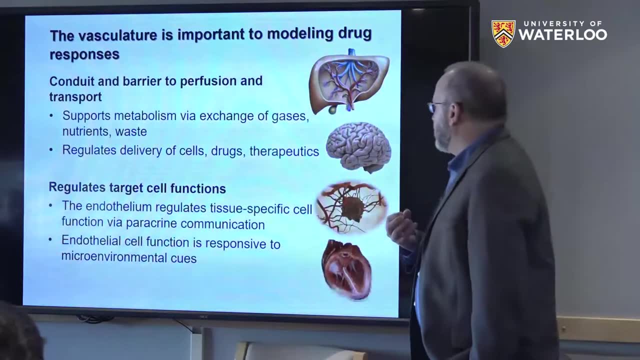 in the tissues that we're interested in, And so the endothelium can secrete molecules that act in a paracrine manner, or they can molecules that are secreted and go to act on other cells in the system. They can regulate the function of those cells. 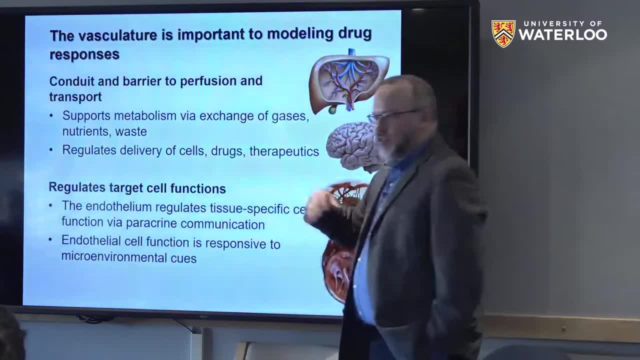 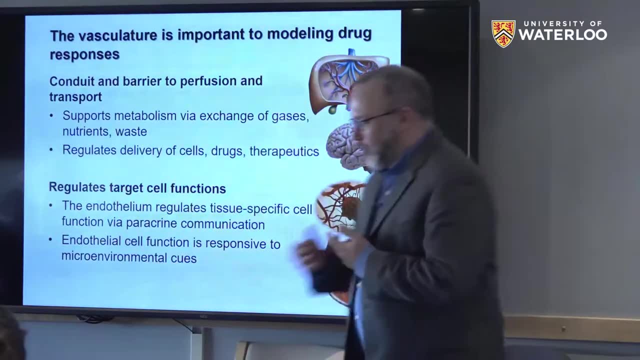 and the endothelium itself is also responsive to its cues in its micro environment. So the signals that the endothelium produces are also regulated by what's going on in the tissue And one of the important signals that the endothelium sees these cells that line the blood vessels are the physical. 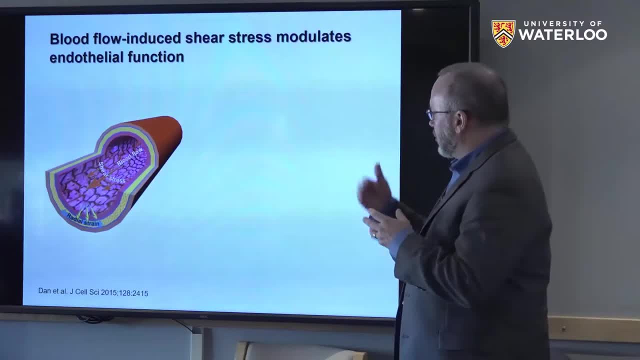 forces So as blood flows through a blood vessel, it exerts shear, stress or drag on the endothelium, It causes the blood vessels to strain epithelially and circumferentially, and all these forces are felt by the endothelial cells and the cells then respond accordingly. So for example, the adhesion. 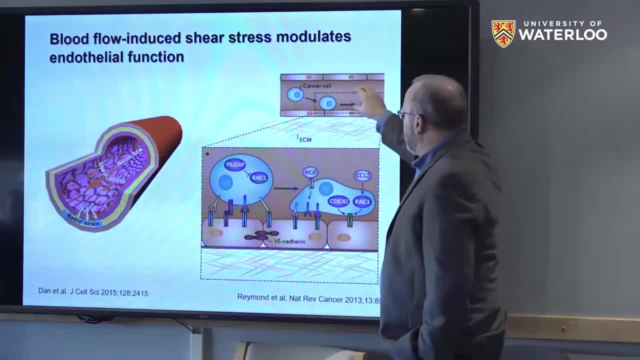 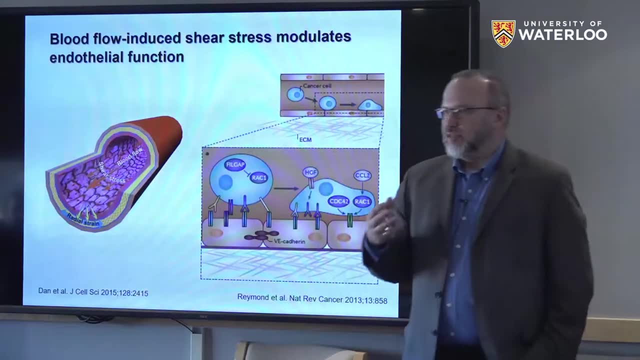 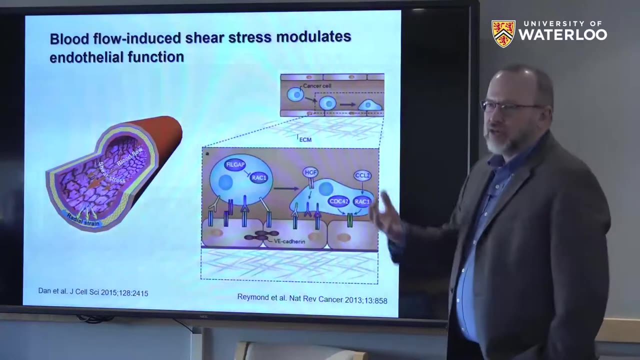 of circulating cancer cells or immune cells in the blood vessel and their ability to adhere to the endothelium and eventually crawl out. all that's influenced by shear stress. The endothelium produces receptors under shear stress that when they're sheared they wouldn't be. 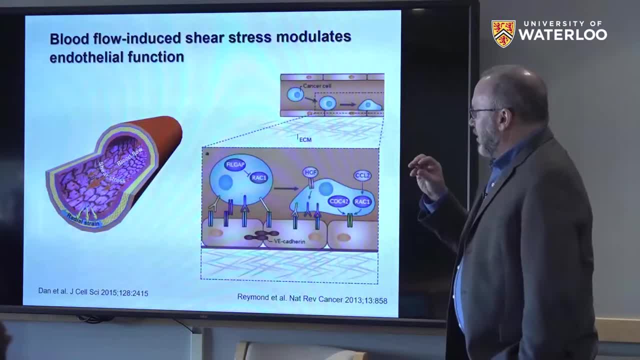 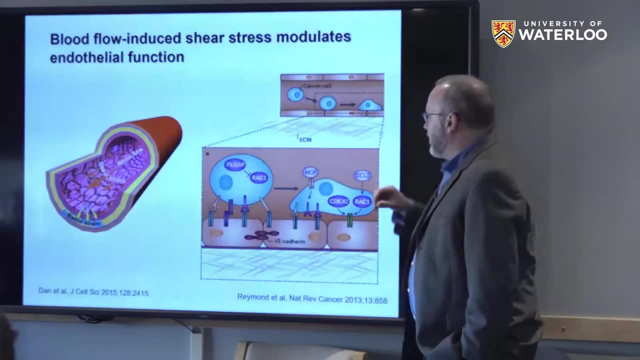 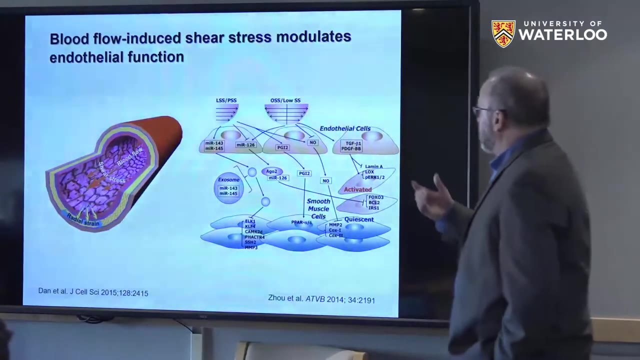 there if they weren't sheared And so recapitulating the mechanical environment. the shear environment is important if you really want to study the in vivo or physiological mechanisms by which cells can adhere and leave in cancer and in immune responses. Additionally, the type of flow that the cell sees, whether it's laminar shear, 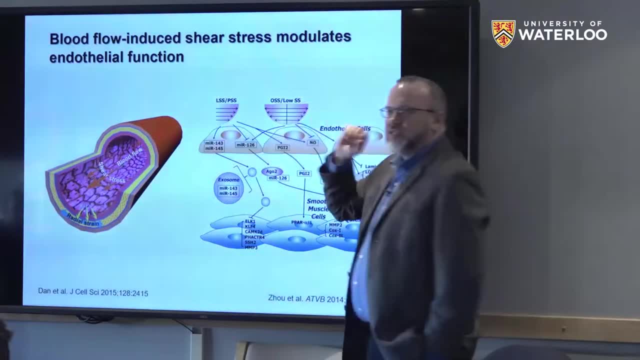 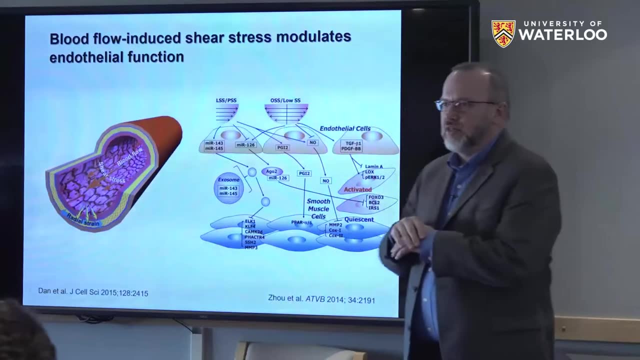 stress, or pulsatile in one direction versus an oscillatory type shear stress. this is going to influence different signaling pathways or turn on different signaling pathways in the endothelium, causing them to make different factors that are then going to influence the cells within the tissue. So, for example, in 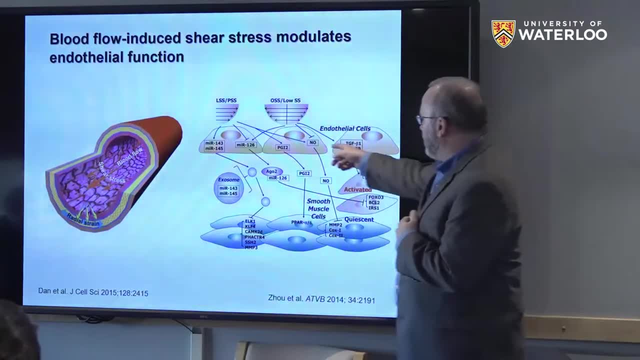 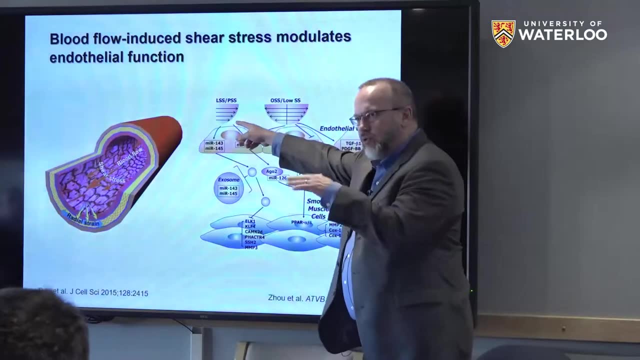 blood vessels, where you have smooth muscle cells, the production of something like nitric oxide, which causes the cells to become quiescent, is regulated differently, whether you're in high flow, laminar shear stress or oscillatory shear stress. So again, the fluid environment, the mechanical, hemodynamic. 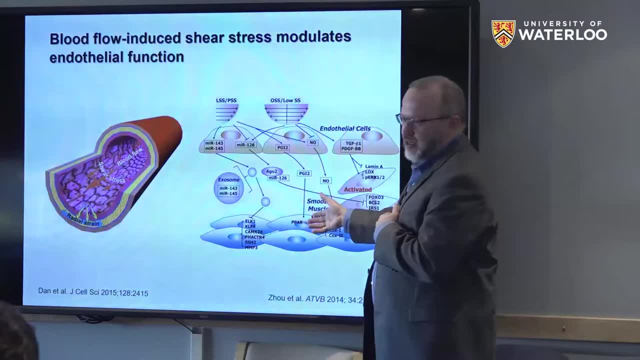 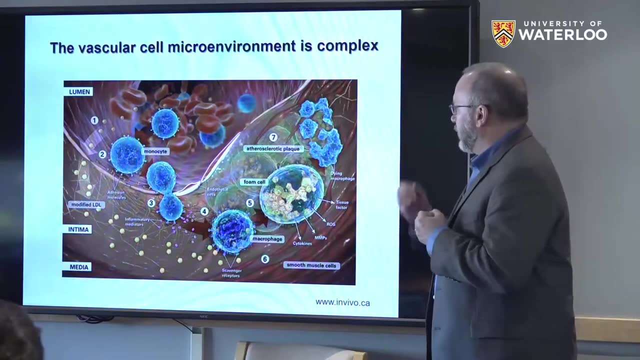 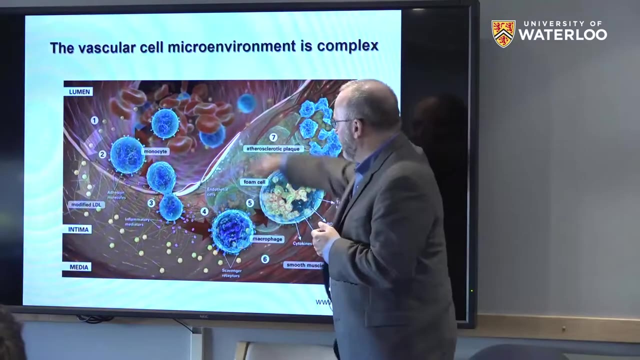 environment influences how these cells signal to the underlying cells, And so the vascular environment, therefore, is obviously complex, right, Lots going on. You have multiple cell types, you have flow forces exerted by flow, you have a 3D structure and you have this barrier And, right now, a lot of 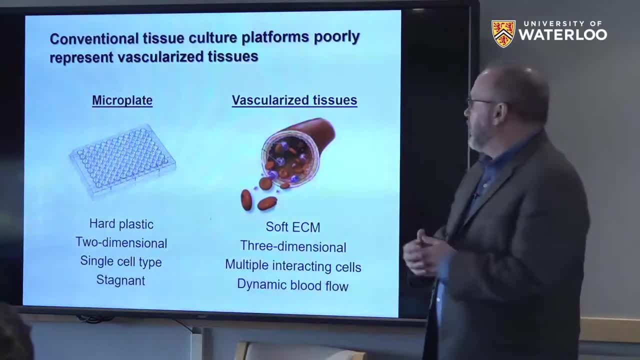 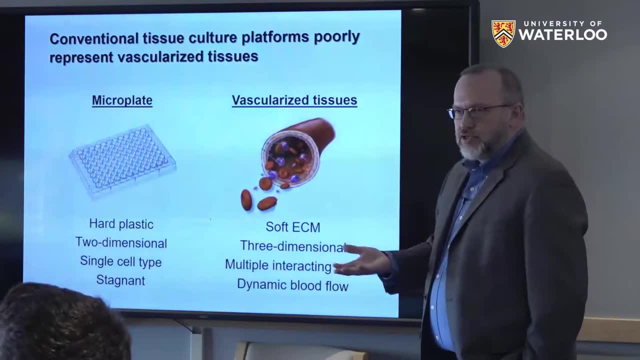 biology, as you're aware, is done in dishes right, So on the left is a typical microplate. it's a hard plastic, it's two-dimensional, often is only a single cell type and clearly doesn't have the blood flow. it's a stagnant. 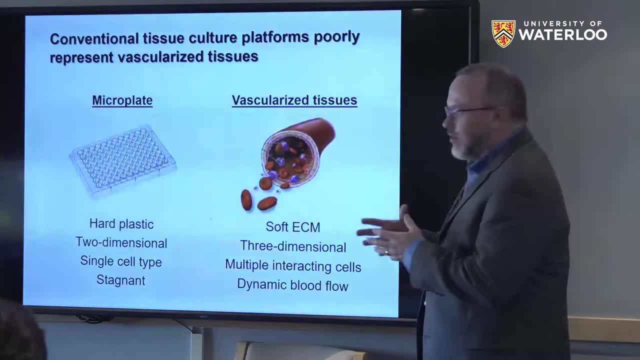 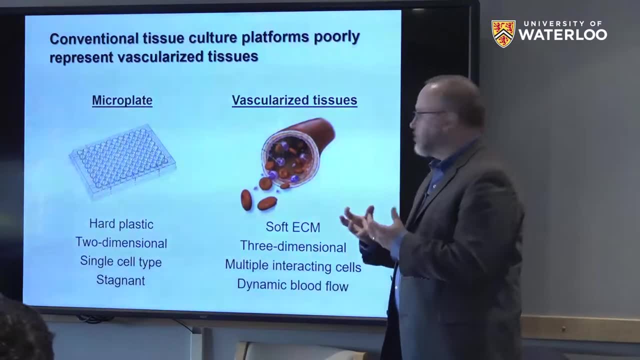 environment, And so this really doesn't represent very well what happens in the body in a real vascularized tissue. Vascularized tissues are soft, they have an extracellular matrix, they're three-dimensional, they have multiple cell types that interact in these complex manners and they're. 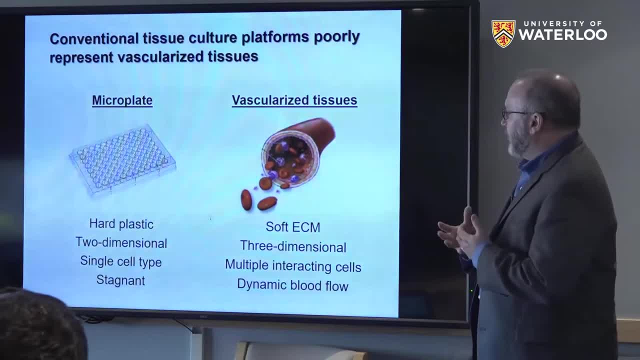 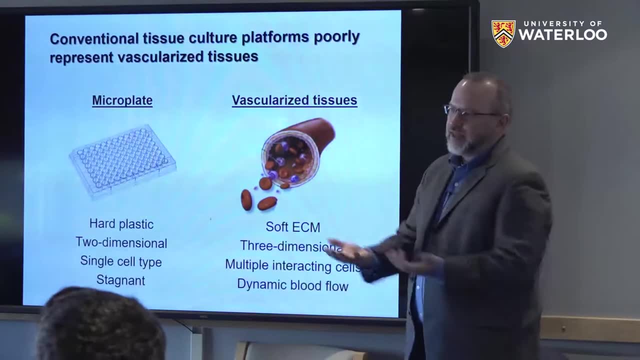 subjected to dynamic blood flow, And so there's been a lot of effort and interest in. can we model or recapitulate what happens in a vascularized tissue in the body? can we recapitulate that in the lab? Because if we're interested in 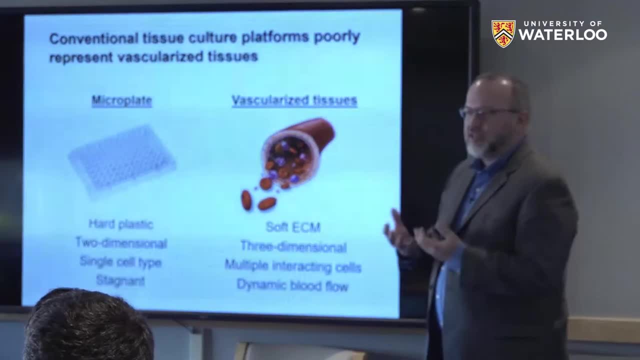 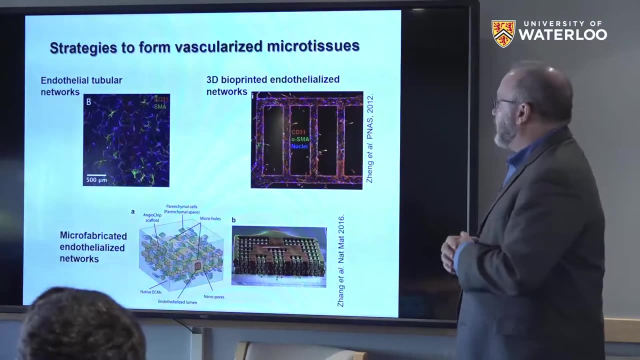 studying drugs and seeing how they were shown in the body, presumably a lot of these factors are going to be very important. So we're going to do a lot of research to see if these factors are going to be important for drug responses. And so there's lots of strategies to engineer or form vascularized 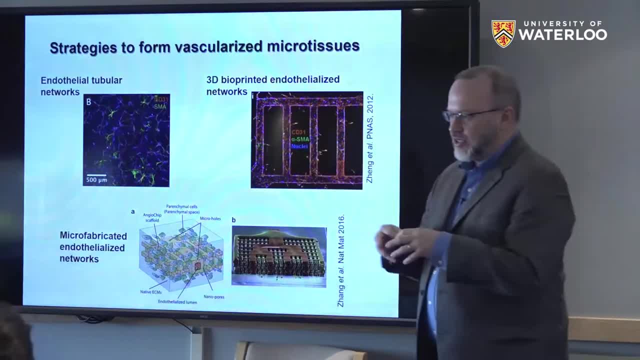 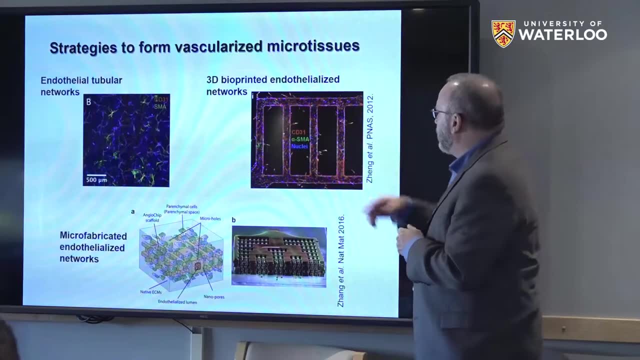 microtissues. You can just sort of stick endothelial cells in a structure and they'll actually assemble to form tubular networks. You can bioprint 3D bioprint structures. this is from Milica Radicek's lab at the University of 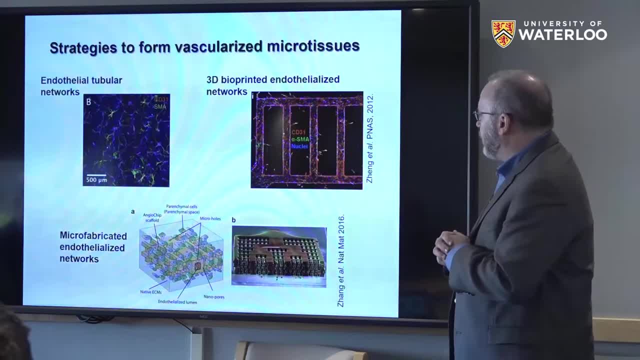 Toronto you can come up with these complex microfabricated networks, and all these approaches do recapitulate aspects of the vasculature and are a effective in many ways and for different applications. The direction we've gone is to try and actually go a little more simple than these, I think. 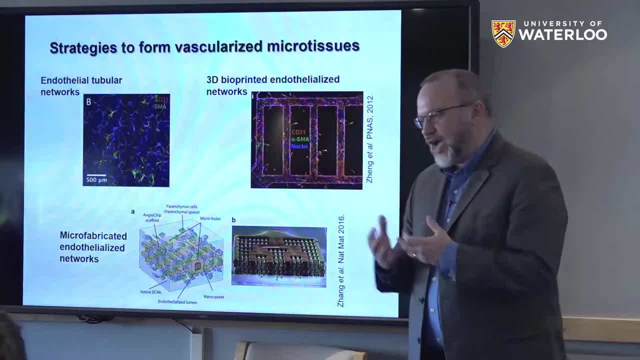 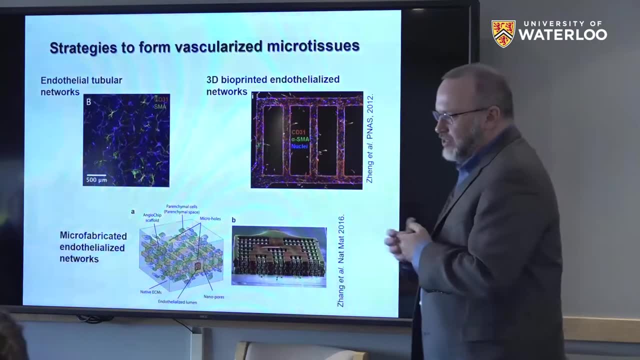 these are complex and the complexity sometimes presents challenges to actually use them to do fundamental biology and drug discovery. And so we've taken a little bit of a step back and asked: you know, can we use microfluidics to make little more simpler systems that still capture key components of that? 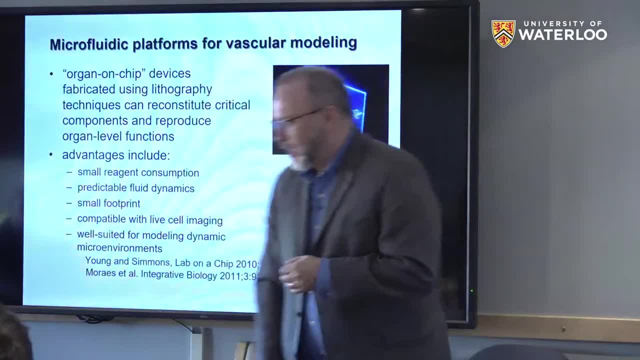 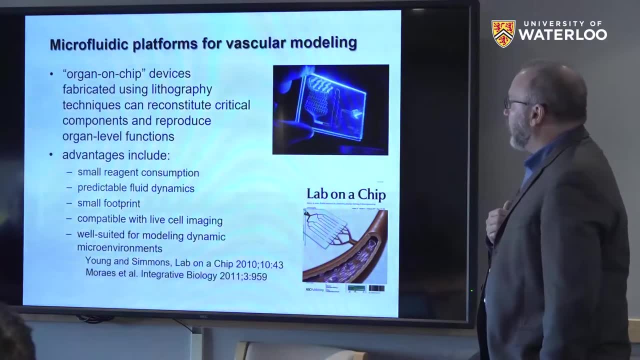 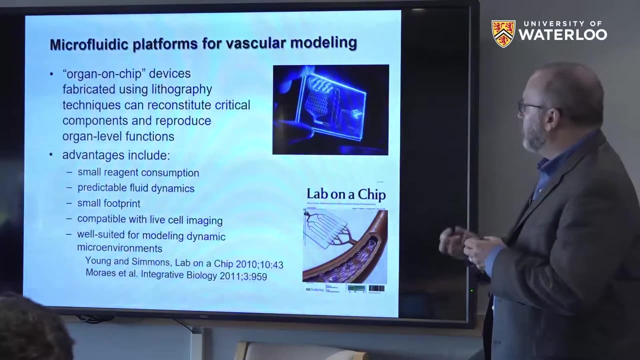 vascularized tissue environment, And so microfluidic platforms are well suited for vascular modeling. These are sometimes called organ on a chip devices. They're fabricated using lithography techniques, and the idea again is: can you recapitulate critical components and reproduce organ level functions on a chip or in a dish that mimics what's? 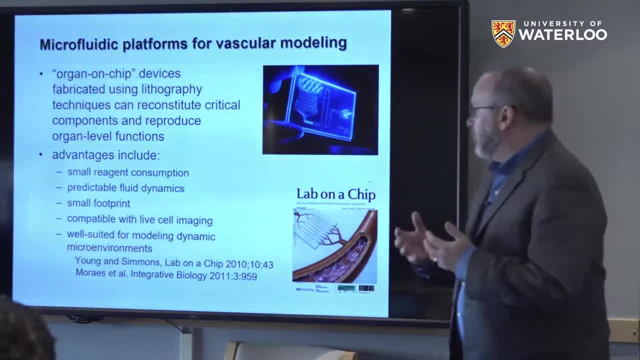 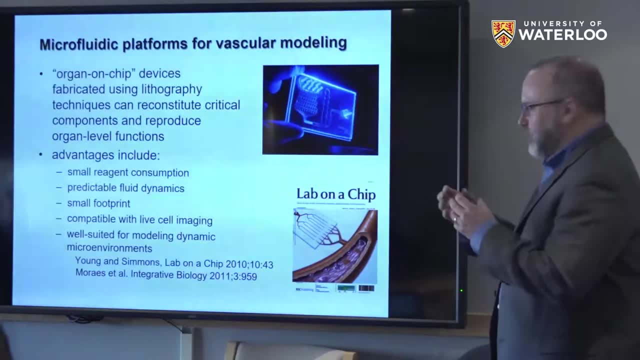 going on in the body. And the advantages of microfluidics, you may be aware, are small reagent consumption, because everything's miniaturized. the fluid dynamics is very important. They can be small footprint and you can imagine them doing many in parallel. They're compatible with live cell imaging, so for certain, 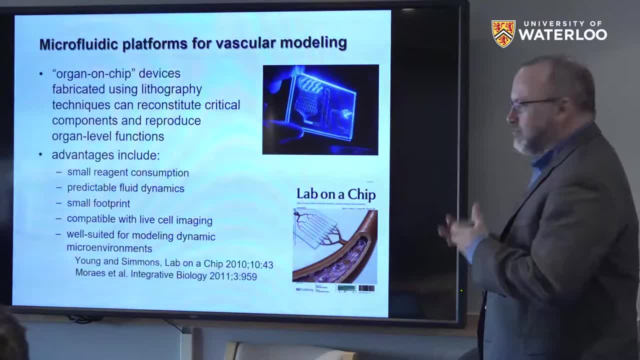 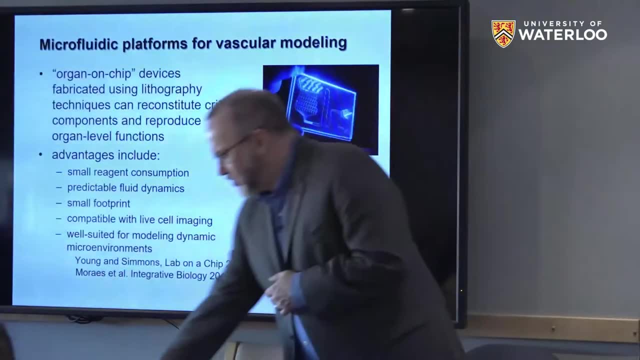 applications. that's really useful- And for modeling the dynamics and the mechanics that occur in micro environments. they're often well suited and we have a couple of reviews on that. So this is the platform, the general idea of the platform that we've been using for several years now. Again, it's fairly 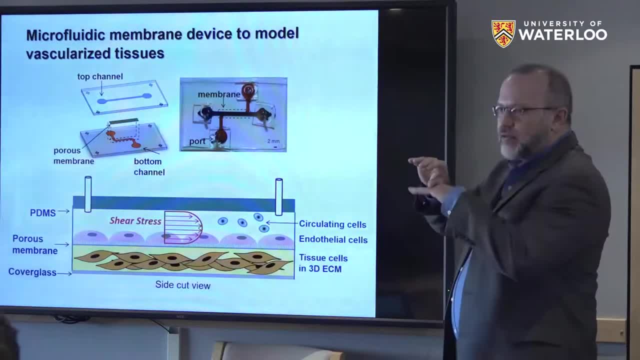 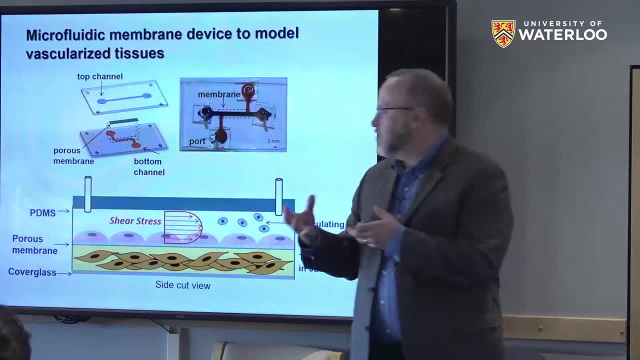 straightforward. It's just two channels that are stacked on top of one another, separated by a porous membrane, And so these channels are made out of a polymer called polydimethylsiloxane or PDMS, and then the porous membrane is a could be a variety of polymers We use. 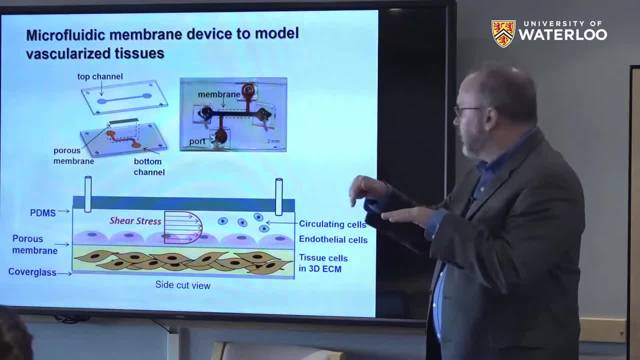 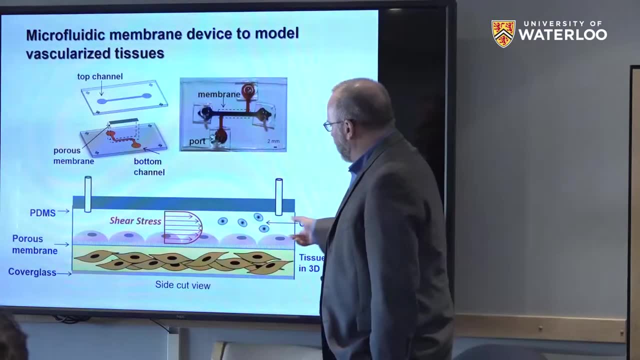 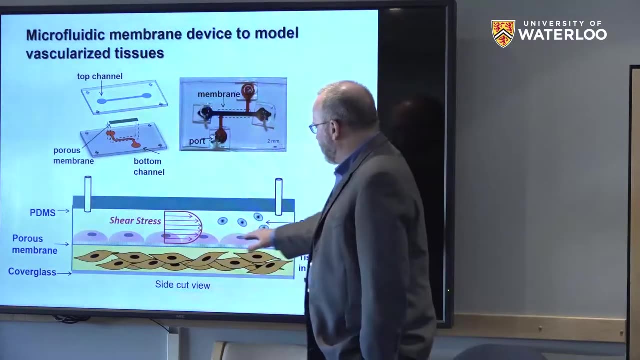 PET or polycarbonate, and then it has pores in it, and the pores allow transport between the top channel and the bottom channel. And so our idea is, by stacking these we can create a blood vessel channel on the top and a tissue channel on the bottom, And we line the membrane with endothelial cells. the pink: 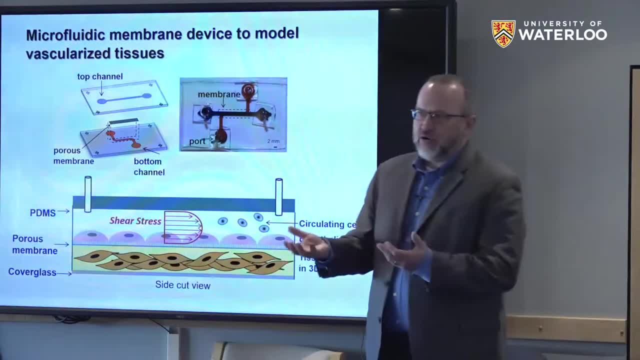 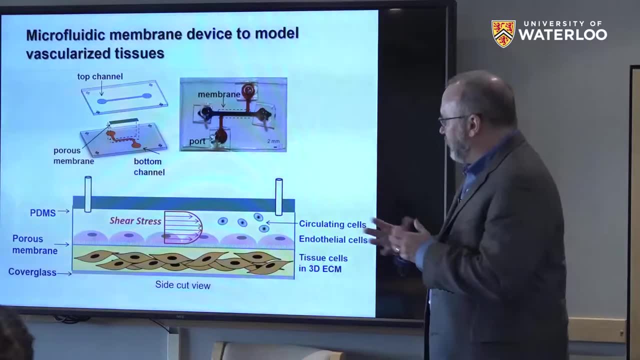 cells here And in the bottom channel. we can either leave it empty or we can fill it with a 3D biomaterial embedded with cells of interest, the tissue cells of interest, And so we see this as sort of a platform technology type approach where you could 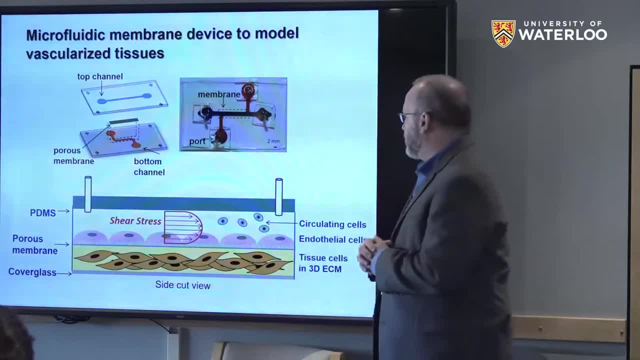 stick in your tissue of interest, depending on what you're trying to model or study, And by pumping fluid through the culture media, through the top channel, we can exert a physiological shear stress on the endothelium, We can put through circulating cells, you can put through drugs and you can now. 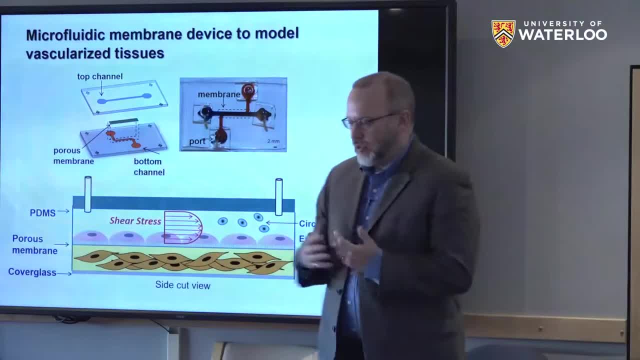 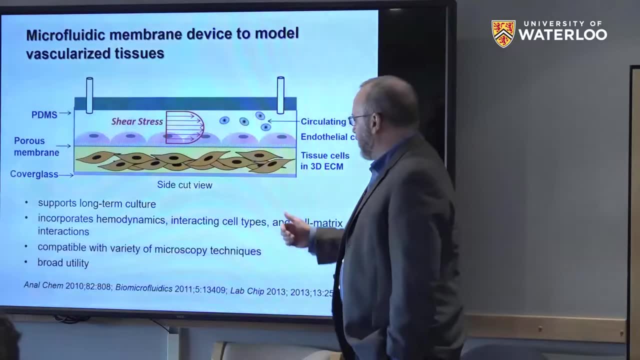 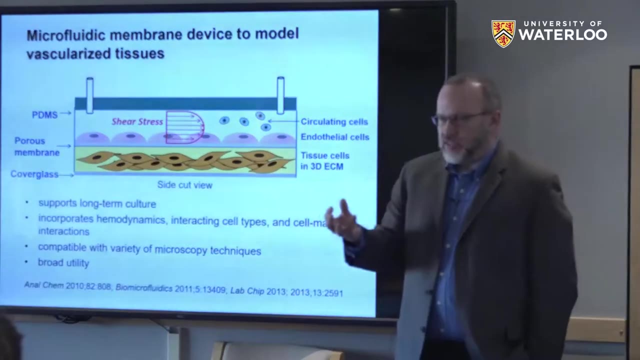 recapitulate many aspects of what we see in the actual body. We can grow cells for long-term in this system. It incorporates the hemodynamics, incorporates multiple interacting cell types and incorporates cell matrix- interactions that we know exist in vivo but are not. 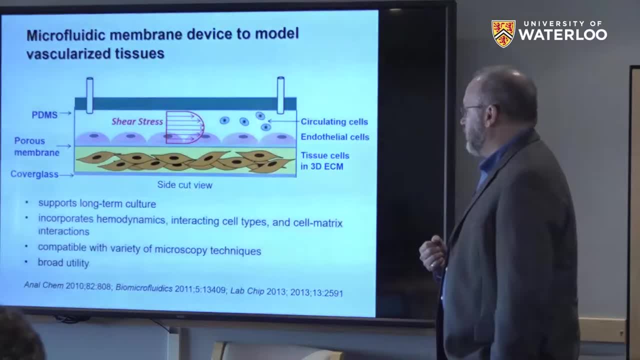 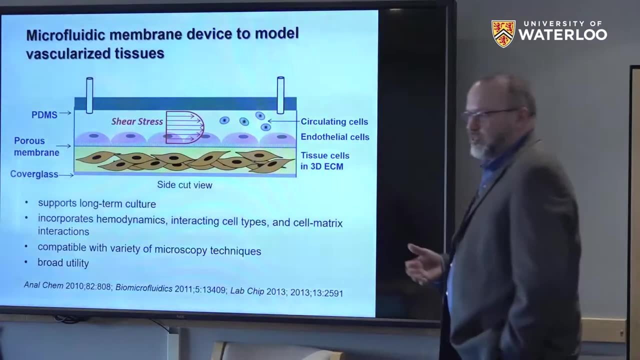 well represented in traditional petri dish type setups. It can be set up to be compatible with a variety of microscopy techniques, and we think it has broad utility for a wide range of applications, And so I'll show you some of the applications that we've worked on and kind of the direction we're heading. 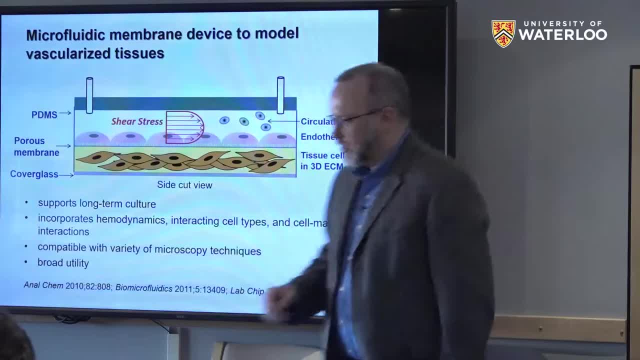 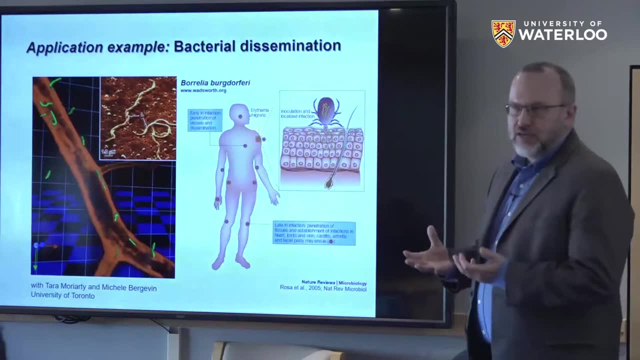 with this, but it's all based on this kind of basic concept. So the first application I'll tell you about is our work and interest in using this to study how bacteria leave the blood vessel to get into target tissues where they can cause disease. 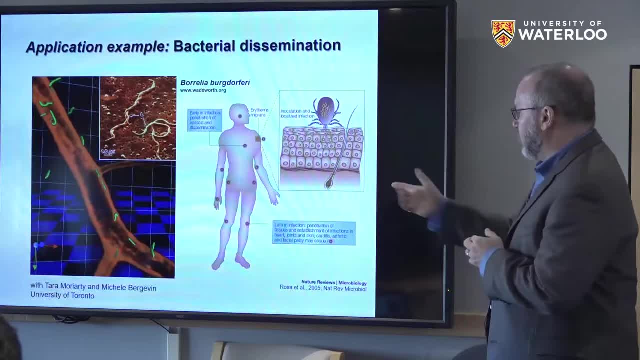 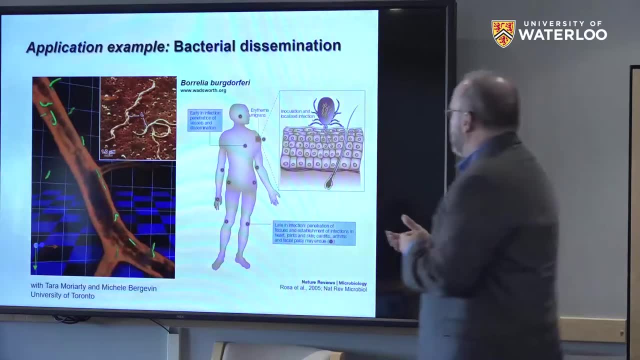 And this is a collaboration with Tara Moriarty at the University of Toronto, and we co-supervised Michelle Bergevin, a master's student, and Tara studies the bacterium that causes Lyme disease, And so the idea with Lyme disease is: you have a tick, you're walking off in the woods somewhere. a tick bites you. it releases these bacteria into your, they get into your bloodstream and then the bacteria swim through the bloodstream and eventually hit target organs and tissues. where they leave the bloodstream and they're not causing any harm within the blood. but once they leave, they then get into the heart, the joints, the skin and so on where they cause pain. And so this is. you know you hear more and more about Lyme disease is more and more of a problem. Antibiotics can be effective, but what would be really effective is if you could actually prevent the bacteria from leaving the blood vessels in the first place and allow the body's immune system to get rid of them. 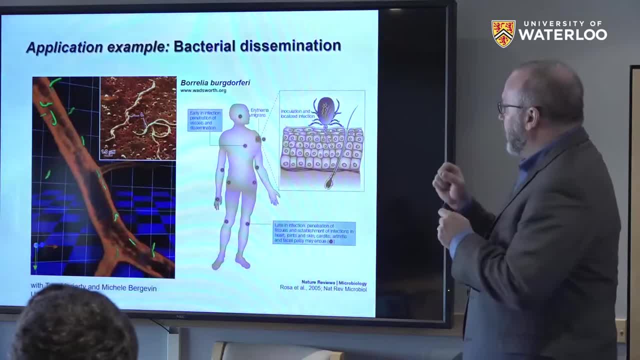 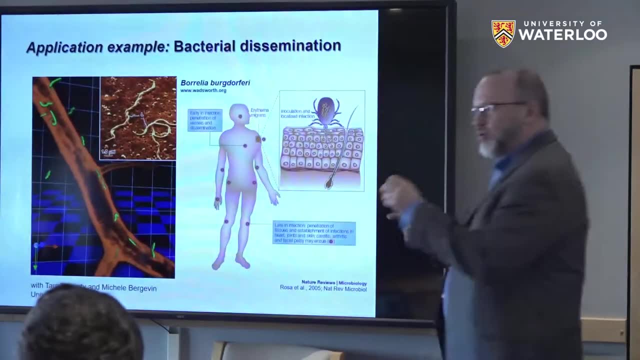 And so Tara really wants to understand: how does a bacterium adhere to the endothelium and then get out of the endothelium? And the bacterium look like these: they're about 30 microns long, only 0.2 microns in diameter, and the way she studies them or had studied them, is she studied them in mice and doing 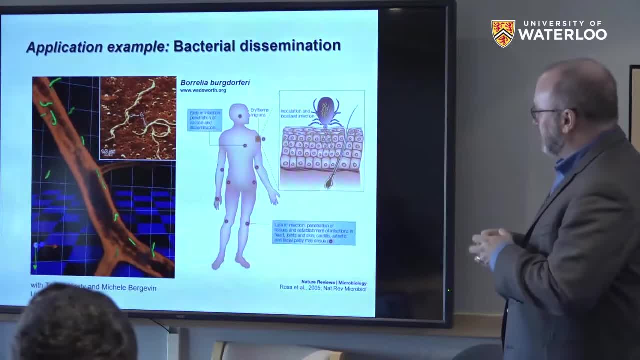 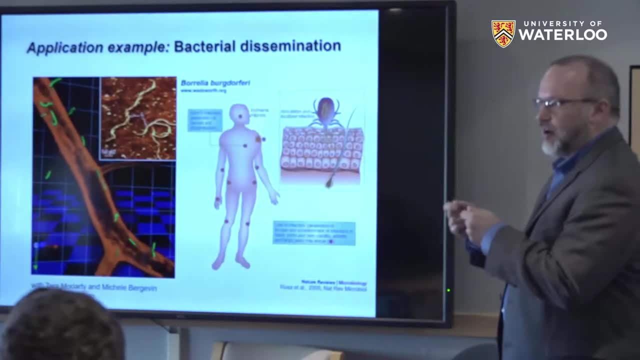 intravital imaging in mice. She would inject the mice with tons of bacteria, like way more than would ever be reasonable, and then watch a blood vessel And hope that she got a bacterium leaving that blood vessel during that experiment And it's kind of like searching for a needle in the haystack. The immune system gets rid of a lot of bacteria. 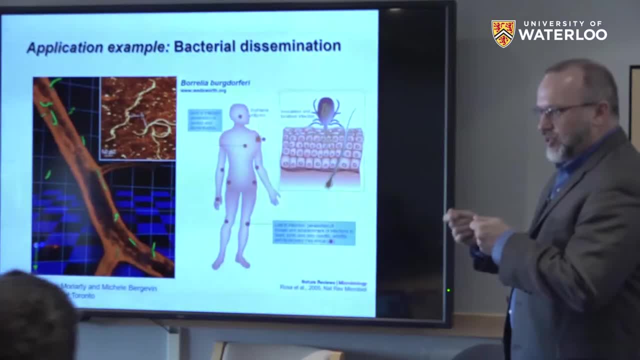 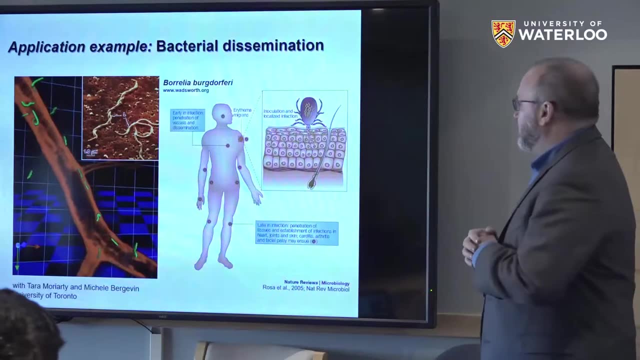 they inject. and then you have to hope that the blood vessel you're looking at does have a bacterium come by it and that bacterium does choose to leave the blood vessel at that time point, And so she would go through dozens of mice to get you know, just a very small amount of data. 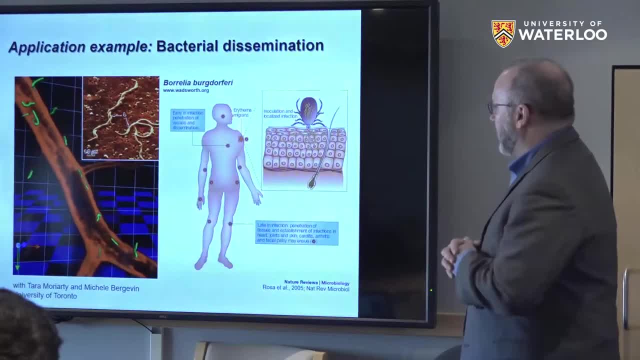 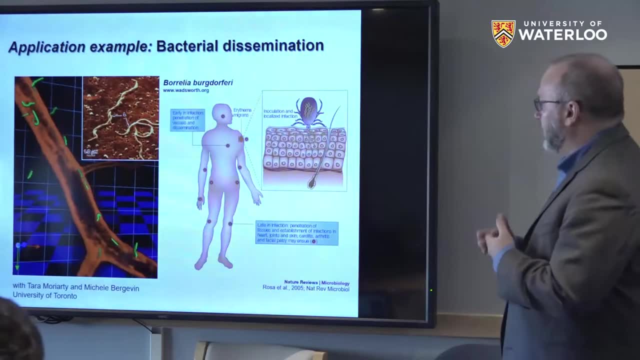 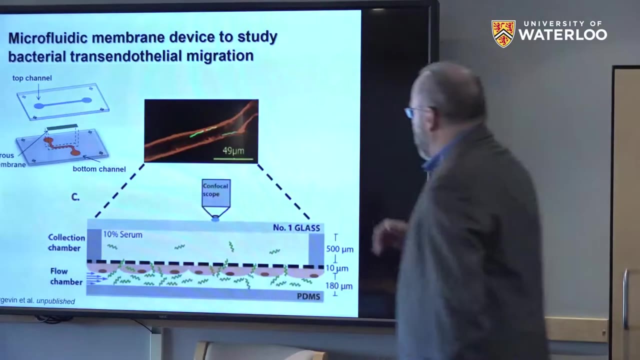 So highly inefficient, not ethical, all sorts of problems with it, And so she was really interested in: can she study this in vitro? Can she use a microfluidic model to recapture, to capture this transport process? And so this is where we've been applying our two-layer channel chamber system. 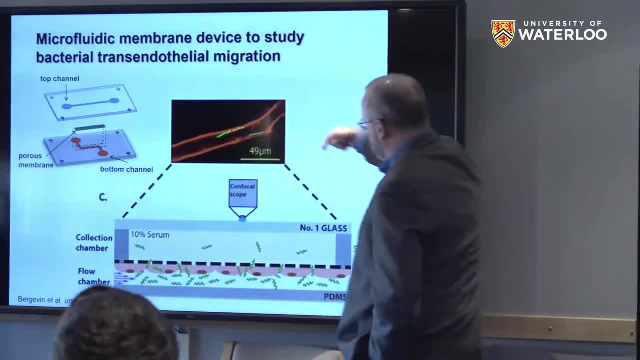 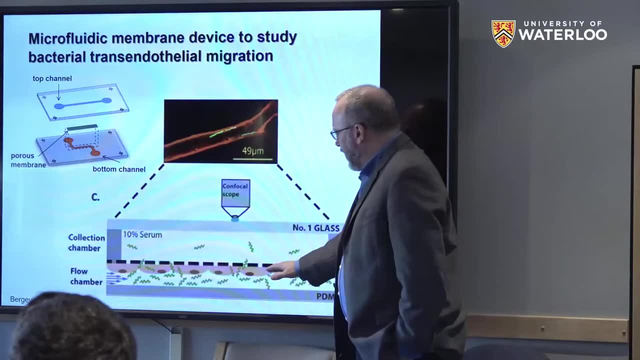 So in this case we flipped it upside down, because her microscope is an upright microscope, so she visualizes from this direction. But again, here's the blood vessel chamber, the endothelium lining, that, and then our collection chamber, we call it, And this is where the bacterium are injected into the bloodstream and then they migrate. 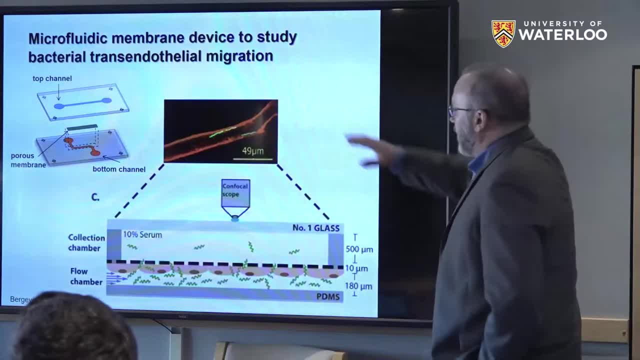 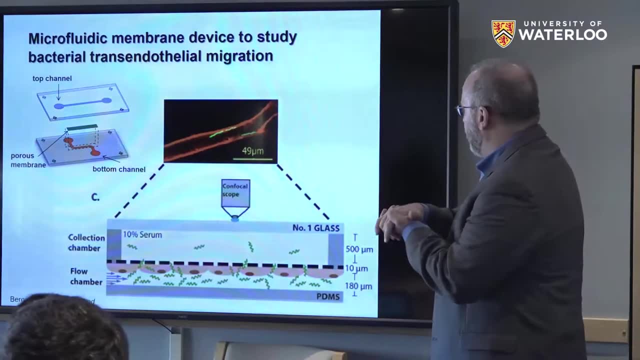 through the endothelium into the collection chamber And the setup is very similar to what I described before. It's two PDMS layers with a glass bottom and then a porous membrane on the top- Or sorry, glass top in this case, because we've inverted it. 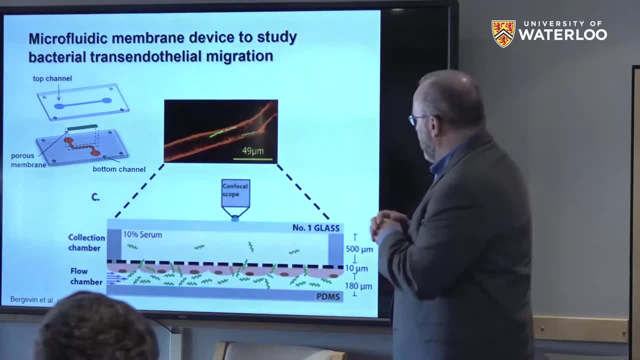 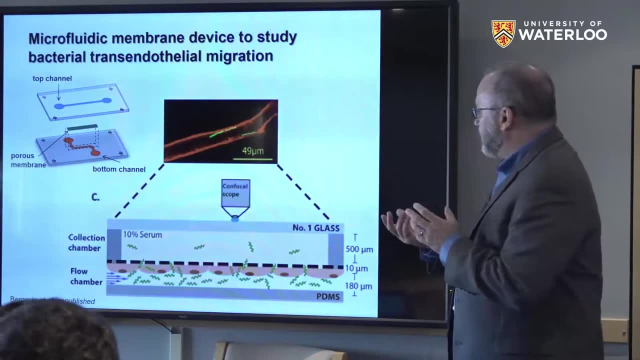 And the dimensions approximate what we would see in vivo. The bacterium are engineered to fluoresce green so we can track them in real time as they go through these channels, And then we can visualize them using real-time confocal microscopy. visualize live cells swimming through the. 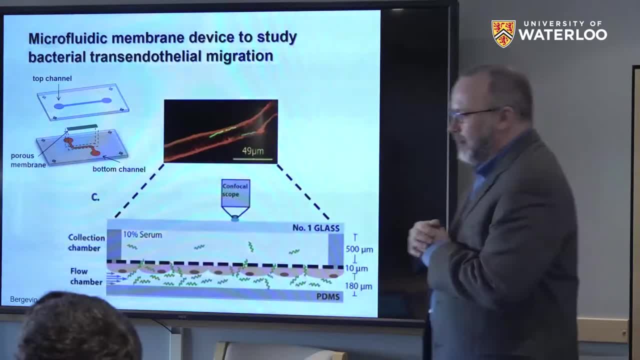 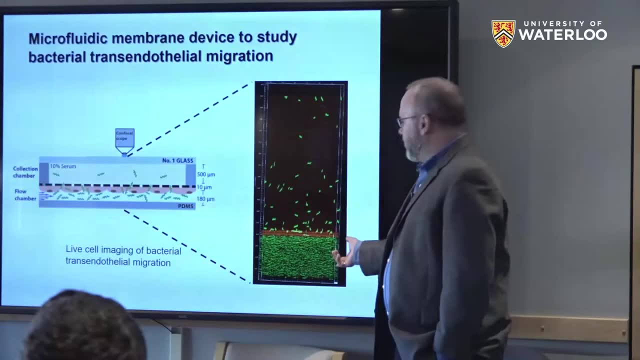 endothelium, squeezing through the endothelium into the collecting chamber, And so this is the sort of images we get. You can see the bottom chamber is very high density of bacteria that have been injected and then the endothelium is shown here in red on the membrane and you can see individual bacteria that have 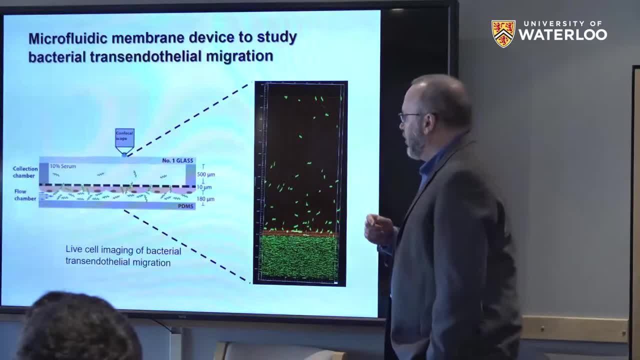 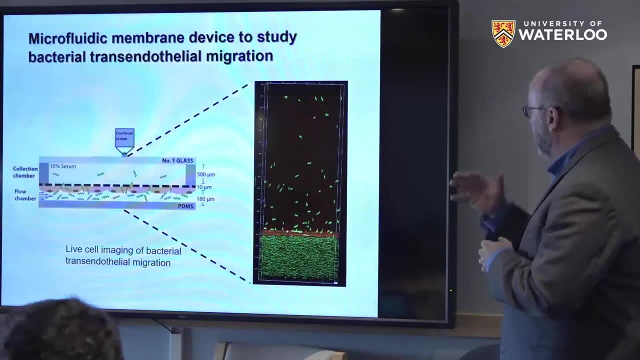 penetrated the endothelium, are now swimming into the collection chamber, And so Michelle is able to do this in using live cell imaging and scan very large volumes very rapidly and actually pick off then individual bacteria And then using image analysis approaches she can then actually 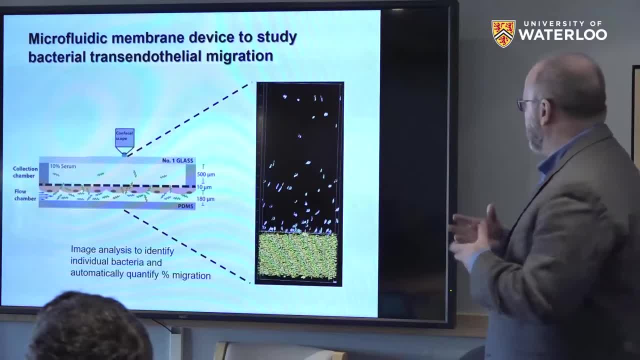 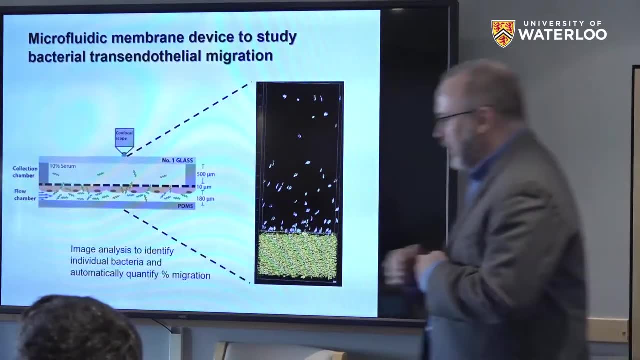 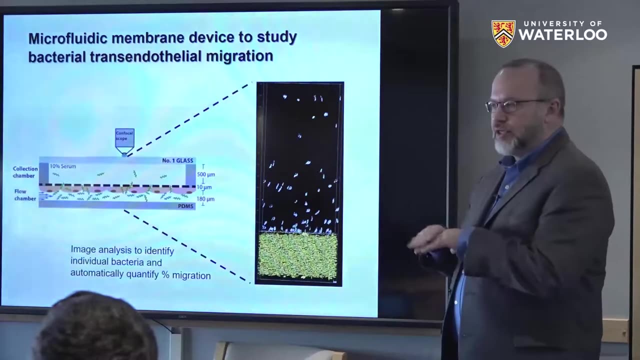 identify individual bacteria and quantify what fraction of the bacteria that have been injected have actually been able to migrate through, and look at the dynamics and the kinetics by which that occurs. And so this method turns out to be very sensitive, That what had been done in the past is all this had been done under static conditions in. 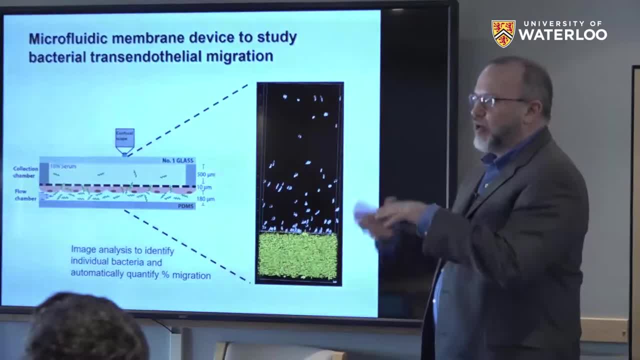 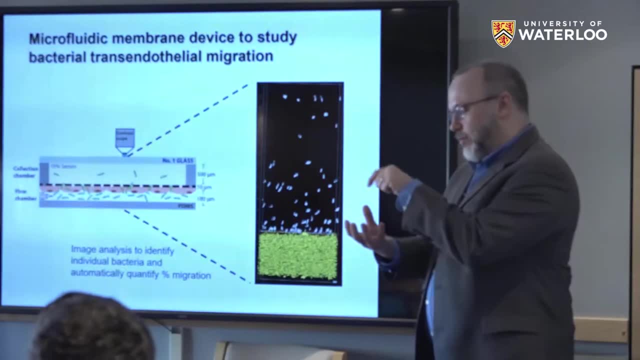 what are called trans-well devices. Trans-well devices are basically just a membrane that sits in a plastic dish and the bacteria were added on top And they were watched. how many would or not not watched? they would. they would swim through the endothelium. 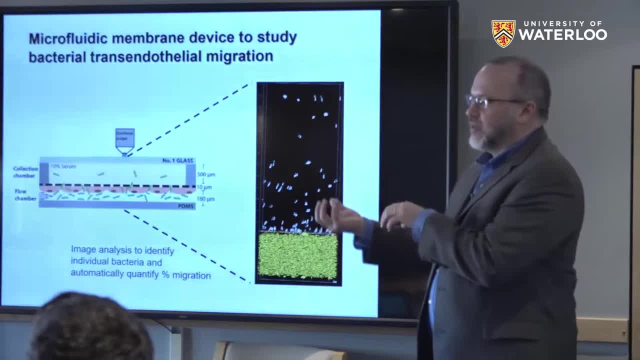 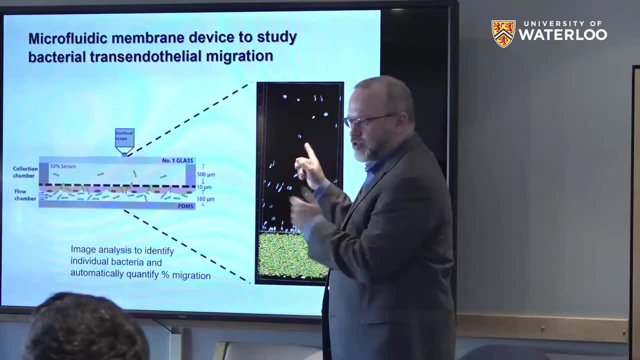 They would collect the collecting chamber and measure the fluorescence in a plate reader. With Michelle's system, because we two things: one, we can pick off individual bacterium, so I'll show you that gives us much more sensitivity. and then, second, she can do this all under flow, right. 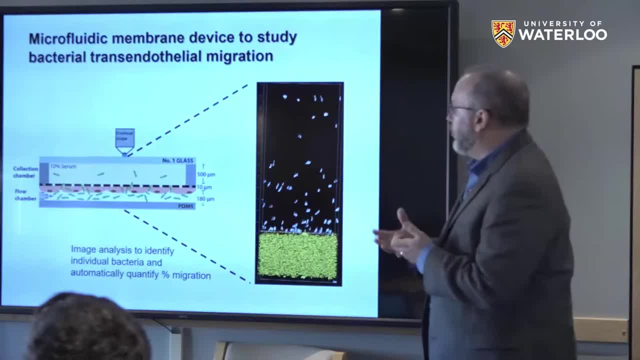 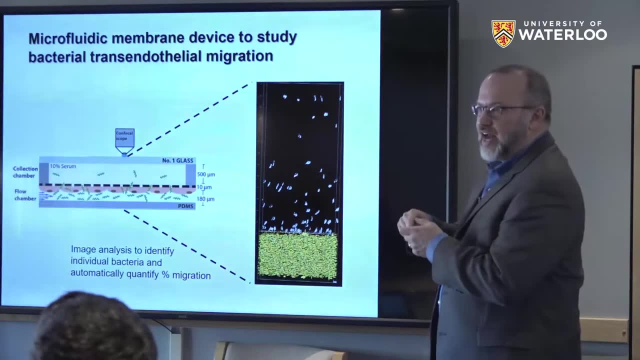 So now we can introduce the shear stress component, and Tara has shown that the adhesion of bacterium to the endothelium depends on shear stress. They adhere better under stress- Sheer conditions than they do under static. So this is a case where, if you don't model the shear stress, 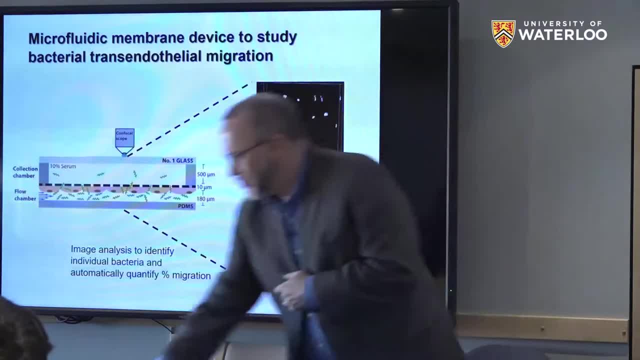 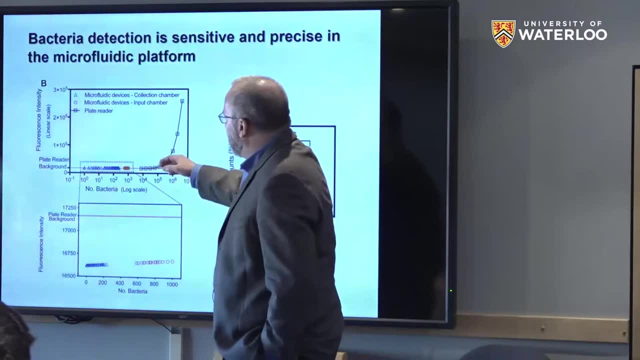 you're actually not capturing what's going on in the body, And so the sensitivity we can get it's shown here. so what's plotted here is the number of bacterium- It's a log scale- and then the fluorescence intensity, and this is for a plate reader. 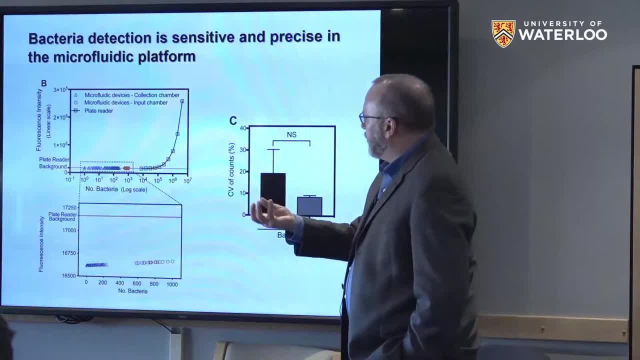 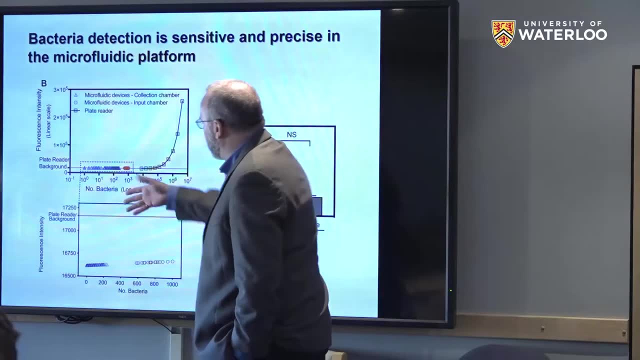 So a standard way that it would have been done. you put it into an instrument that measures your fluorescence intensity and you can see we've got some background level that we can't read below, and that's equivalent to about 10 to the fourth degree. 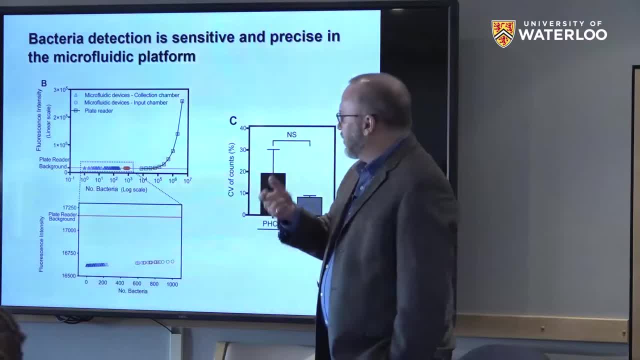 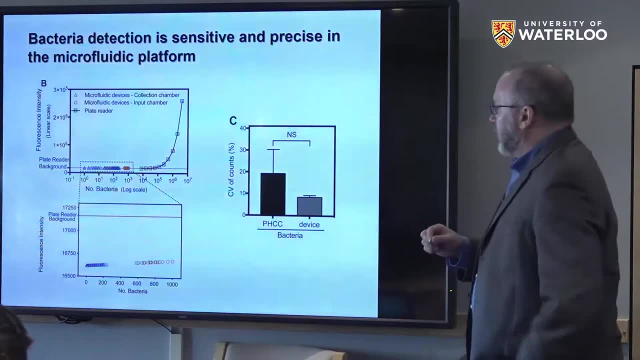 So we can actually measure that with bacteria. but when we start looking in the microfluidic device with the confocal microscope, we can get down all the way to individual bacteria. So we have much more sensitivity in terms of being able to track this and see. you know. 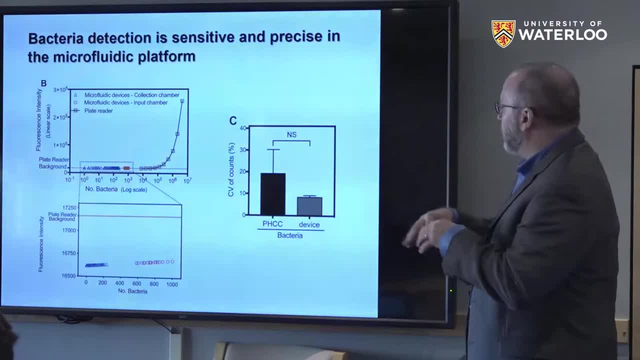 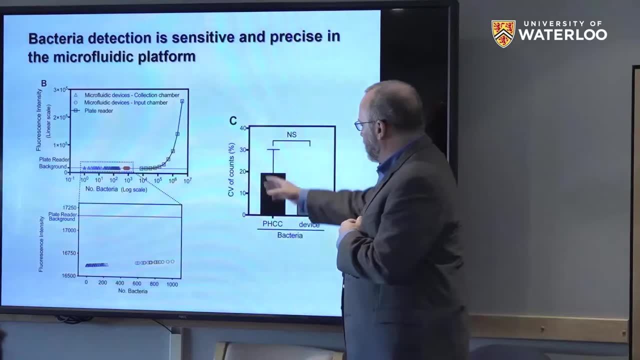 earlier on, when just a few bacteria are getting through the endothelium, we can actually pick that up. We also have more precise measurements. This is the traditional way that you count bacteria. You can see the coefficient of variation is about 20% or less than 10%, so the precision of our measurements is also better. 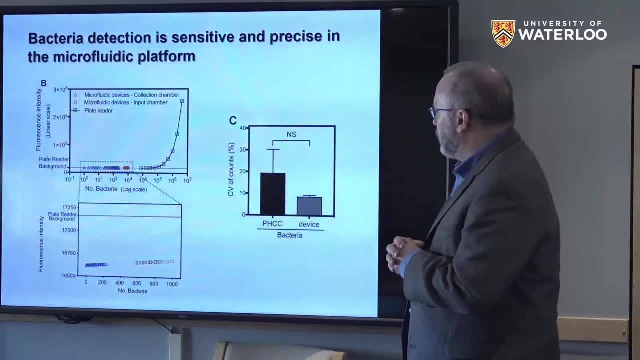 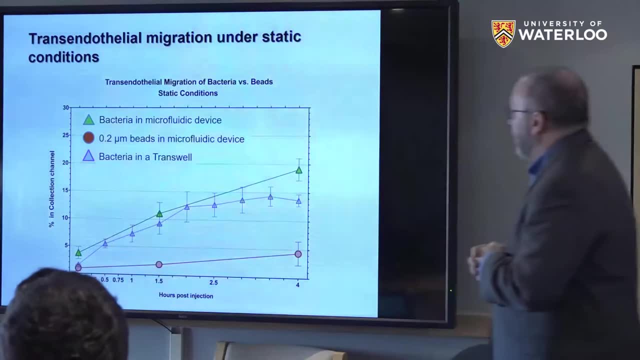 So just there, I think there's some advantage to doing it with this approach. But again, the big advantage, the big advance, I think, is the fact that we can do it under shear. So we compared how bacteria swam through the endothelium or migrated through the endothelium over time. 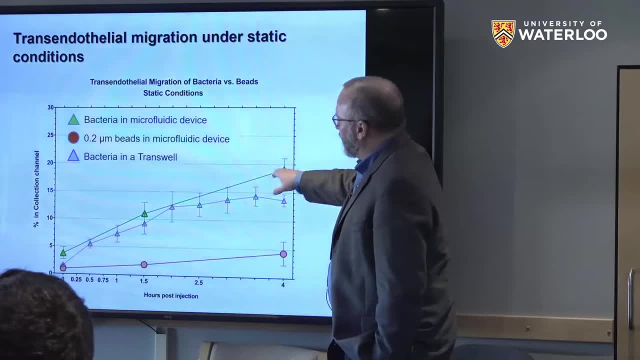 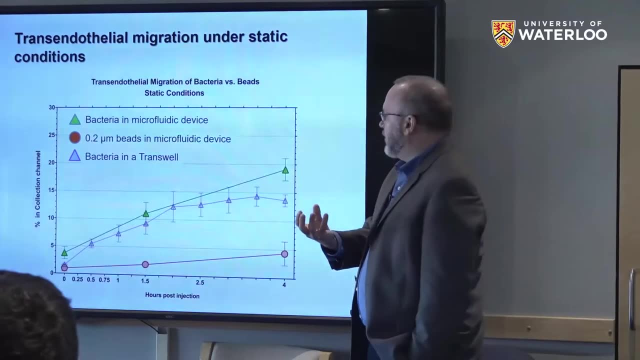 So the green bar shows the actual bacteria in the microfluidic device. You can see, by four hours under static conditions about 20% of the bacterium have been able to migrate through the endothelium. We compared that to the traditional. 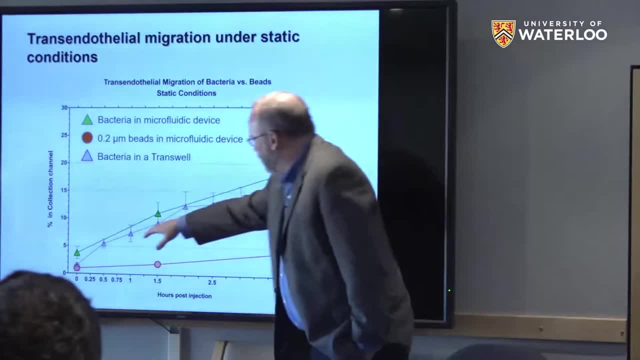 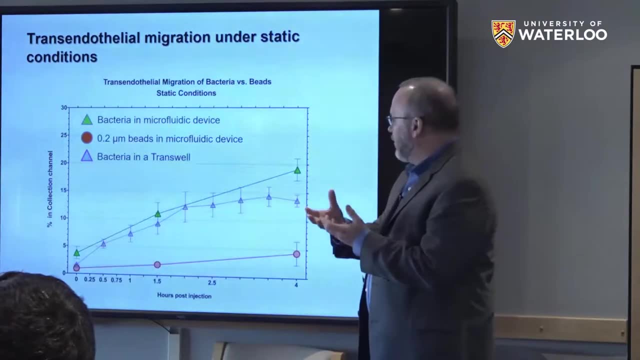 method, the transwell, because it was static And you can see the curve fits. very similar kind of deviates a little bit at the end, But through much of the time we see the same kinetics. So that was reassuring that we're not. our microfluidic device isn't really changing anything under static conditions. 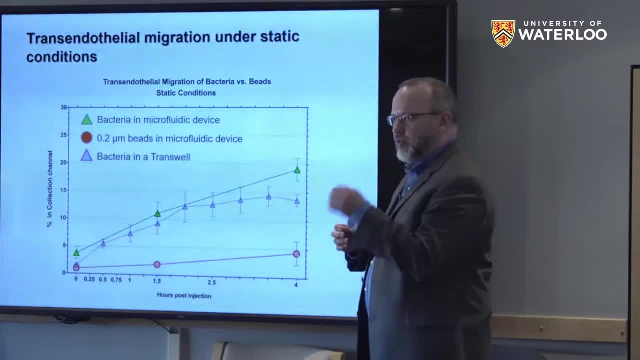 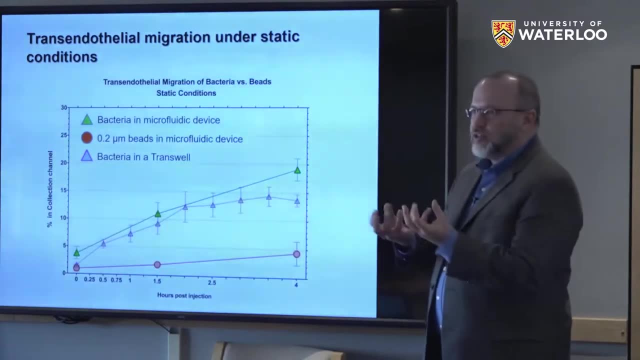 And as a control we use little beads that are the same diameter as the diameter of the bacteria- 0.2 microns- Because the concern here is that the endothelium isn't completely intact And if you have holes in your endothelium, bacteria will just go through the path of least resistance and go through the holes. 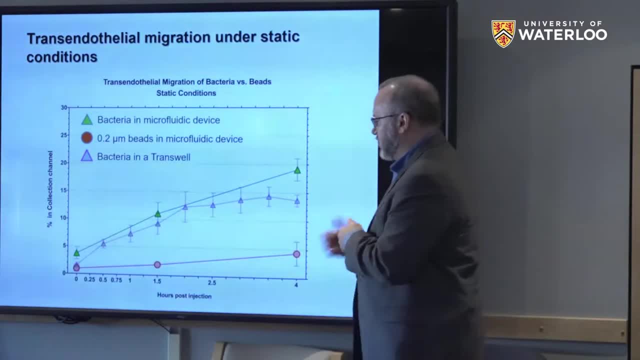 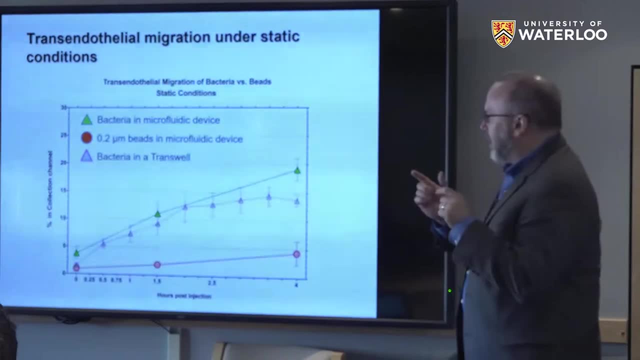 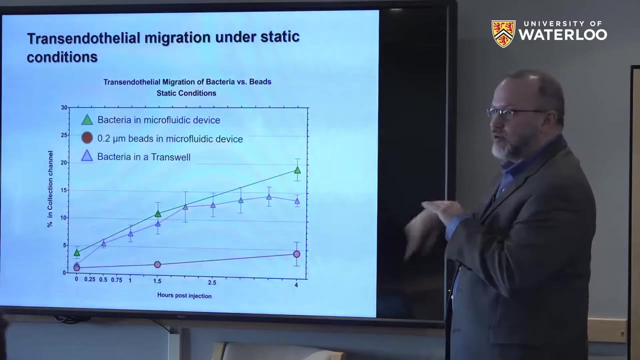 And we'd expect that to be the same, Same with the beads, And we don't really see any substantial leakiness. So that gave us confidence that this is actually an active migration mechanism. The bacterium are somehow either wiggling through the endothelium or actually there's evidence they can pierce in the cell and come out the other side of the cell without killing it. 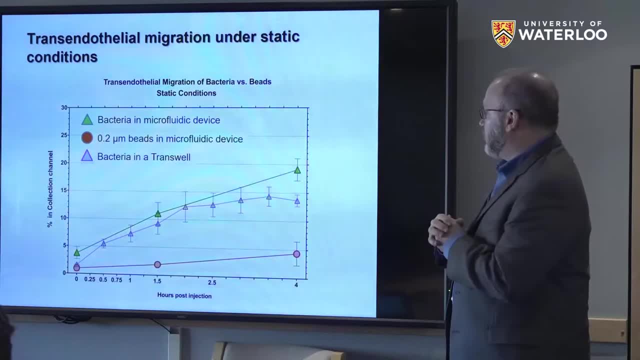 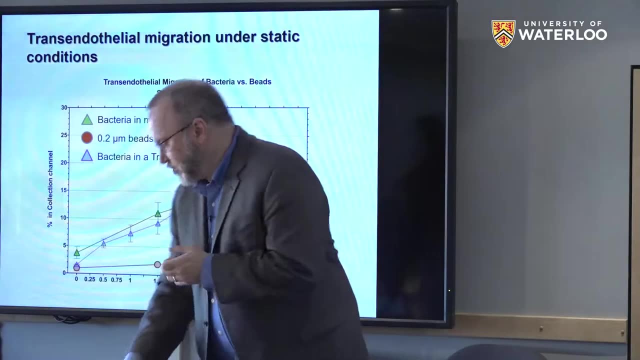 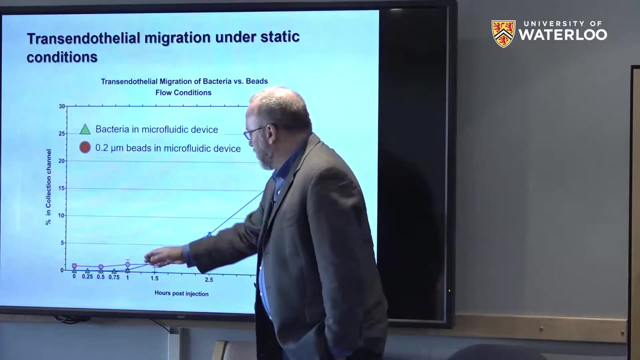 And so that's what these sorts of tools will now allow Terra to study in much more depth, with much more mechanistic understanding. We've also done under shear, and, as you might expect, under shear the dynamics change. What we find is there's a lag before there's any bacteria going through the endothelium, and then it increases over time. 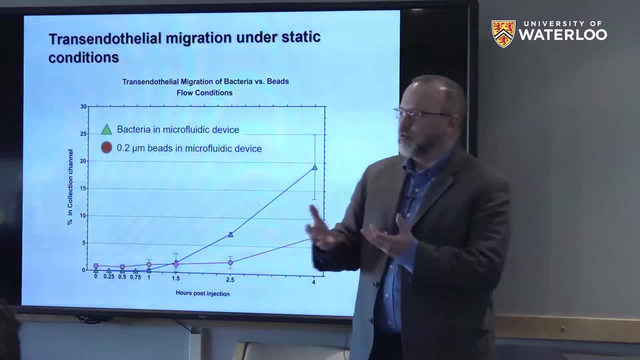 At four hours in this set of experiments at least, we saw the endothelium start to break down. So we don't think this is really representative of active migration at this point, And you can see that we got more beads coming through at this point. 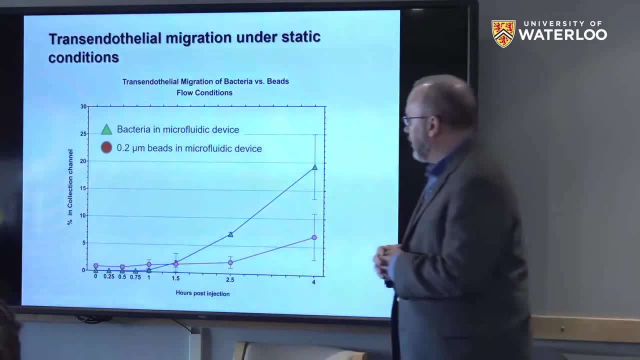 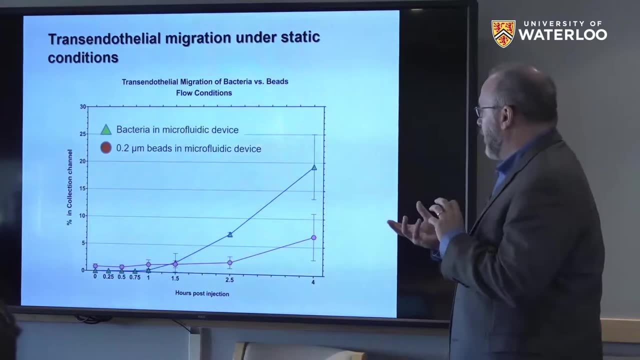 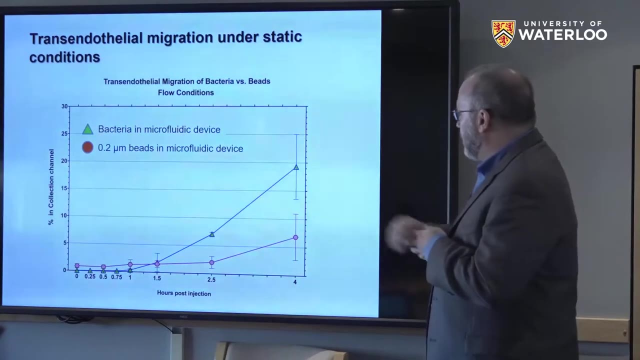 But certainly up to two and a half hours where we don't get many beads at all getting through. we see this active migration that is delayed a little bit under shear. So you know, we think that Part of that's just because you have to build up enough bacterium and they're not. their transit time is much shorter under flow. 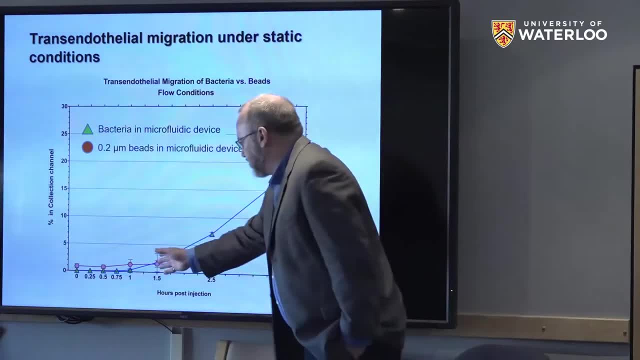 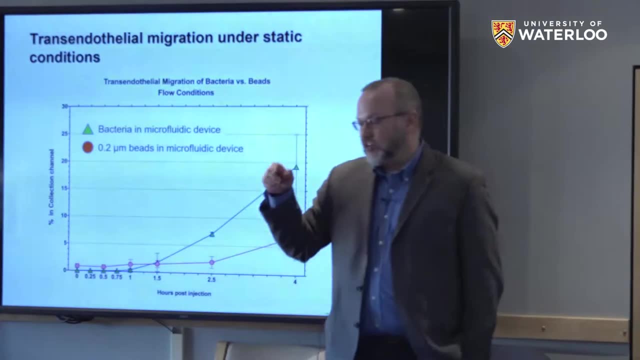 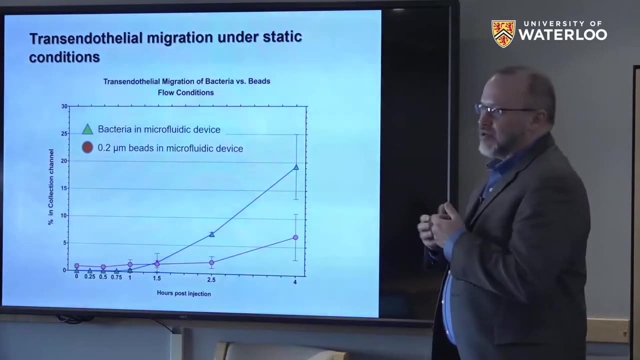 So we think this is not necessarily this lag, isn't necessarily physiological, But what this system now lets Terra do is start studying the mechanisms by which the bacterium are able to adhere to an endothelium and then squeeze through. And the bacteria are nice because you can knock out any gene you want and start studying. you know, does this gene have a specific role in migration? 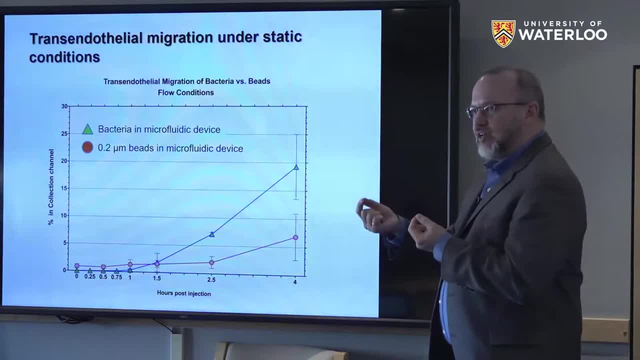 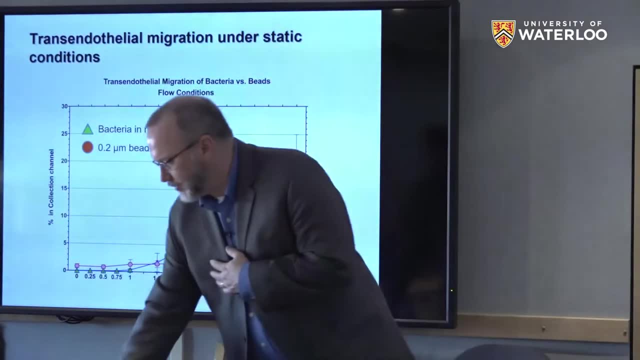 And then you get really mechanistic understanding And are there things you could target? Are there targets for drugs that would prevent them from getting out of a blood vessel? So that's one type of application. In that case we had nothing in the bottom channel. 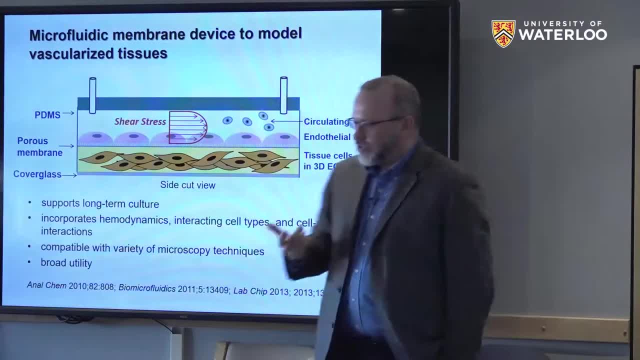 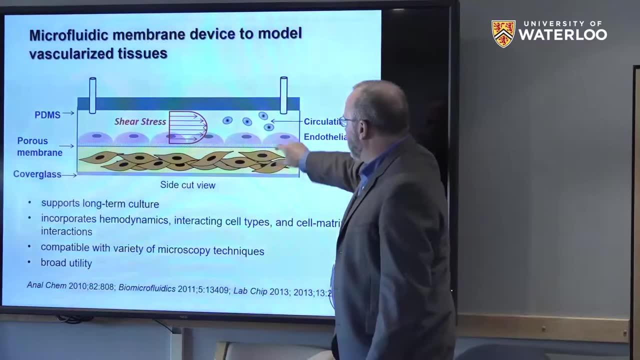 And we just looked at cells migrating through the layer, The other example I'll show you. I think the utility is to model where you now actually have a tissue down here And you're interested in how these cells might communicate with these cells, And so this is an example that's from my own research. 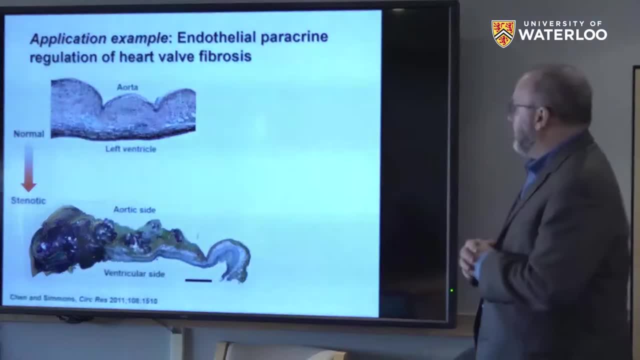 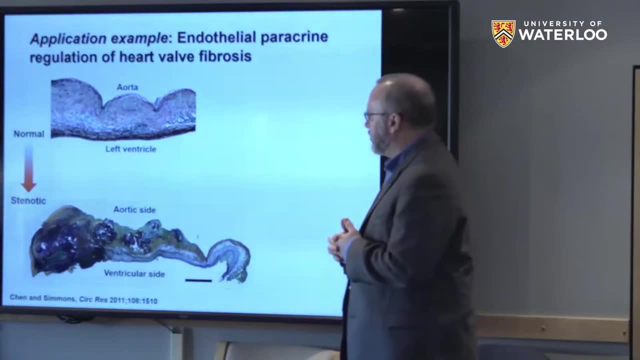 We do a lot of work in heart valve disease and heart valve regeneration And the most common heart valve disease is aortic calcific or fibrotic aortic valve disease, where the normal aortic valve shown here in cross section becomes this: So this is nice: three layers of nice collagen, elastin and proteoglycan tissues And at the end here the end stage disease. it's calcified, There's actually chunks of bone in the valve And there's a lot of scarring. 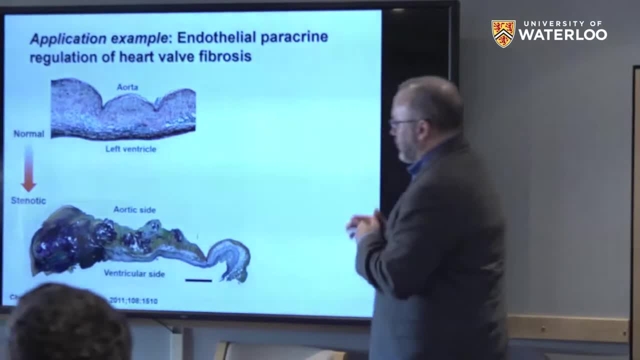 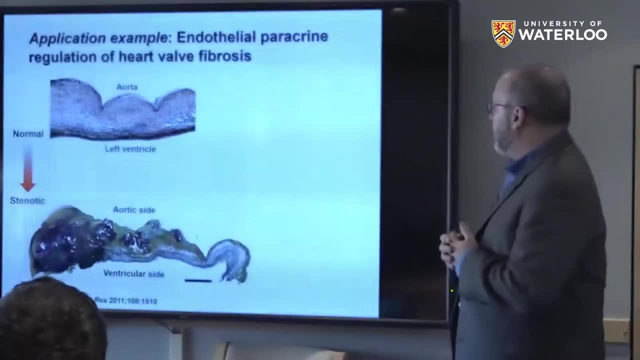 So the bone is the purple and the green is the scarring, And so this change actually causes dysfunction of the valve. If you have severe disease like this, you'll die within two years, And the only solution right now is to cut it out and replace it with an artificial valve. 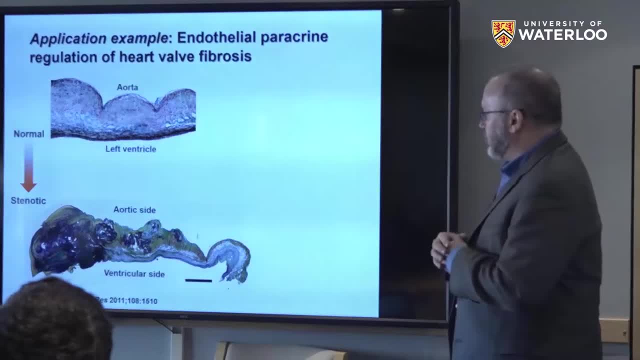 And so we're quite interested and others are quite interested in: is there targets or drugs that could be applied earlier on in the disease to prevent this progression from occurring? What's interesting about the disease from a biomechanics perspective is that the disease occurs primarily on one side. 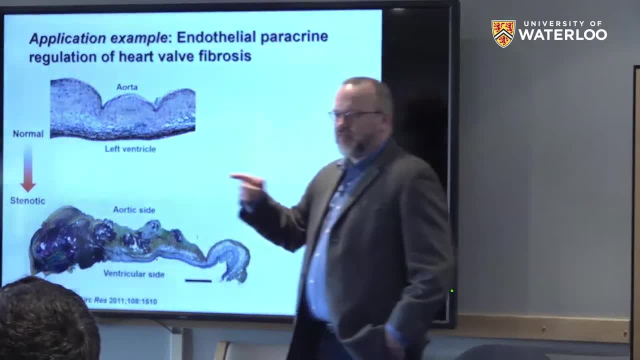 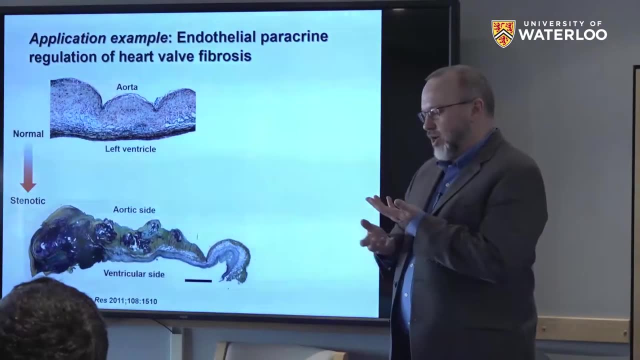 It occurs on the aortic side, the side that faces the aorta. So this valve is between the left ventricle that pumps blood and the aorta that takes blood to the rest of the body, And it's the back side of the valve. 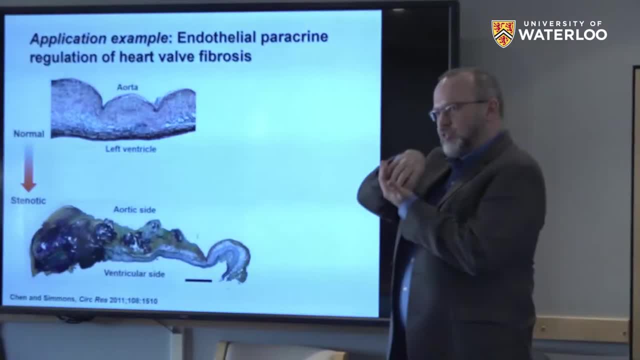 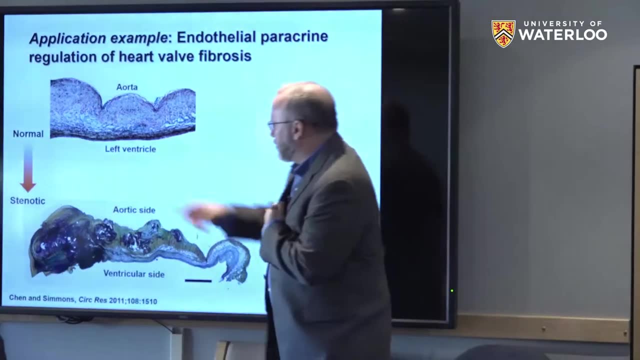 So the heart pumps like this, the blood shoots out. It's this side of the valve that becomes disease, not this side, And you can see that here. This is where all the calcification and scarring occurs. This side is relatively untouched. 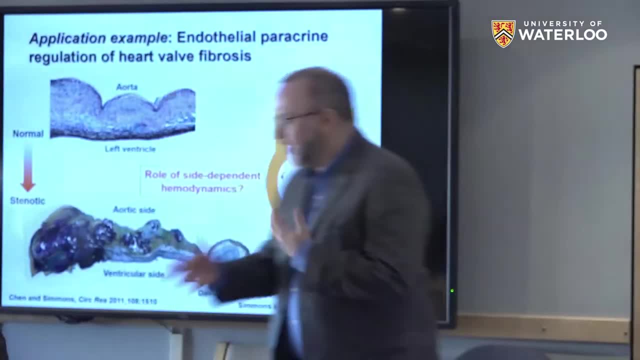 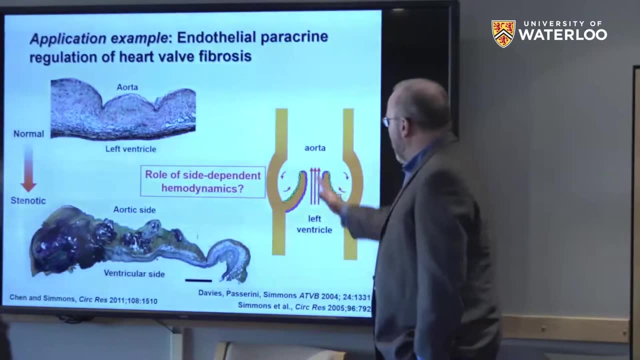 And so we asked: is it the blood flow that is regulating this? Is there a role? And the answer is the fact that when the heart pumps, the blood coming out of the heart is very high velocity, generating high shear stresses on this side of the valve. 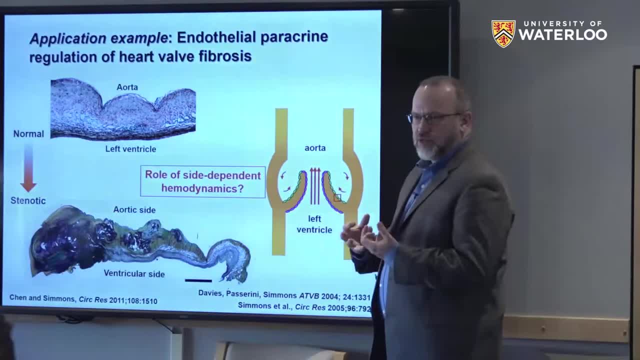 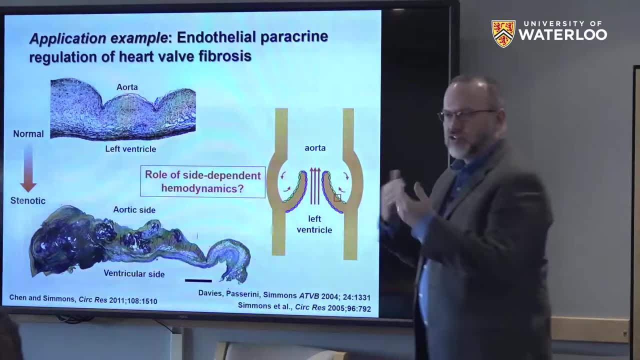 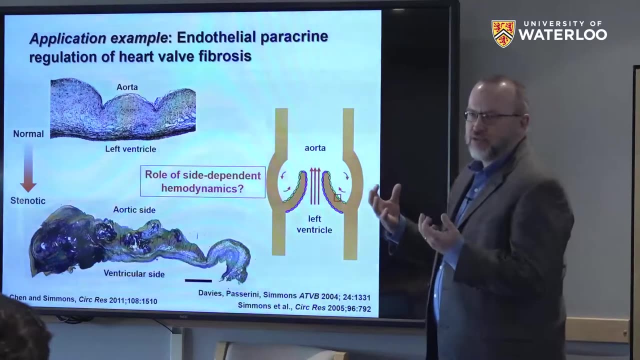 Whereas on the back side of the valve the shear stresses are much lower and disturbed. And is it the differences in hemodynamics which correlates with the differences in disease susceptibility? is there a link there? And this is difficult to study in an animal, because it's difficult to change the blood flow without doing lots of other things. 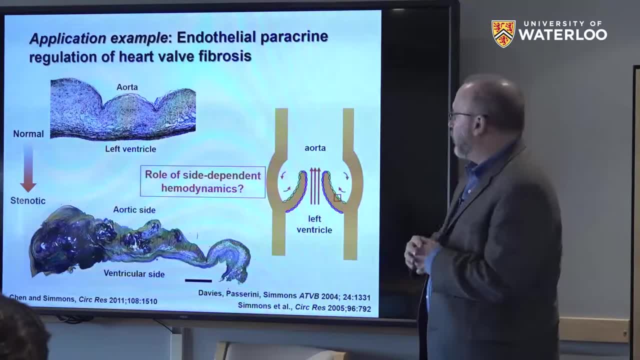 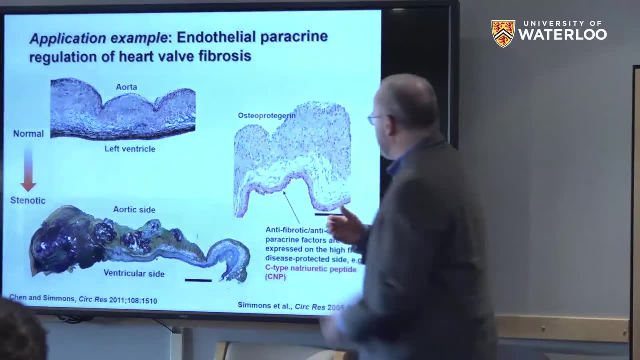 And so if you had an in vitro system to start asking these questions, that would be quite useful. We know this is important because we now, or now, we know it's important because, if we look at the expression of proteins that are known to prevent fibrosis or calcification, 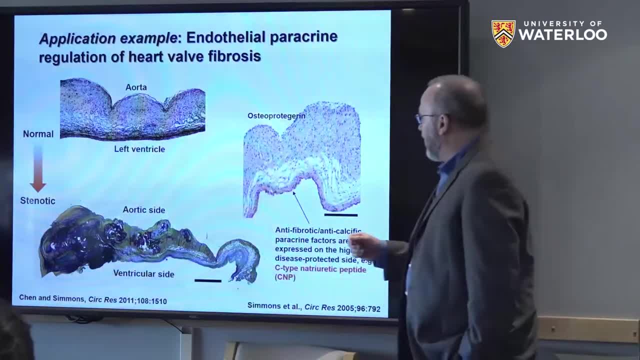 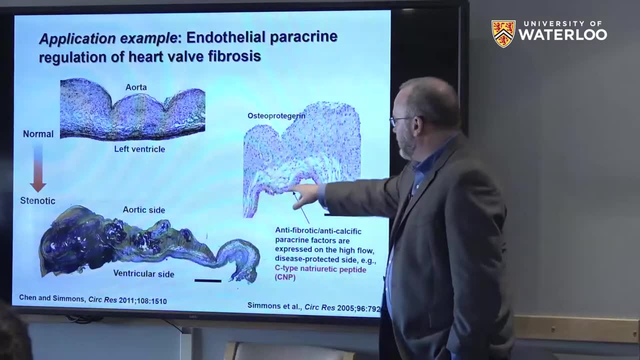 we see that they're higher expressed on the disease-protected side of the valve and lower expressed on the disease-prone side of the valve. So our hypothesis is that the high shear is causing the endothelial cells here to make these protective factors And that's helping to protect this side. 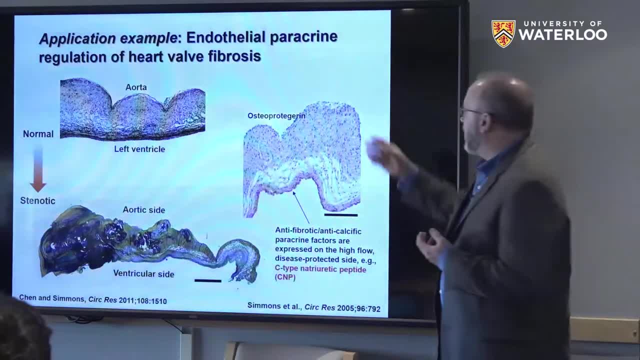 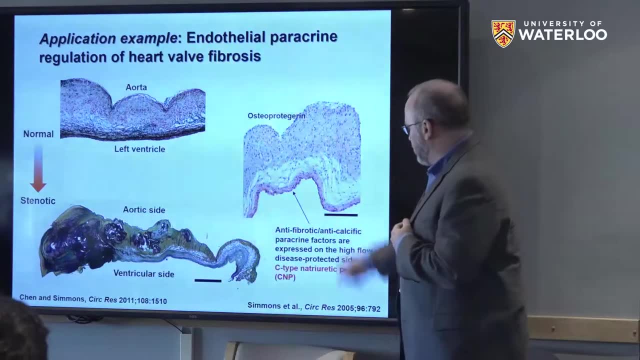 Whereas this side, the endothelium, is not making these protective factors, And this side is then prone to disease if you have a diseased animal- And one of those ones we discovered through this early on was through the C-type natriuretic peptide, which was expressed here but not here- 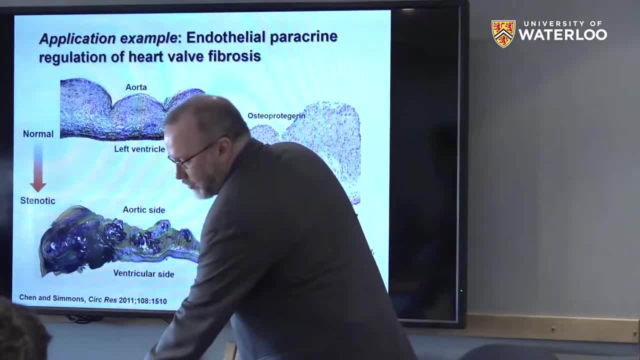 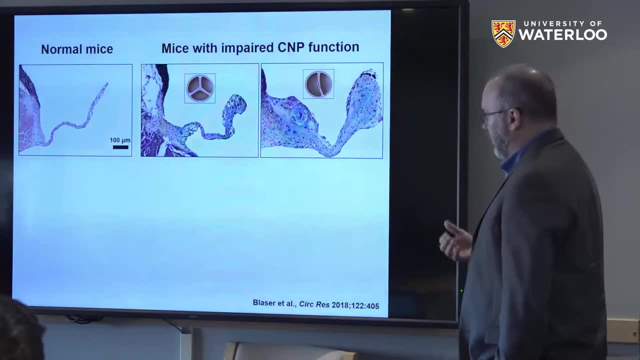 And just recently we've shown, if we knock this out of a mouse, here's a normal mouse valve. And then here's a mouse valve where we've inhibited its CMP function or impaired its CMP function And you see the valves get thicker. In some cases they become bicarbonate. 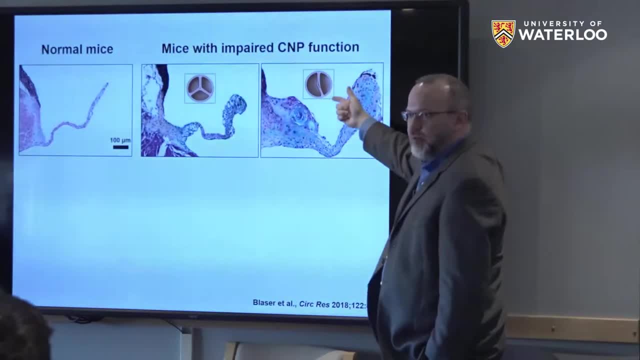 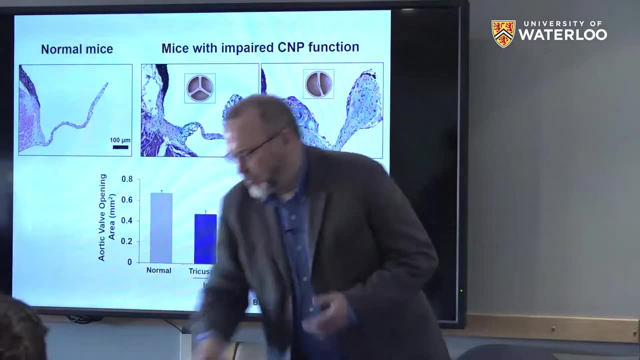 In some cases they become bicuspid. So the mouse is born with the most common congenital defect in humans, bicuspid valves. And their valves are even worse So CMP, and we see this in terms of the function. the diseased valves just don't open as much as the normal valves. 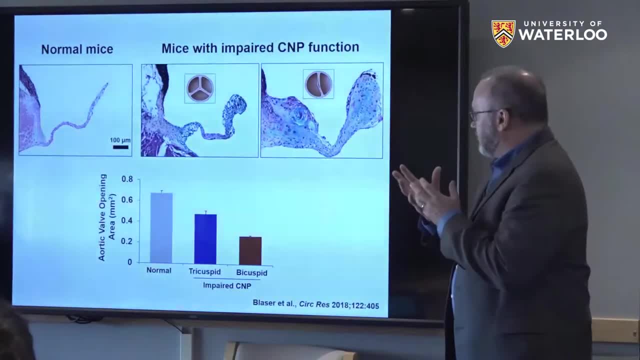 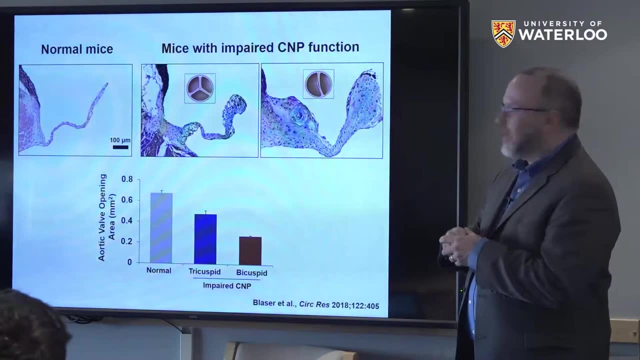 So they do that, they don't do that. And so this clear, now functional demonstration- this we just published last month, this clear, functional demonstration- that CMP protects against heart valve disease. But we still don't know why it's. why is it high on one side and not the other, and is there anything we can do about that? 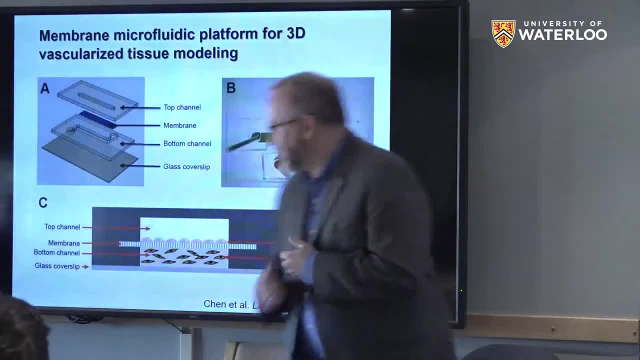 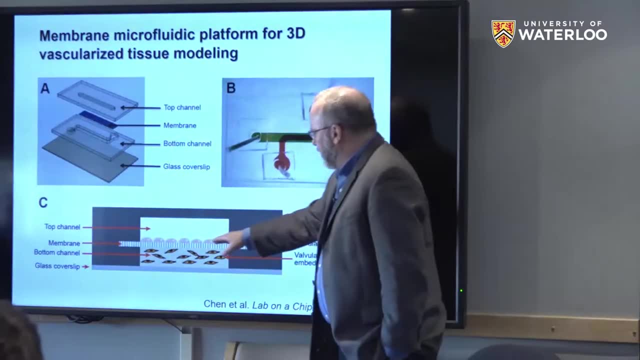 So we've been using our microfluidic system to start to study that. So in this case we have again the two channels on top of one another. The valve endothelial cells are on the top, they're in pink on the membrane And then in the matrix. here we grow the valve. they're called interstitial cells. 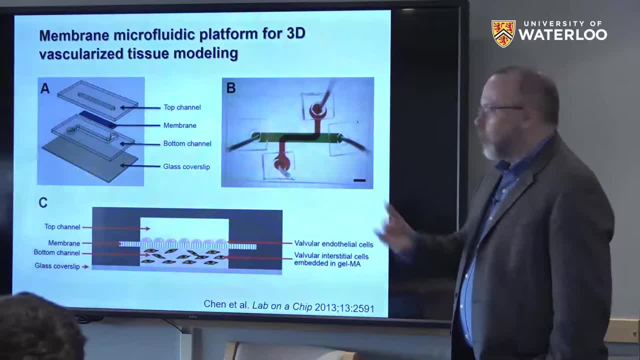 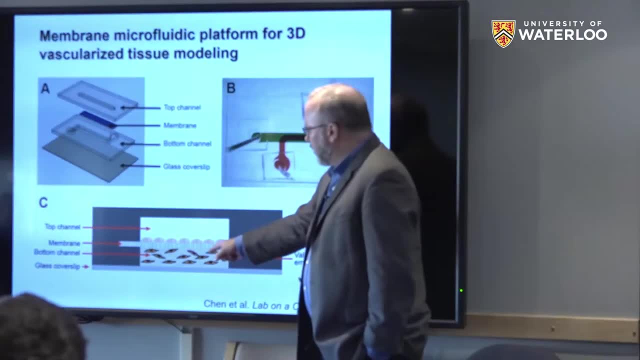 They're the cells that will cause the scarring and bone formation, And we embedded those in a biomaterial image And then in the bottom, here and again, we have this ability for the cells to communicate, and particularly the endothelial cells, to secrete these factors. 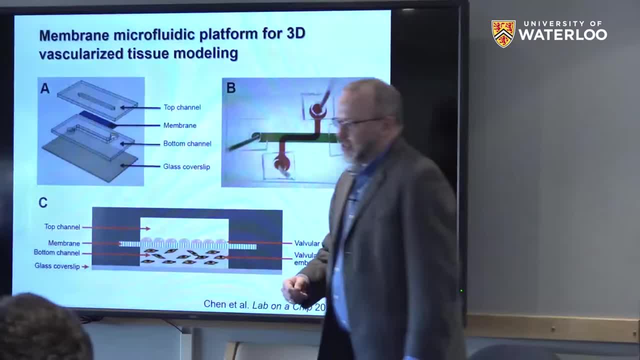 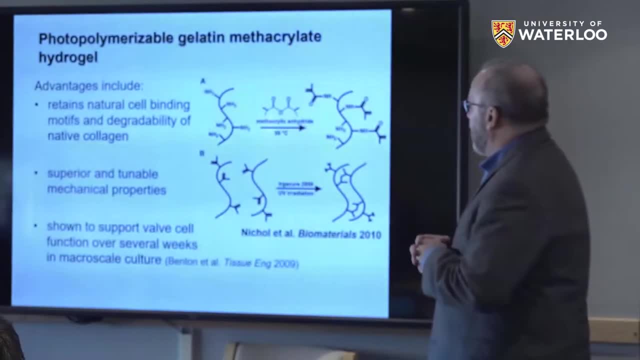 to maybe prevent disease down here, all under shear stress, And so the biomaterial we use is a photopolymerizable gelma or gelatin methacrylate. It has components of collagen in it which allow the cells to bind to it. 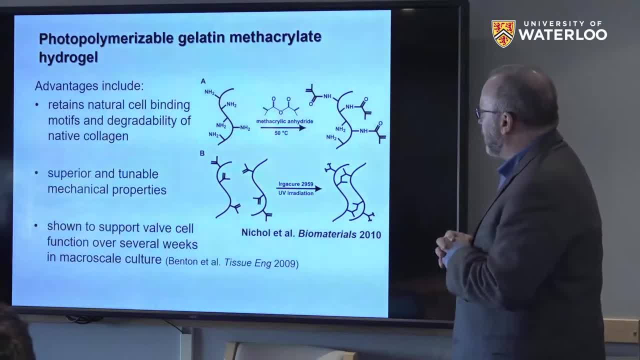 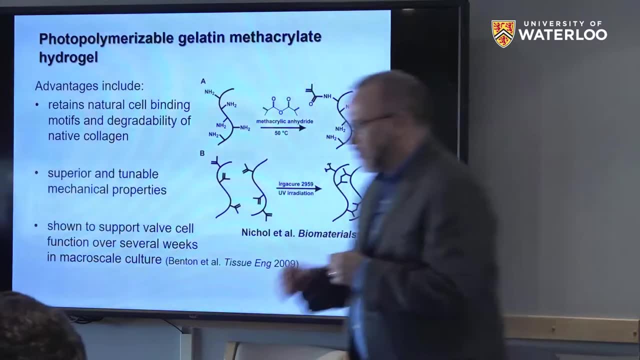 But because it's because it's methacrylated and UV curable, we can tune its mechanical properties, And so we actually tune them to mimic the actual properties of heart valve tissue, which we know is important for the function of these cells. 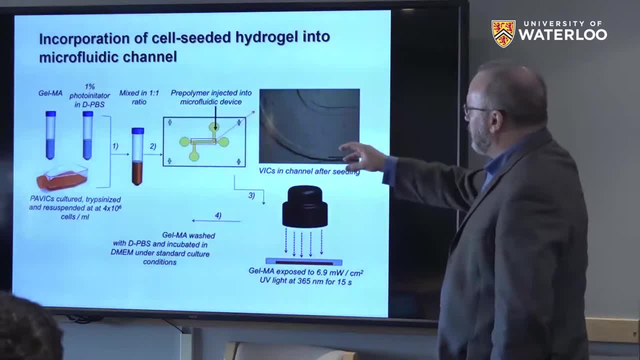 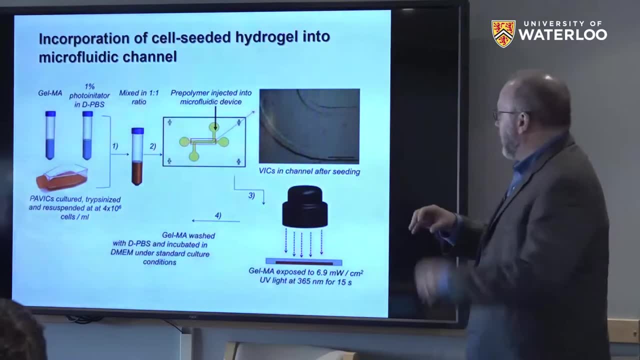 And so the approach we do is we mix the cells with the polymer and the photoinitiator, inject them into the bottom channel and then photopolymerize them straight in the channel. So we have then a gel forming within the channel with cells embedded in it. 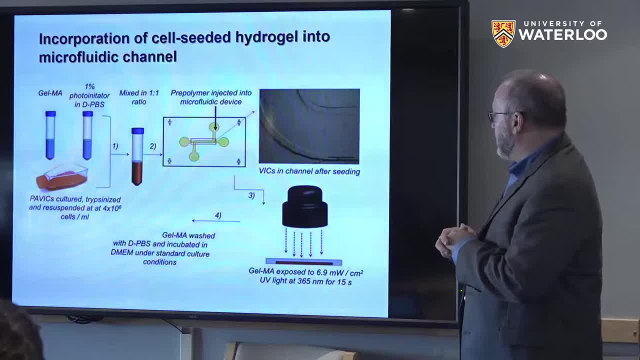 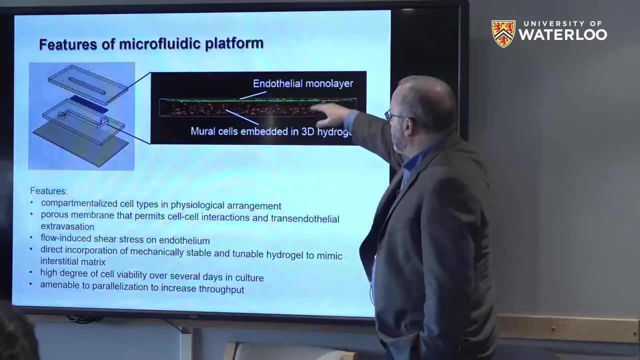 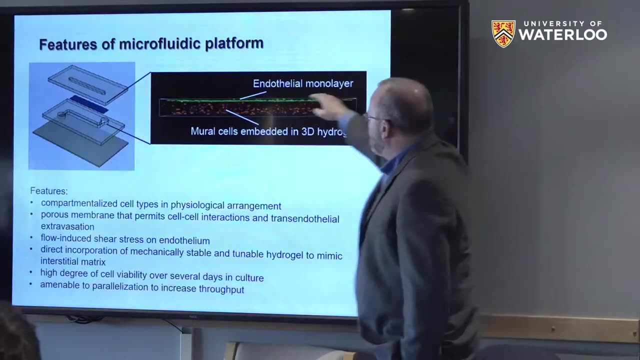 and then we can wash out any unpolymerized matrix or substrate, And so what we end up with and with is shown here. in cross-section You see the cells in red. those are the valve fibroblasts. They're embedded within a 3D biomaterial and then they're lined with an endothelium. 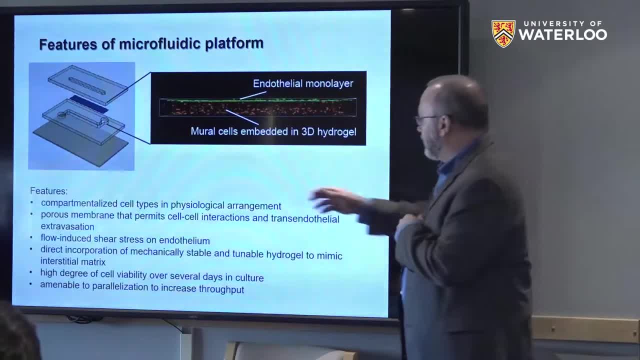 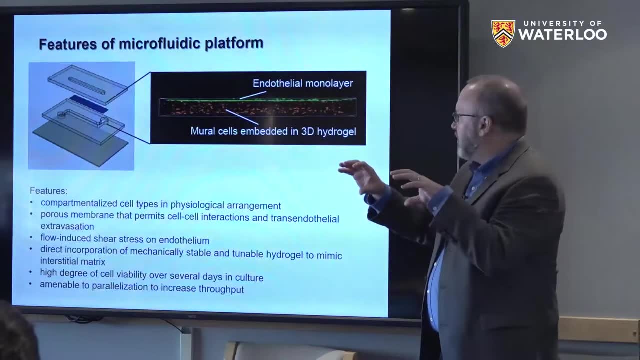 the valvular endothelium and again, we then recapitulate this physiological arrangement. We have the endothelium on the surface, in the flow channel, and then the 3D biomaterial with the cell, the fibroblasts, embedded in the lower channel. 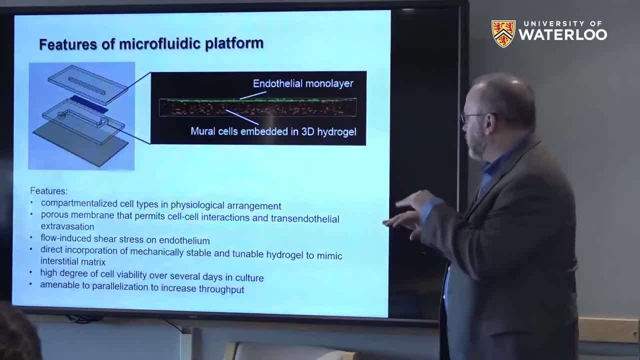 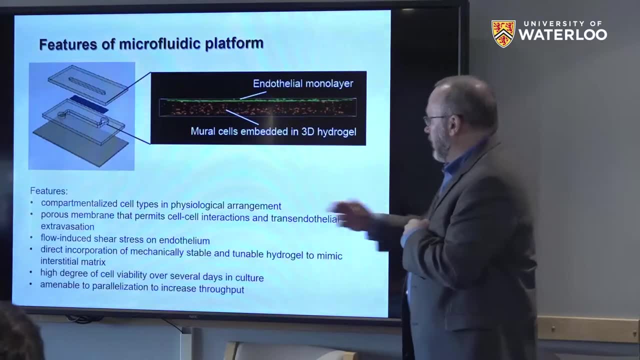 And they're separated by a porous membrane. that again allows the cells to talk to one another, also allows things to crawl through the endothelium. We saw bacteria, but it could also be inflammatory cells. We can apply this shear stress on the endothelium to mimic what's going on in the heart valve. 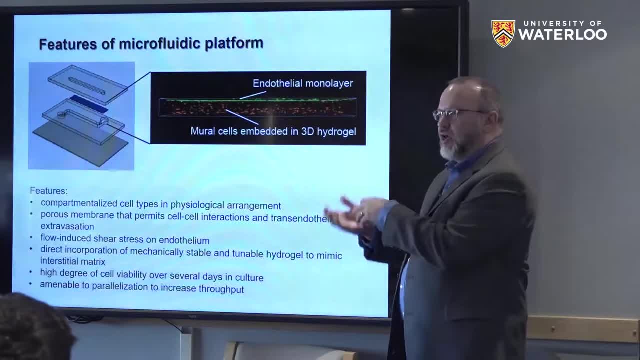 and now ask: does high shear stress produce protective factors? and low shear stress not produce protective factors? And we've been able to tune the system to recapitulate the tissue properties, And we've been able to do this over many days. grow them over many days. 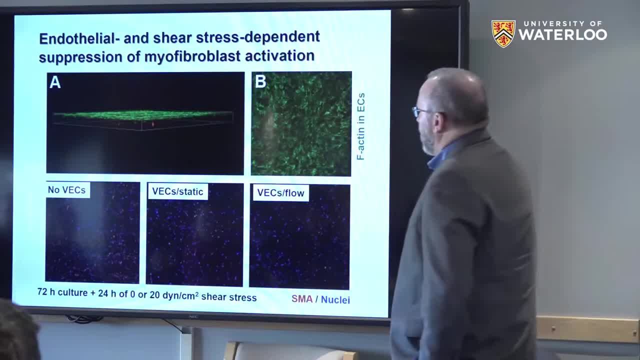 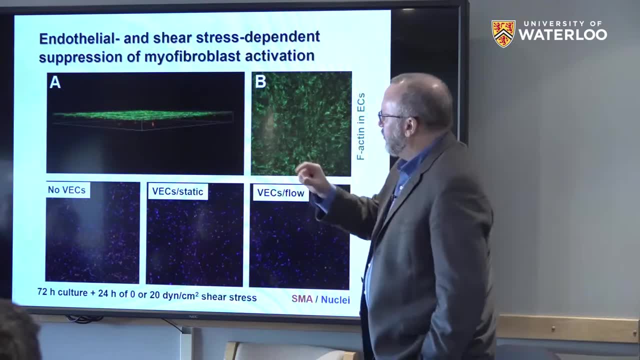 So here's an example of the sort of data we get out. So again, what's shown here now is the endothelium. the endothelial cells are in green. This is looking face down on them And in the bottom channel. what we've done is we've stained the cells for a marker called alpha smooth muscle actin. 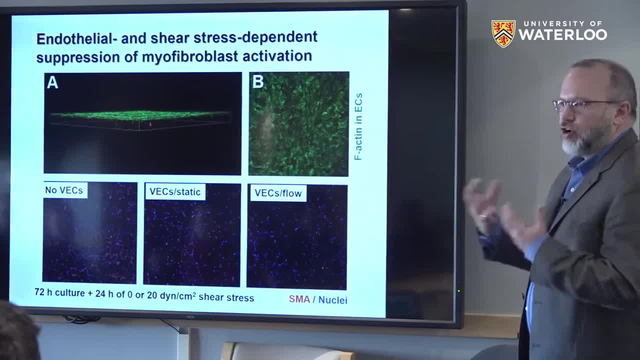 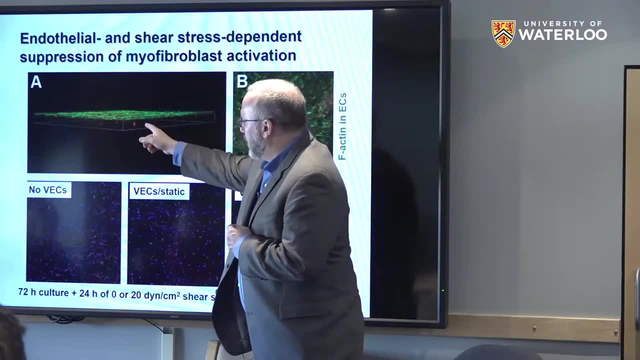 This is a marker of the cells becoming more fibrotic or scar-like, So it's a disease marker in these cells. And so if we have the interstitial cells, the fibroblasts, in the bottom channel, with no endothelial cells on top, 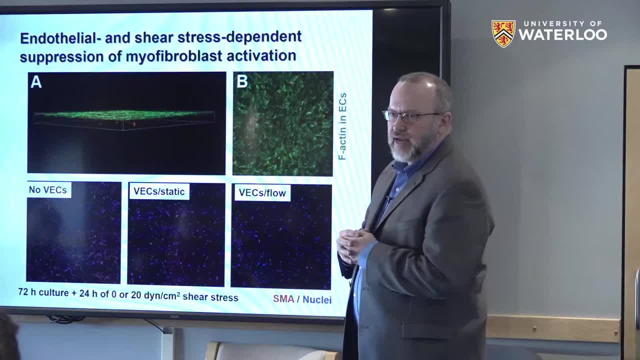 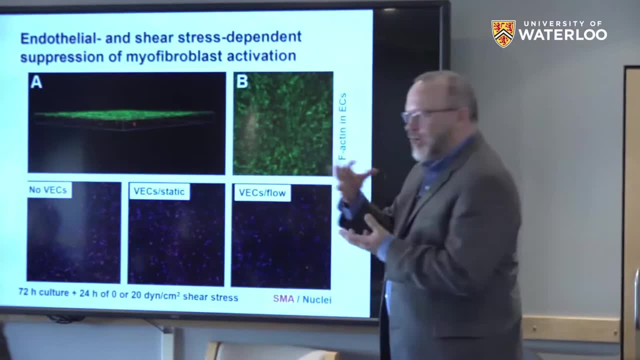 you can see that many of the cells express this SMA, this alpha smooth muscle actin, So they're in a disease phenotype. If we add the endothelial cells and grow them under static conditions, something about the presence of the endothelial cells suppresses this expression of SMA. 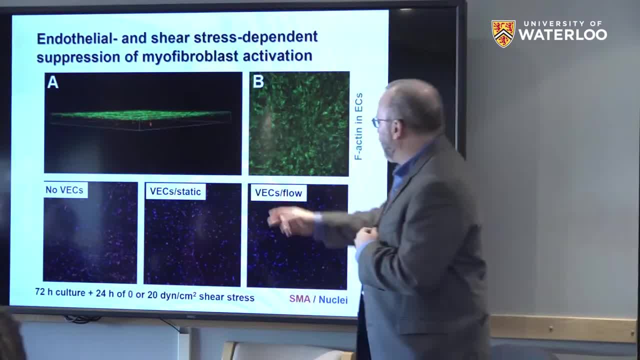 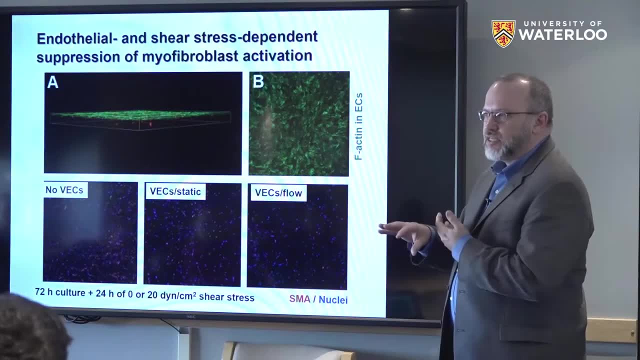 So they're less diseased, they're more healthy. And then if we further include the endothelial cells and subject them to flow, we see even further suppression of SMA in these underlying cells. So the endothelial cells are presumably, or what we hypothesize. 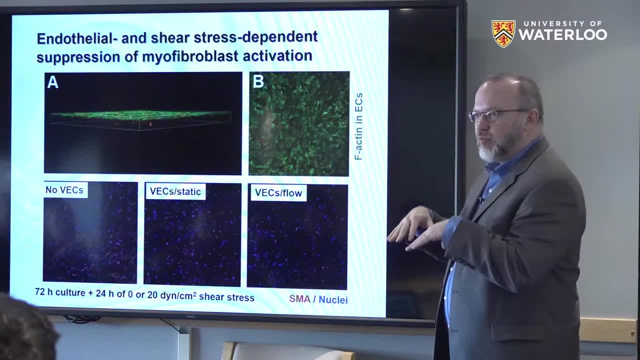 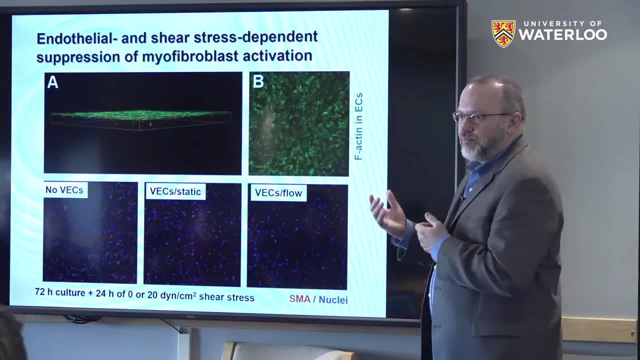 they're secreting something that is getting to the interstitial cells, the fibroblasts, and putting them in a more healthy state, And the endothelial cells presumably make more of that under flow And if you quantify the numbers, you can see that we see the same thing. 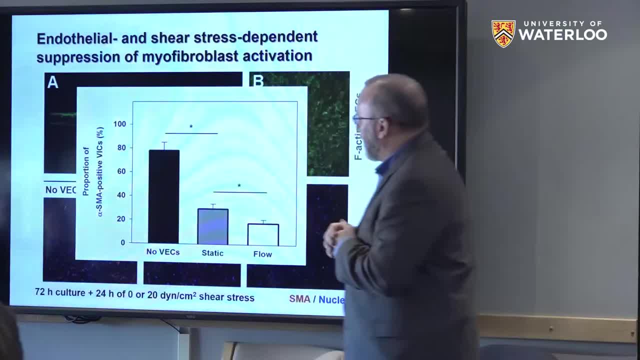 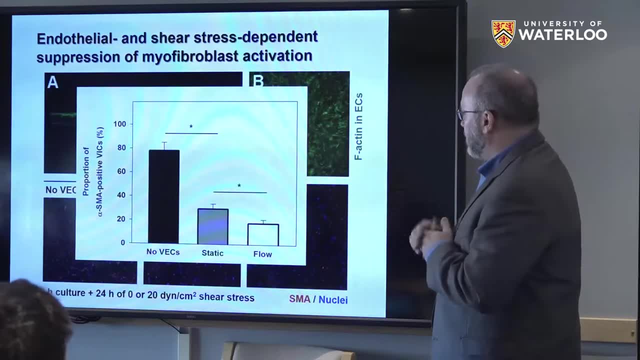 That these alpha smooth muscle actin positive valve interstitial cells- there's a lot of them- without the endothelium, and the presence of the endothelium alone helps normalize them, And if we further add flow they become even healthier. So one question is: is it the C-type nitrate peptide that we're working on? 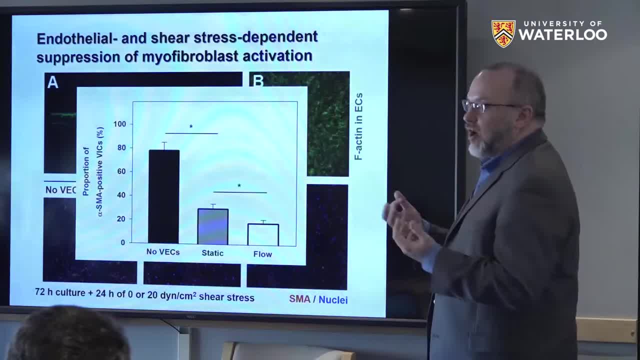 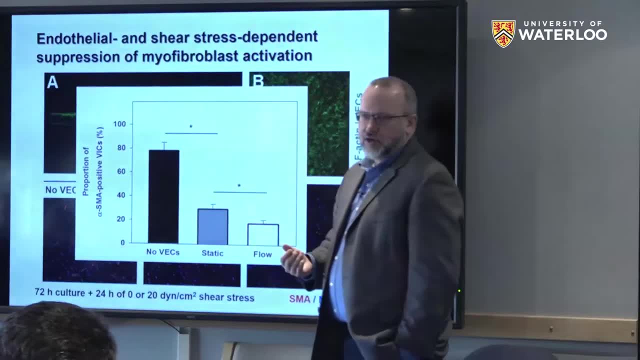 Is this the factor? We're studying that right now, Or are there other factors being secreted Under flow conditions or high shear conditions that are not being secreted under low shear conditions? So this is going to help us, we think. 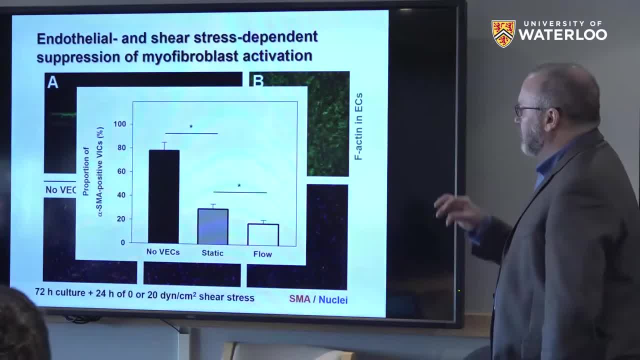 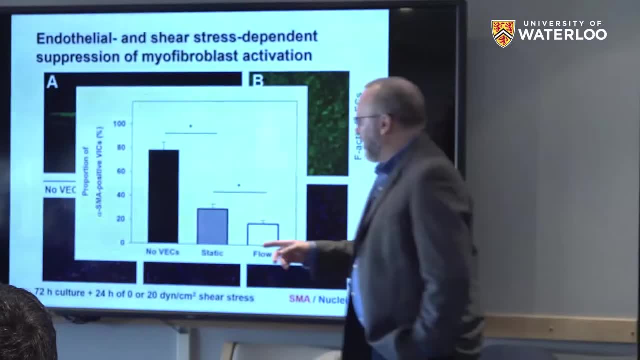 both understand fundamentally what's going on in the heart valve, but also maybe identify other factors that are flow regulated, that are protective, that we weren't able to find in vivo. Maybe we'll find them in vitro and we can chase those as potential targets. 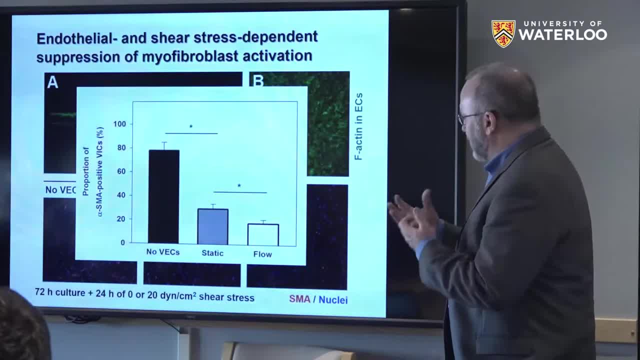 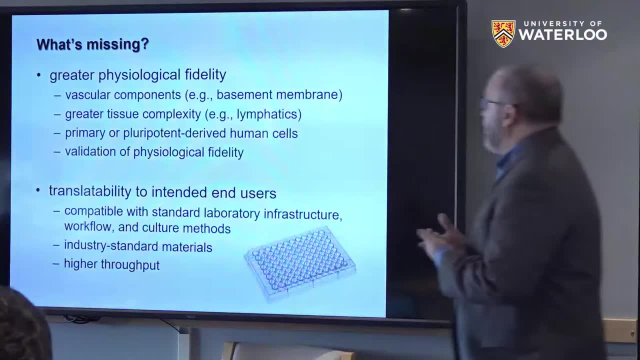 So again, nice, I think, illustration of the sorts of experiments you could do with it or can do with this system. So what's missing from this system? Well, one, I think that we, as I mentioned, we have in some ways sacrificed some physiological fidelity. 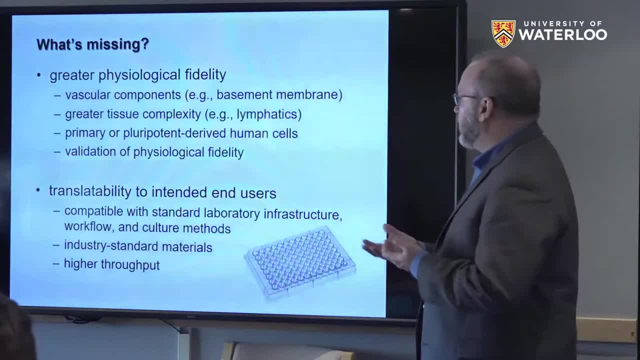 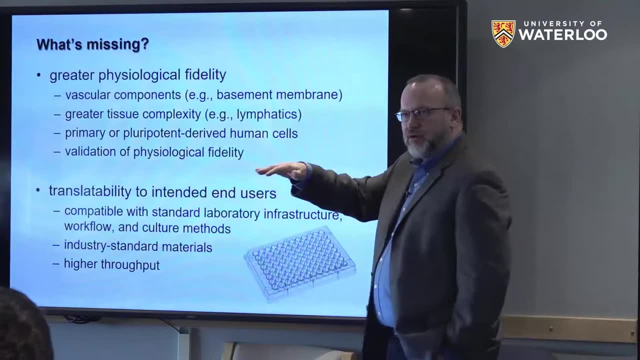 to get a system that's relatively easy to use- And that's been kind of a driving force throughout this and I'll talk a little bit more about that. But we could imagine introducing- we have a membrane in there which is not physiological. 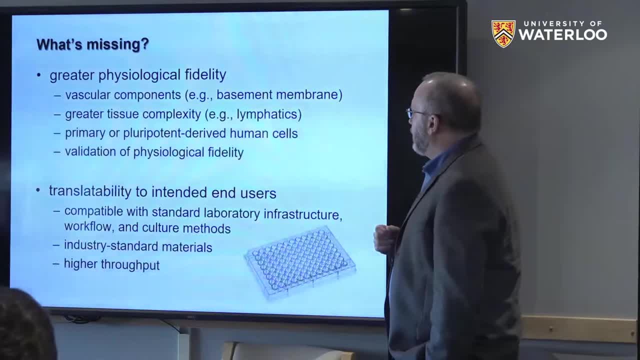 We could perhaps replace that with a basement membrane. Have to think about that. We could include different complexity in the tissue. For example, we don't have any lymphatic system in there. That might be important. We can, and we have been using human cells. 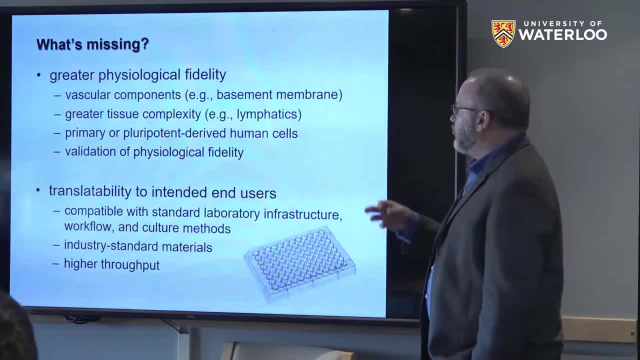 So we're starting to use now pluripotent-derived human cells So we can even do disease modeling, where you could get a blood cell from a patient who has a specific disease and then convert that back to a pluripotent stem cell and then derive that into an endothelial cell. 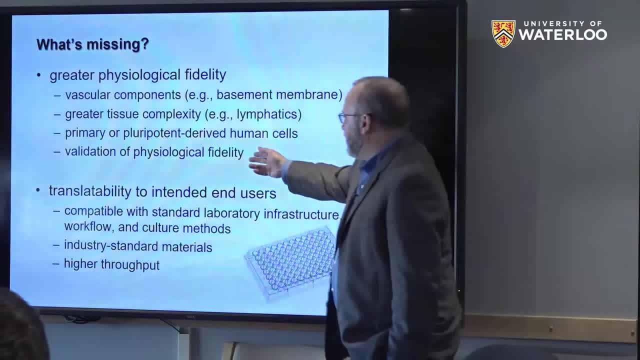 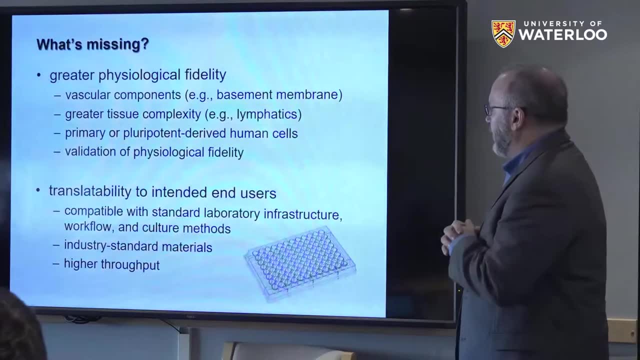 So we can start doing human biology on these, And this is a big one. You have to validate that, that what you're seeing in the chip is actually happening in the body, And so this is the other aspect that we're working hard on now. 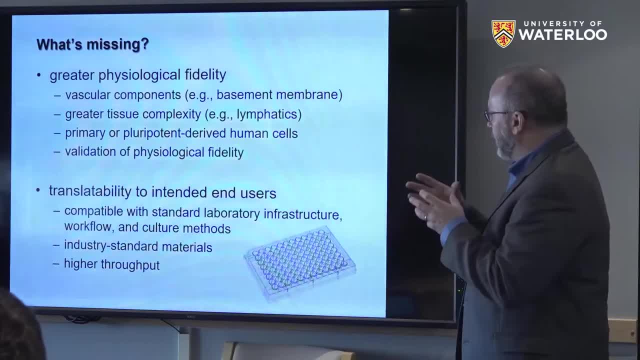 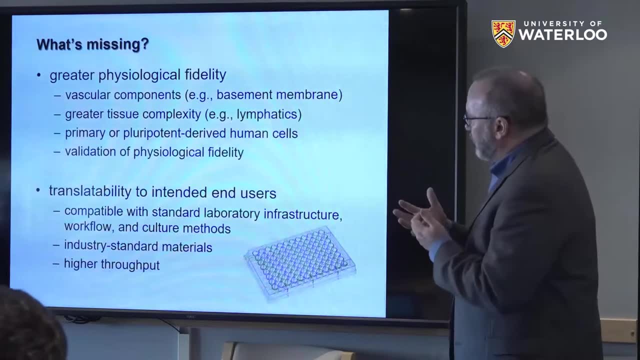 for a variety of systems is: can we demonstrate that the biology that we see on the chip or on the plate matches what we see in the body? The other, I think, really important problem or issue- and this was just, it was in Nature Materials- 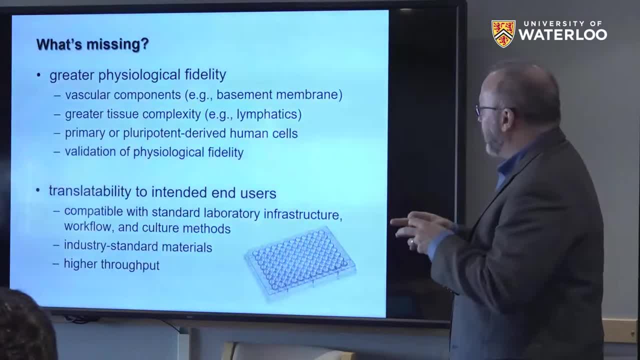 there was an editorial on this just yesterday- is that microfluidics right now, a lot of it are not translatable to end users. So people make these cool devices in the lab that they can work on, like the PhD student working on it. 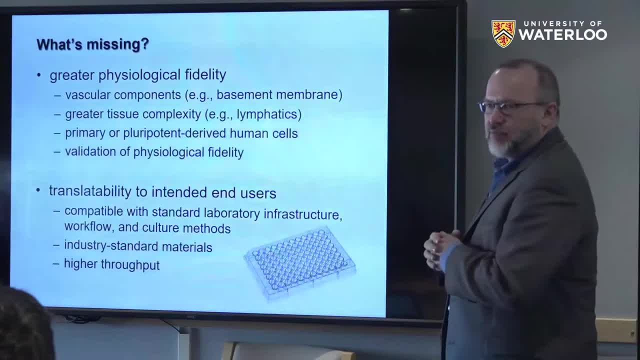 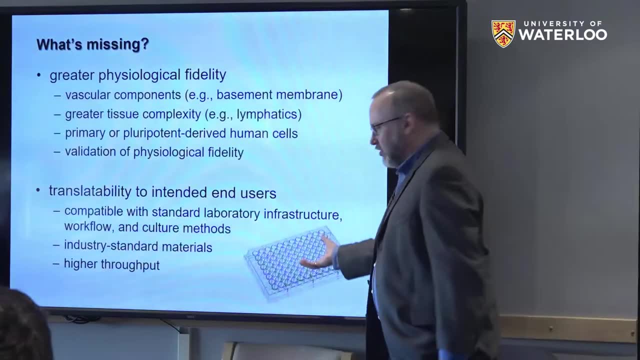 but if they go to hand it to a biologist it just doesn't happen, That translatability and that is lost. So we've been very interested in: can we come up with platforms that look like 96-well plates or look like tools that biologists are familiar with? 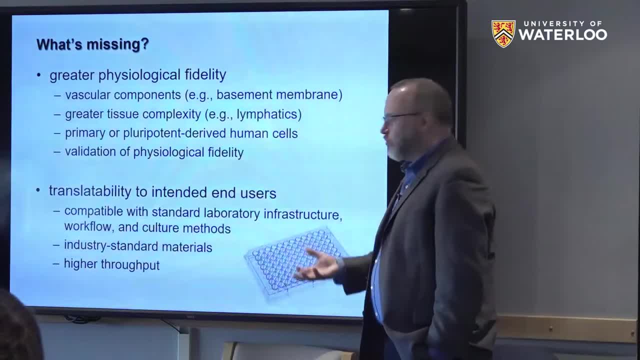 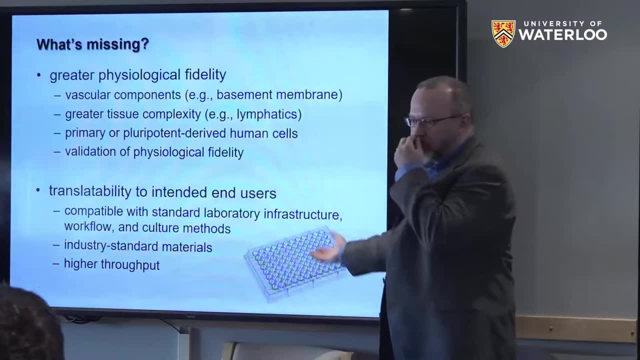 tools that work with the pipettors they have, the liquid handling robotics they have and the methods that they're, the workflow that they're used to? Can we use industry standard materials that aren't PDMS, but use things like plastics that are used? 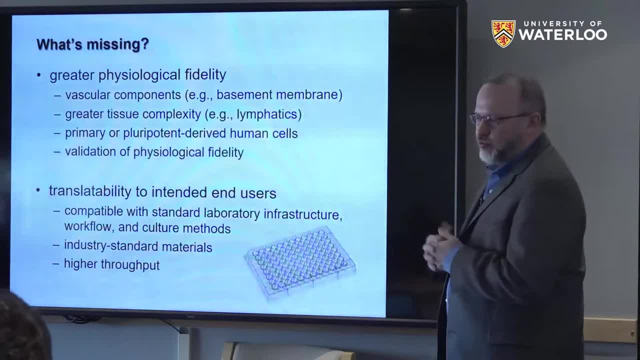 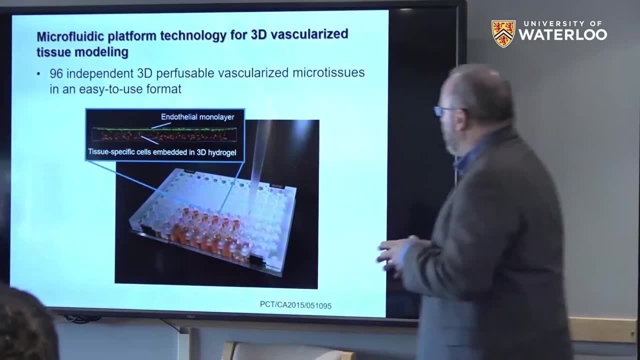 in other traditional well plates And can we get higher throughput. This is of interest for drug development, drug testing. So where we are now is we've come up with a. this is a research associate in my lab. his name's Alex Chabadarov. 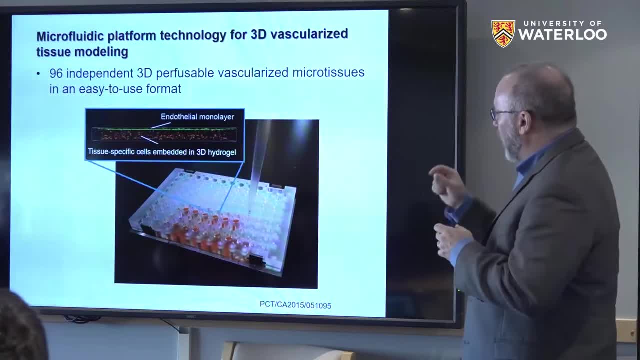 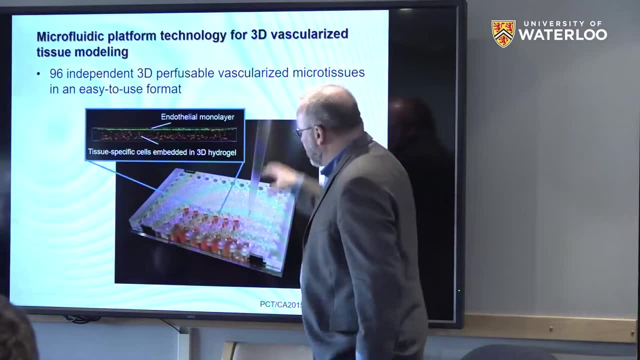 He's come up with a 96-well plate where each well within this plate has one of these micro vascularized, micro tissues. So we use the same principle, but now he's engineered it so that within the bottom of each of these wells, 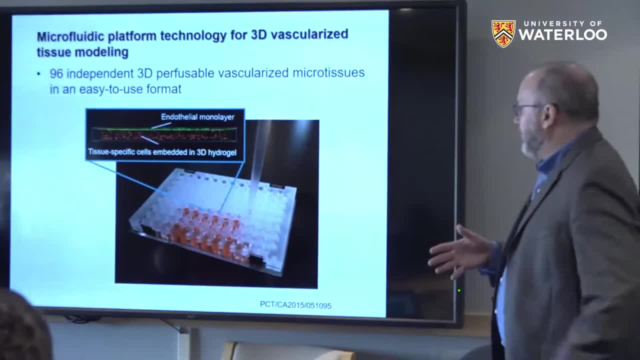 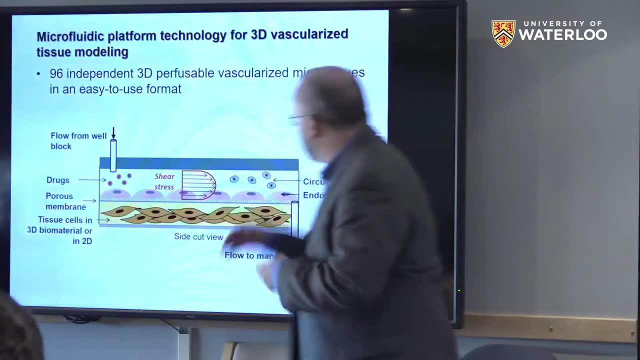 is one of these stacked co-culture micro tissues, And the format, though, is now much more familiar to what a biologist would be familiar with. And, again, that's what it looks like at cross-section. So now, what we can do is we can still have flow. 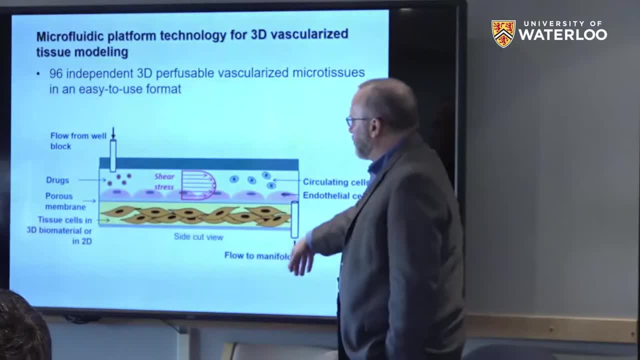 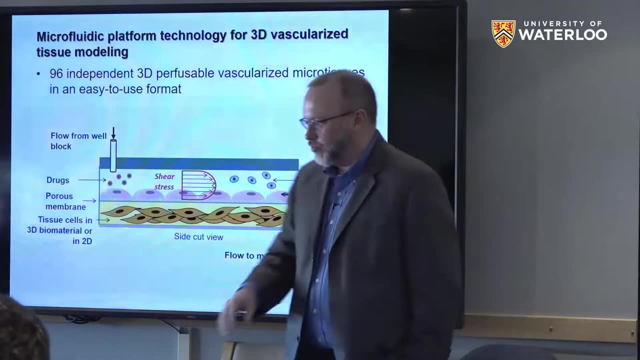 We pull flow through the top channel, It's then pulled into a manifold down here, and each channel, each chamber within the 96 wells is each being fed separately. So we get the throughput. And so what we're, what we think. 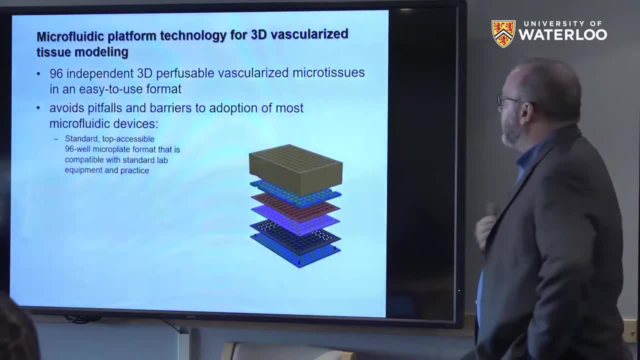 and this is still under development- is that this system avoids many of the pitfalls and barriers that have been prevented adoption of many microfluidic devices. One is: it's a standard format. It's top accessible, meaning you can pipette things in. 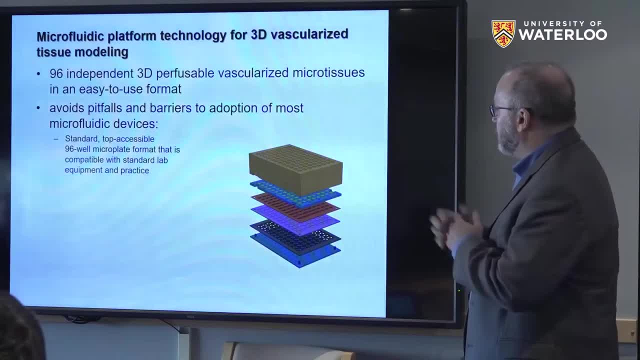 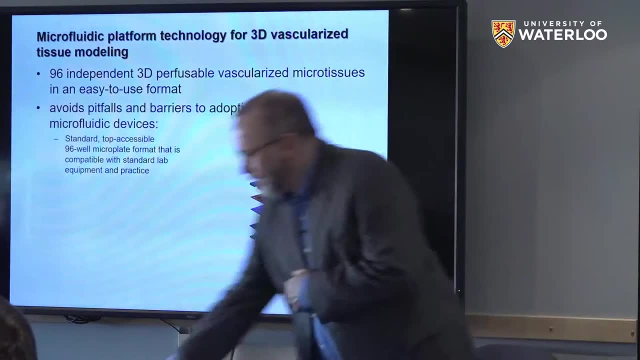 You don't have to pipette things through channels which can cause bubbles and problems. And it's because it is standardized format. it's compatible with standard lab equipment. in practice We regulate the fluidics for a single port, So we just one tube plugged in. 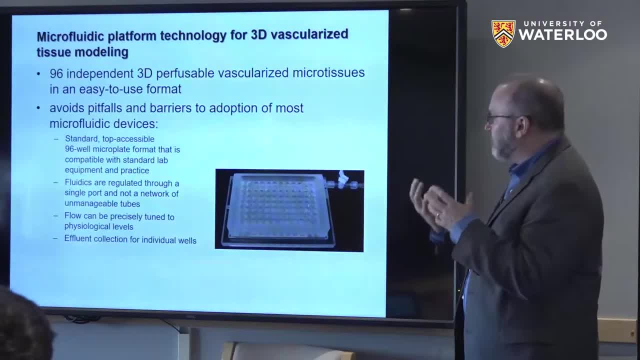 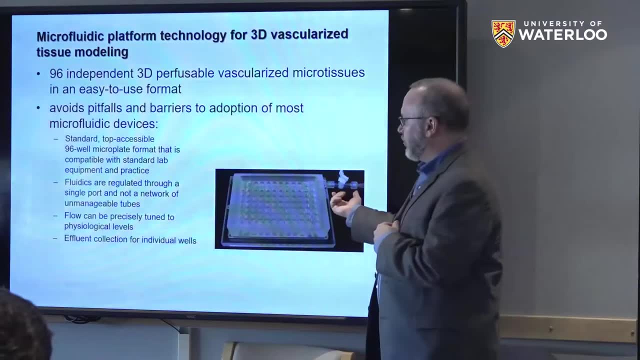 We don't have 96 tubes in and 96 tubes out, which. there are platforms like that, which clearly people are not readily translatable, And we can precisely tune the flow over to physiological levels. So there's a lot of systems that will perfuse your cultures. 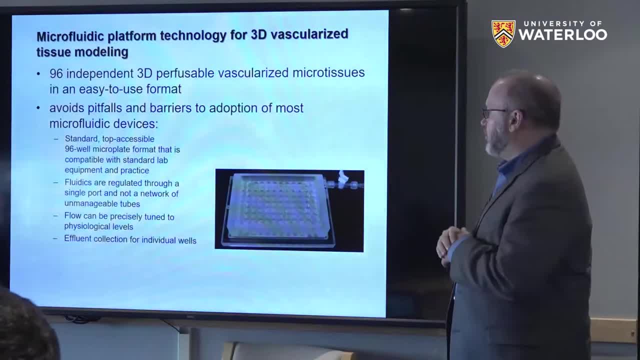 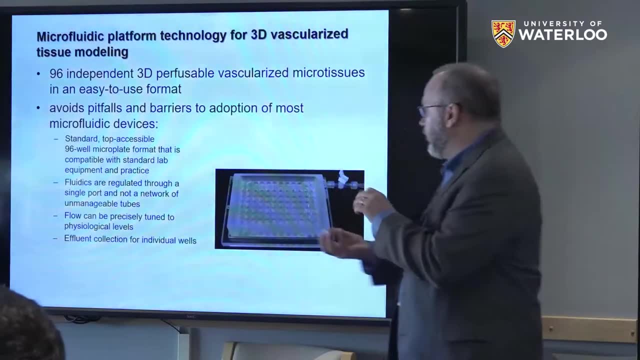 to feed them but not give you actually physiological shear, shear stresses, And so we're able to do that with this system And we've ended in the ordinance that we can actually collect the effluent from each of these individual wells because that might be of interest to sample. 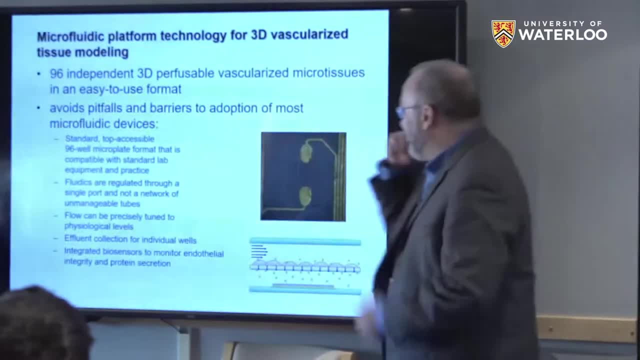 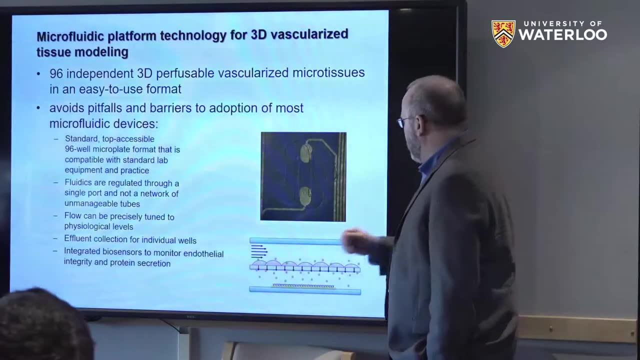 for biological assays. We're also incorporating in some sensors into these systems. So we have electrodes that we can put in here to monitor the quality of the endothelium. We have sensors down in the bottom channel to measure things getting through the endothelium. 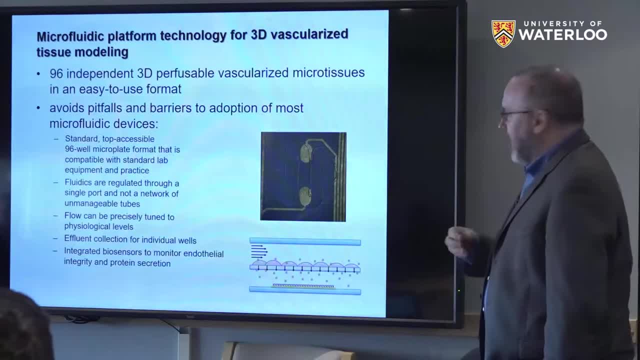 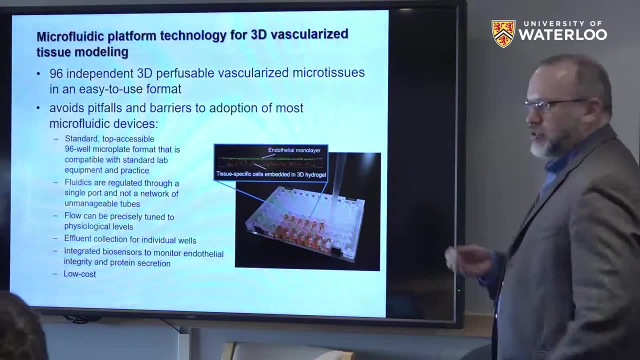 So by integrating these biosensors on the plate, we think we can add some functionality, And the idea behind all this is it will be relatively low cost. A lot of the components are currently available and are readily fabricated, And we're looking to fabricate them even lower cost. 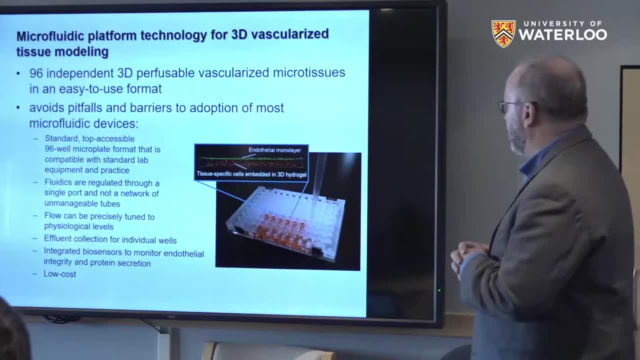 so that they would be disposable, And I think that would also be a key feature to adoption. So this is where we have a lot of effort and kind of interested in commercializing this and have some discussions to move that in that direction, And I think this is exciting for us. 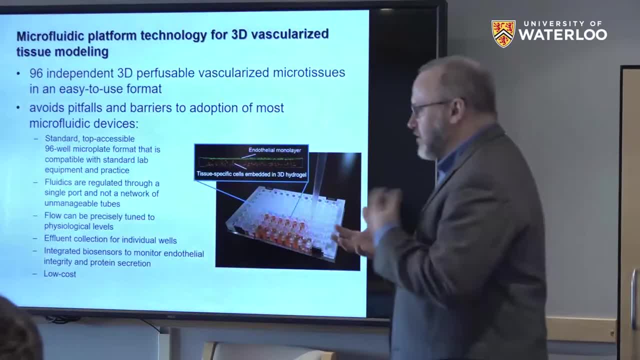 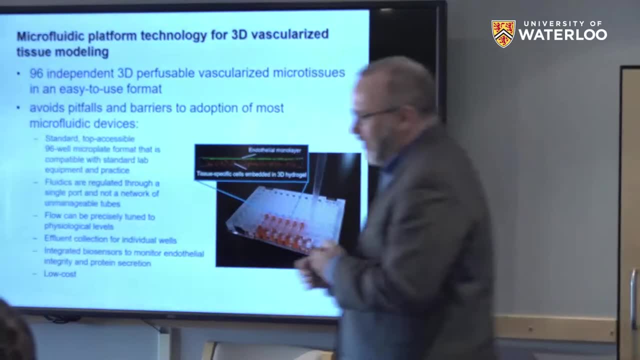 And there's a lot of interest from the farmer partners we talked to. because of the potential And part of this whole process of commercialization, we have to demonstrate that potential And so that's what we're working on right now. We're looking at using the system to model liver. 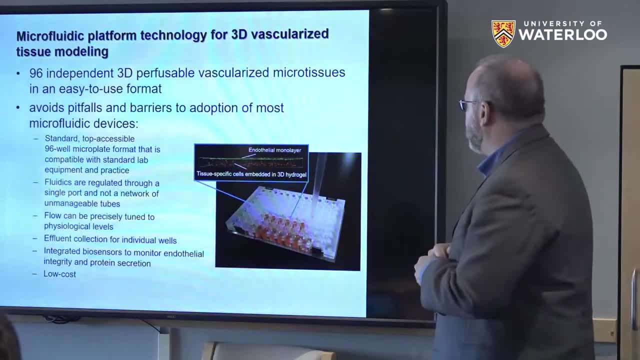 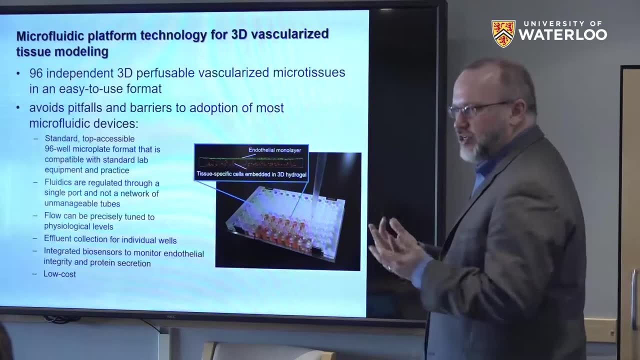 blood-brain barrier and cardiac are the three target tissues that we're working on. These are all of big interest to the pharma industry and I think are well-suited. They're all vascularized tissues. The vasculature plays an important role. 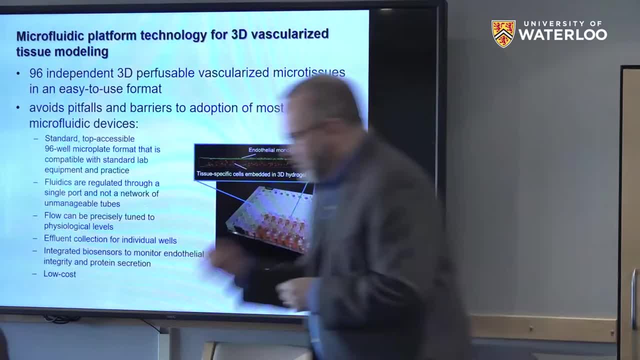 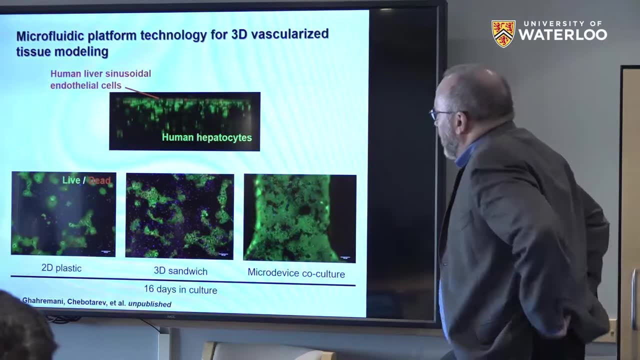 in all of those tissues, and so we think this is well-suited. And just as a kind of a proof of concept or proof of principle that this might matter, here's some early data from our liver testing. So, with the liver model, 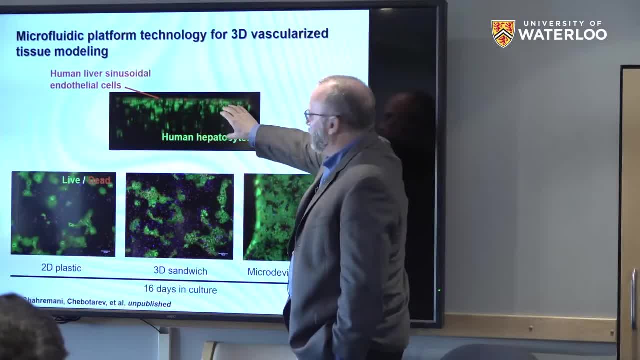 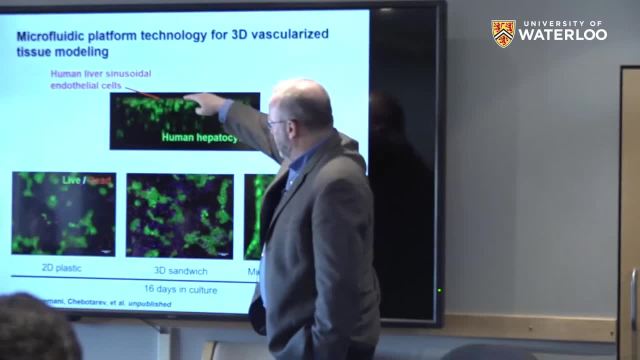 we put liver hepatocytes in the bottom chamber, They're embedded in a 3D biomaterial And then we have liver human and these are all human. so these are all primary cells, liver endothelial cells on the top. And if we grow these, 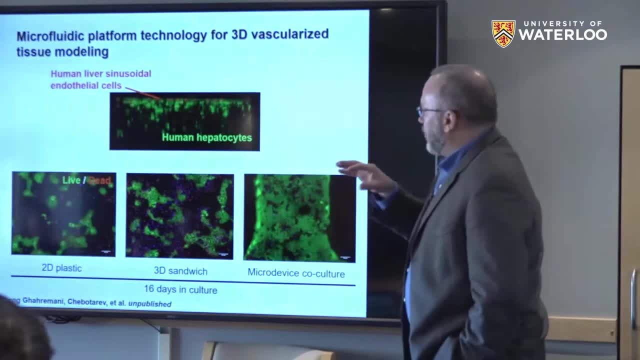 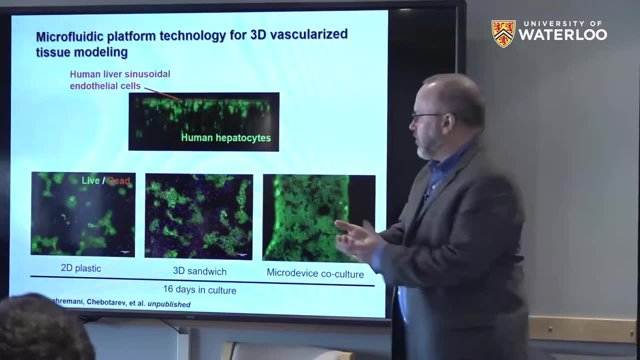 this is under static, so we haven't even introduced the flow in this case. But part of the problem right now with liver modeling is that the hepatocytes don't live very long in culture. If you grow them on a plastic plate, they die within three to five days. 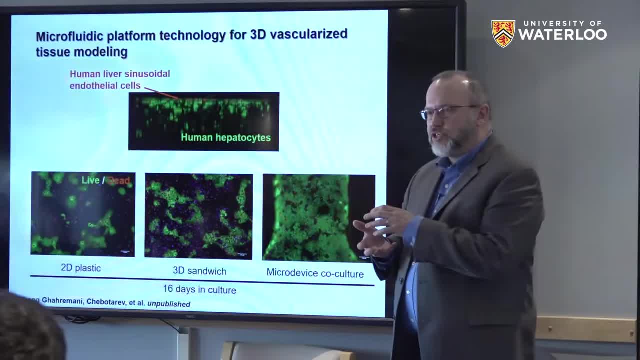 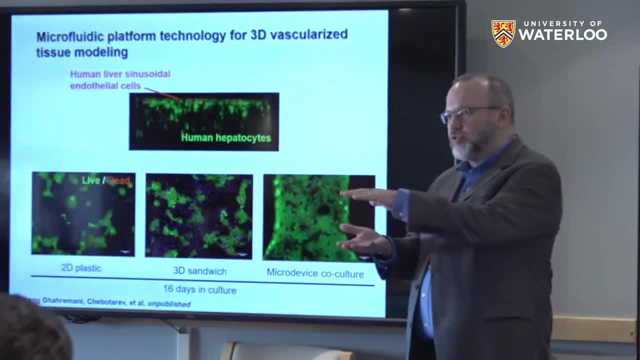 The current gold standard model is called a sandwich culture. So you put down some collagen, you put the hepatocytes on the collagen, and then you overlay it with another biomaterial, matrigel, And so they're in kind of a 3D arrangement. They last a little longer- five to seven days, but they can't go beyond that- And pharma companies? the problem is that if you have a drug that's slowly metabolized, that's what the hepatocytes do: they metabolize drugs. 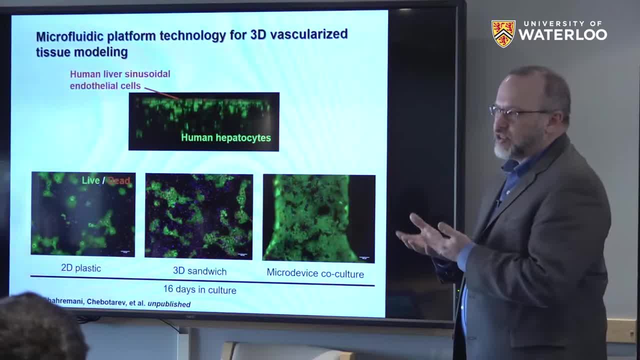 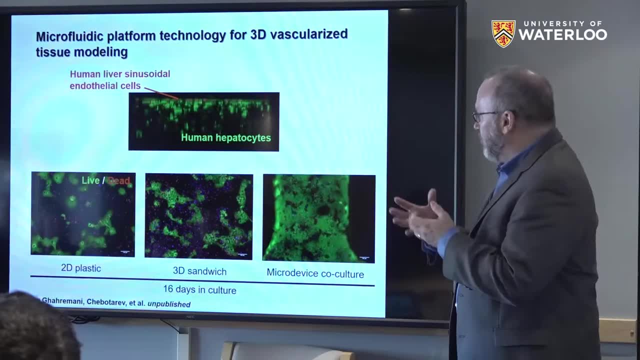 If the drug's slowly metabolized, they don't have an in vitro system to study those drugs because none of their in vitro systems live long enough. So at minimum, if we could get these hepatocytes to live longer, that would be an advance. 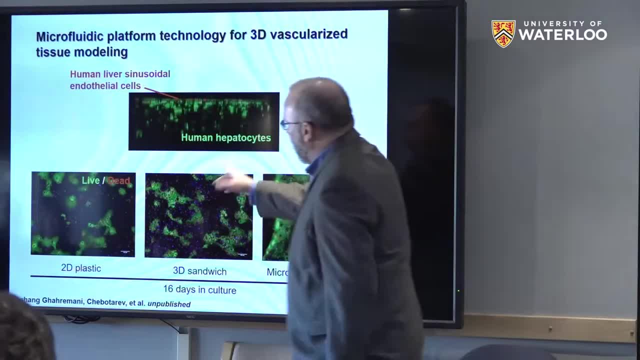 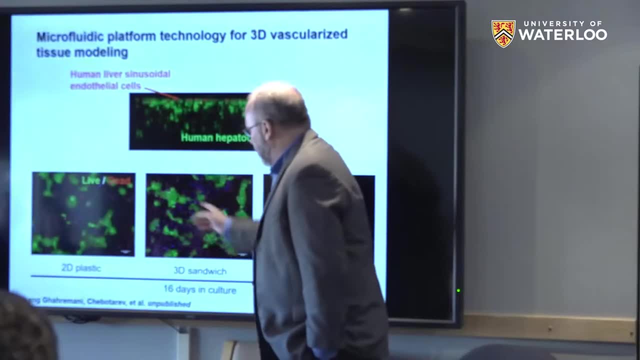 And this is what our initial data is showing. So this is a live dead stain. So live cells are green and dead are red. And we have three conditions: plastic dishes, the current gold standard, 3D sandwich culture and then our microfluidic device. 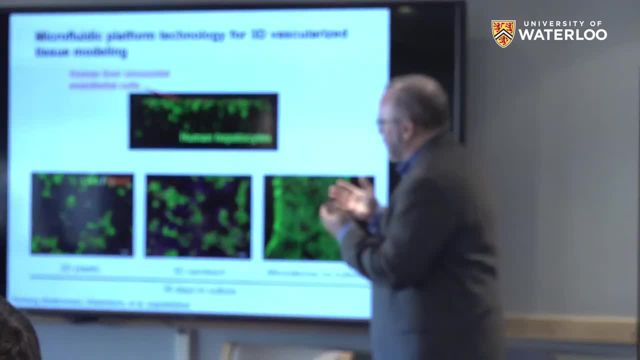 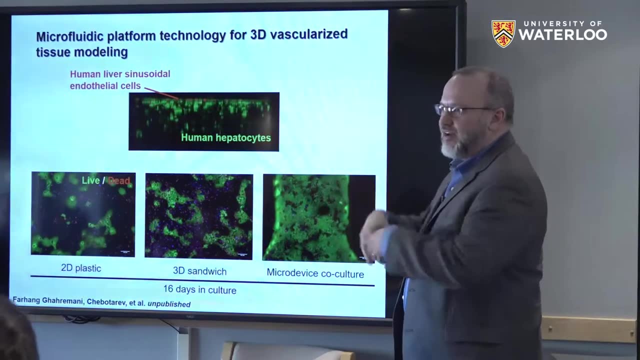 where we have the endothelium, in the hepatocytes, And I think you can see just qualitatively that in the 2D plastic there's lots of red cells. There's actually lots of cells that are gone, They've died and come off the plate. 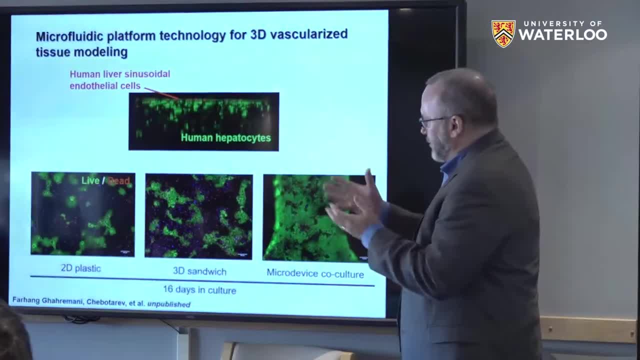 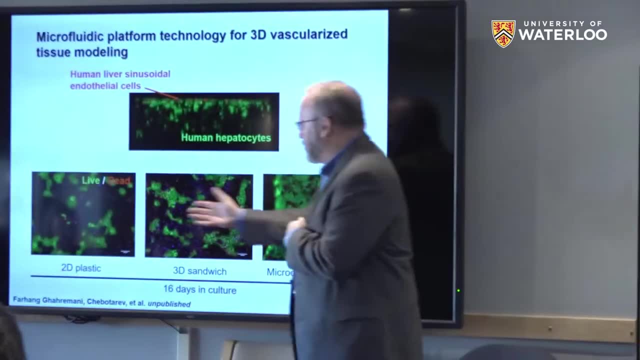 There's fewer cells there, And this is after 16 days in culture, so much longer than what people are able to normally culture hepatocytes for, And that's what we see In 2D plates. they just don't live Even in 3D culture. 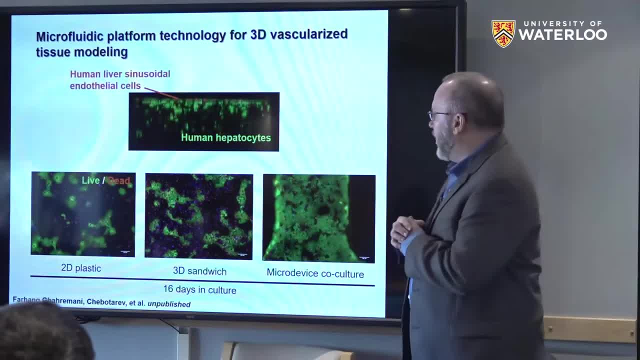 you can see, we still have some viable cells, but many, many dead cells in red there, Whereas in our microfluidic co-culture, where we now have the endothelium, you can see lots of viability in the hepatocytes. So I think this is really encouraging. 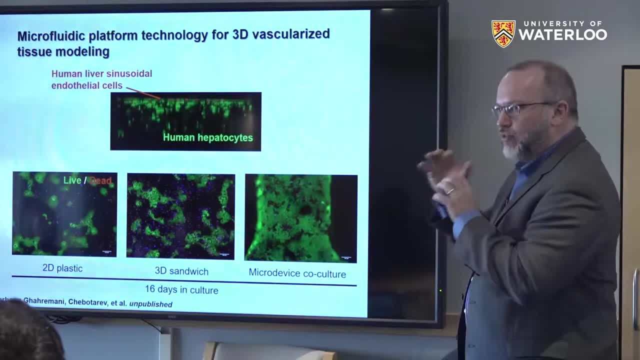 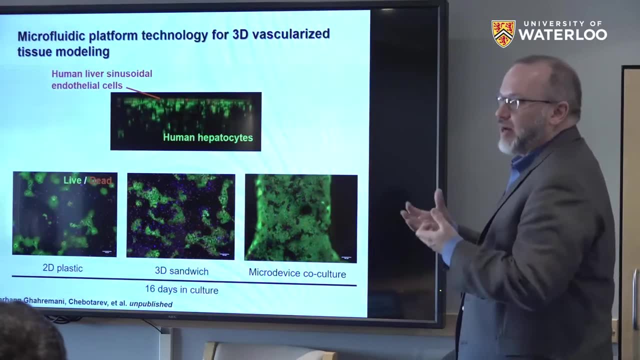 that we're able to. even just by co-culturing, without flow, we can get the cells, the hepatocytes, to live longer, presumably because the endothelium are secreting things that are keeping the hepatocytes alive. And now you set up the ability. 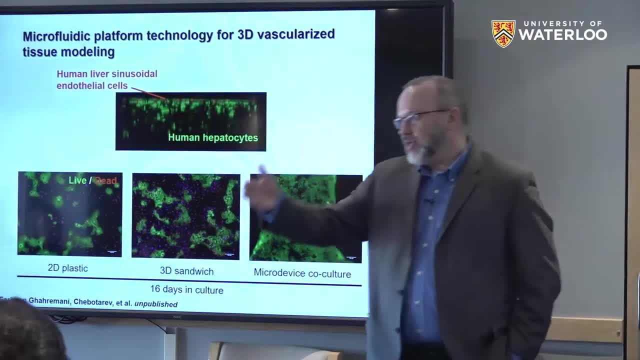 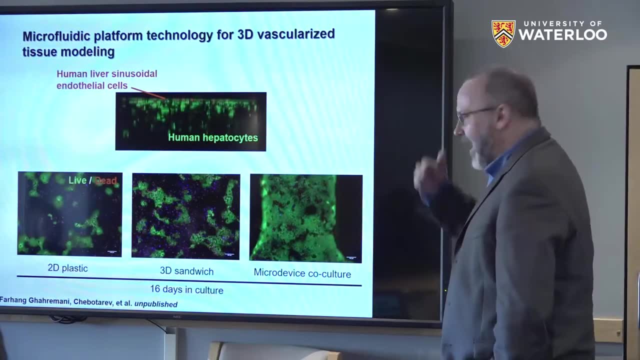 to do 16 or maybe even longer cultures to look at slowly metabolizing drugs, And so this, I think, is a nice demonstration. We're now adding flow to that and then demonstrating that if we put in these slow metabolizing drugs, do we actually see things in this system? 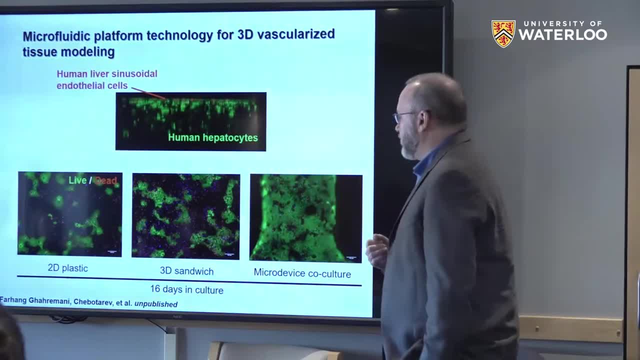 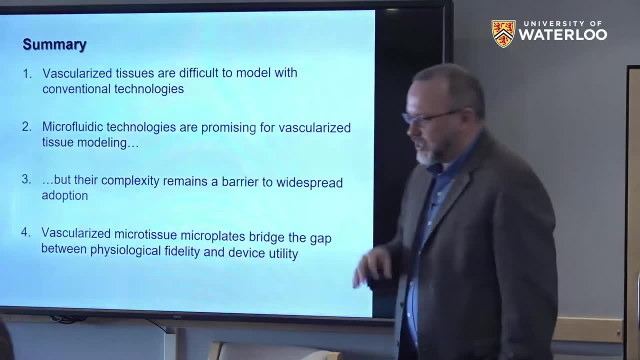 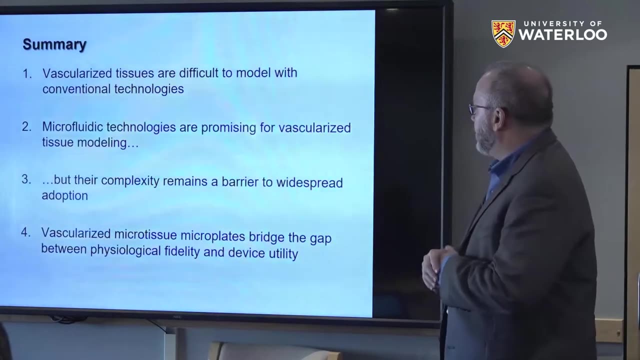 that we'd expect in the body. So we're continuing to do validation there and just one type of application. So just to summarize that section, kind of take-home messages, our vascularized tissues are difficult to model with conventional technologies- dishes, basically. 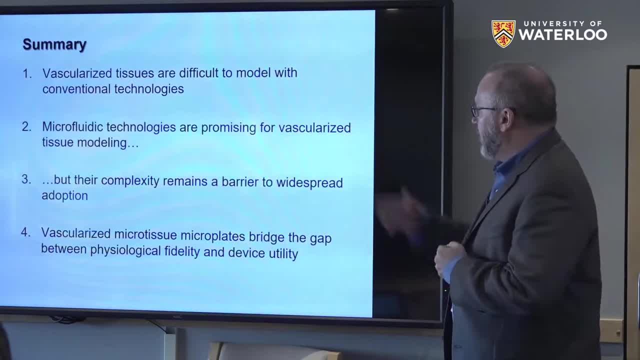 Microfluidic technologies are promising for these applications. but point number three: there complexity remains a barrier for widespread adoption And you really don't see a lot of good examples of microfluidic devices that are kind of off-the-shelf usable by a biologist. 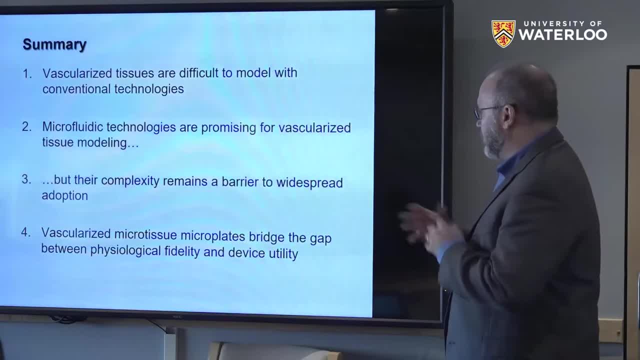 And we think that this microplate and this approach may help bridge the gap between physiological fidelity. So we sacrifice maybe some physiological fidelity, but we have a device that's useful and can be actually used. So we think this is a nice compromise and something that could be readily adopted. 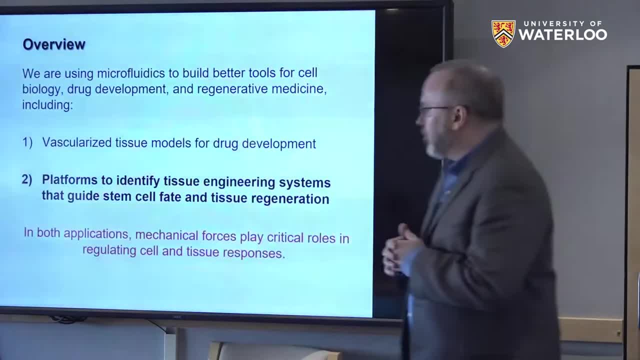 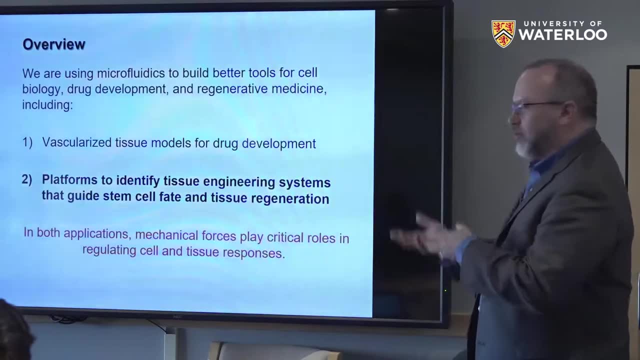 Okay, So that's part one And the second part. I just want to talk about some of our platforms where, again, we've used a microfluidic approach, but for a very different application. In this case, we're interested in. 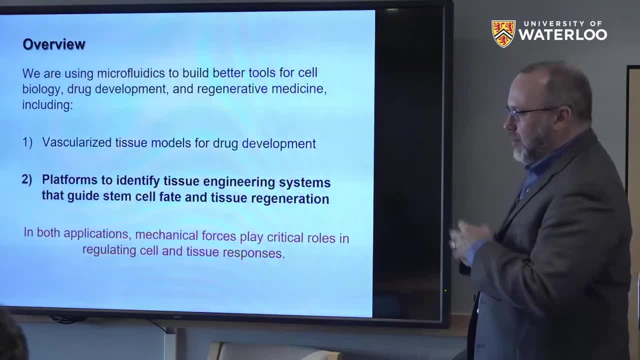 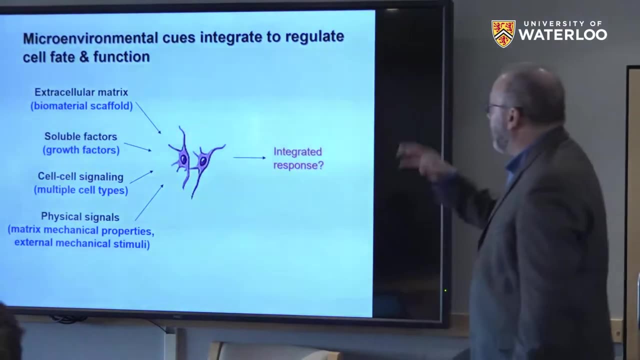 can we identify microenvironmental factors, things like biomaterial factors and mechanical factors that can regulate stem cell fate and ultimately tissue regeneration? And so again, we're interested particularly in mechanics, And if you think of all the cues that a stem cell might see, 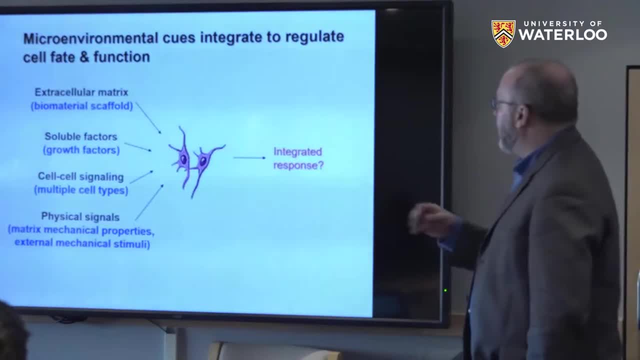 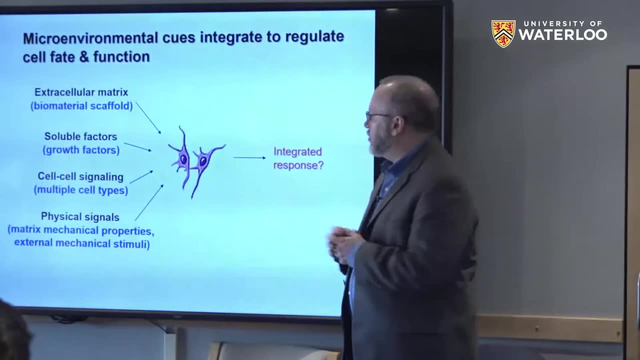 in its environment, either an engineered environment or a native environment. it receives cues from the material it's in or on. It receives soluble cues in its environment. There's other cell types often signaling to it, but it'll also see physical signals. 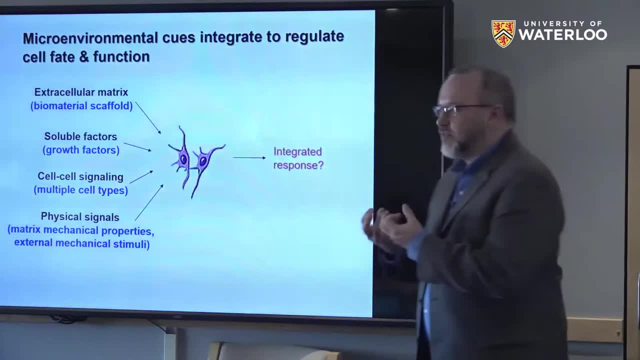 things like the physical stiffness of the material it's in or on, or external mechanical stimuli, a stretch, for example. And the question we're interested in is: how do these factors, how do these factors integrate? Because the cells respond to each of these factors independently. 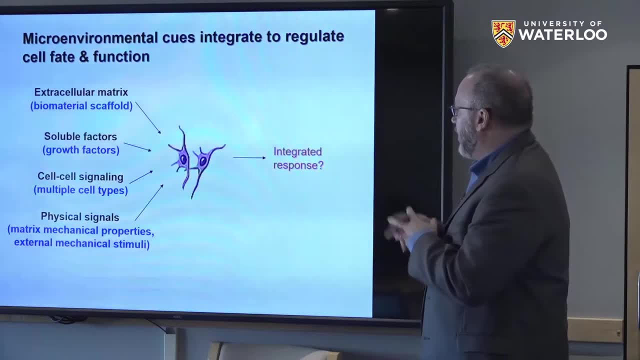 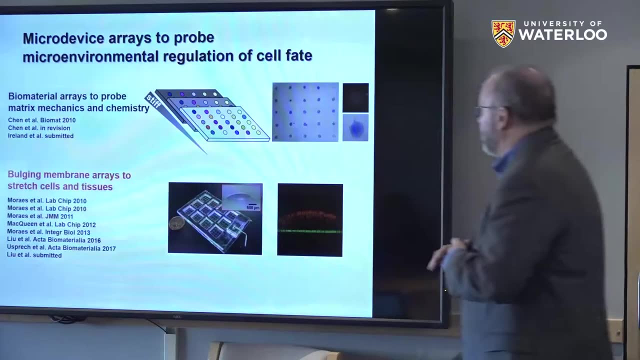 but may respond to them in some complex, integrated manner. And when you start combining these many factors, what is the integrated response? And so we've been developing a whole bunch of technologies to allow us to study this And, again, fairly simple type approaches. 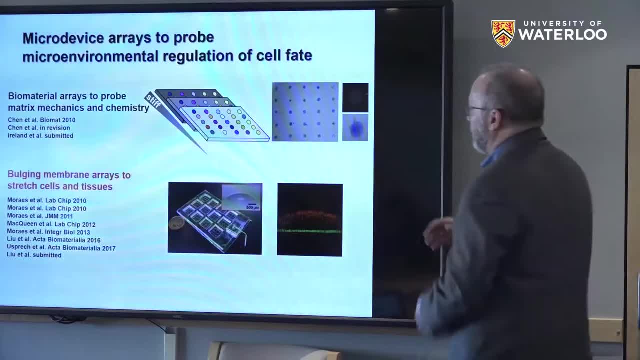 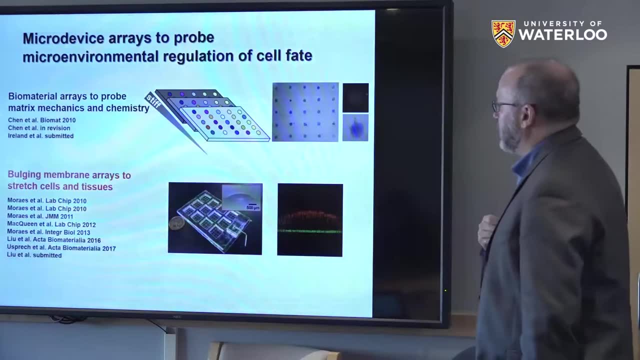 but basically arrays that allow us to study how biomaterial properties influence cell function and then how mechanical factors influence cell function and stem cell function. So we're going to talk about the last group primarily and talk a little bit about our early work. I guess Chris Marais was here. 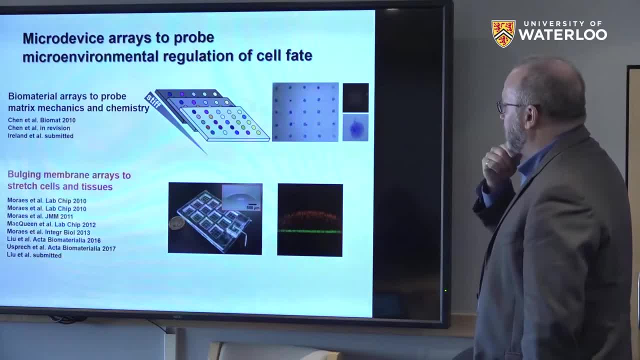 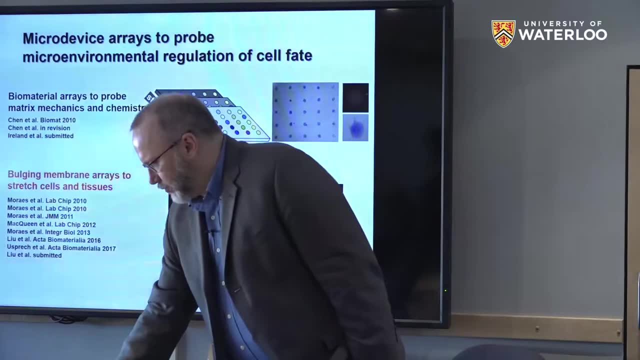 maybe a couple of months ago, He was a PhD student in my lab, and so he started us working in this area. I'll talk a little bit about his work and then our more recent work, And so I'll get motivated by a problem that we're interested in. 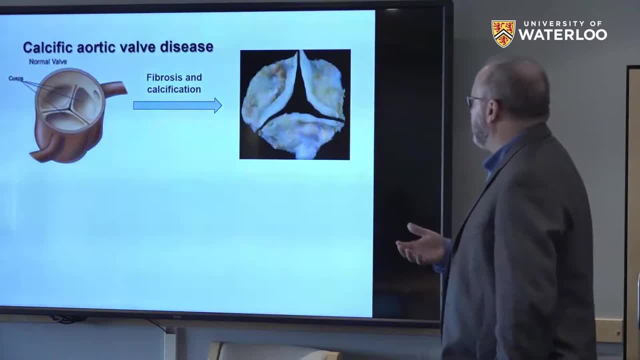 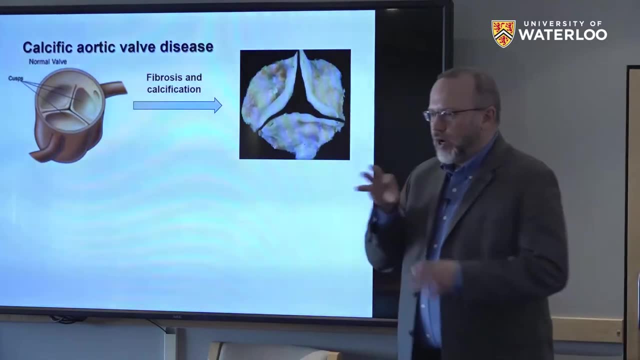 again is then: why do these heart valves become diseased and fibrose? So there's the normal heart valve and then, as they calcify and fibrose, they look like this, And so we're interested in: how does mechanics and other environmental factors? 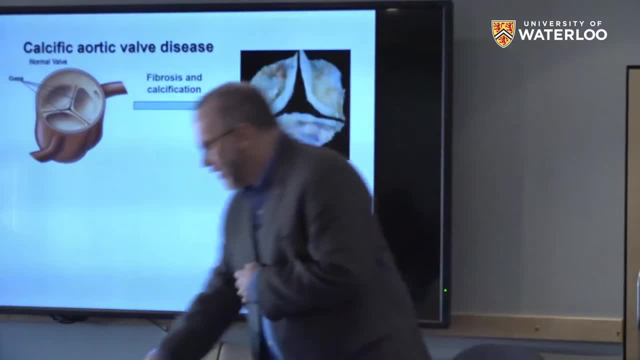 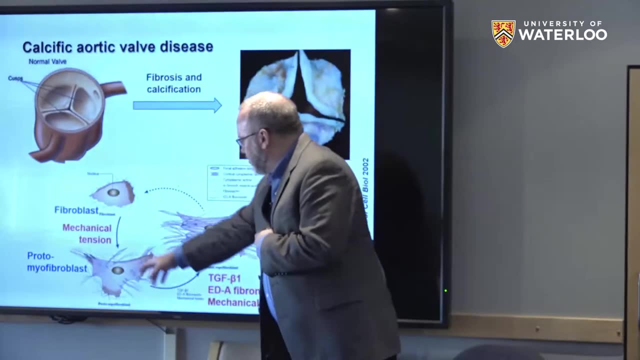 feed into causing that scarring or that fibrosis. And what's known is that fibroblasts, which is the normal cell within a heart valve, one of the factors that causes it to become a myofibroblast, which are these cells. that make the lots of collagen and cause the scarring is mechanical tension's important, But not only mechanical tension. you also typically need a growth factor like transforming growth factor, beta-1, and you need an extracellular matrix protein like EDA fibronectin. 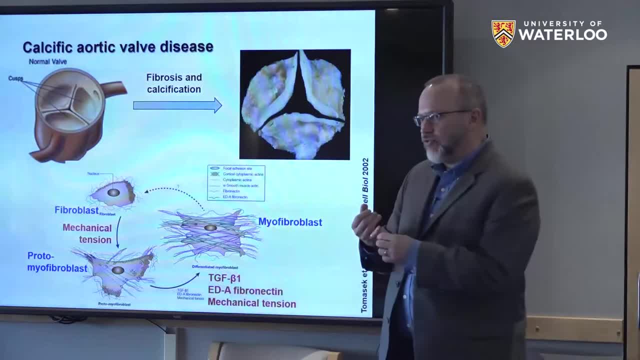 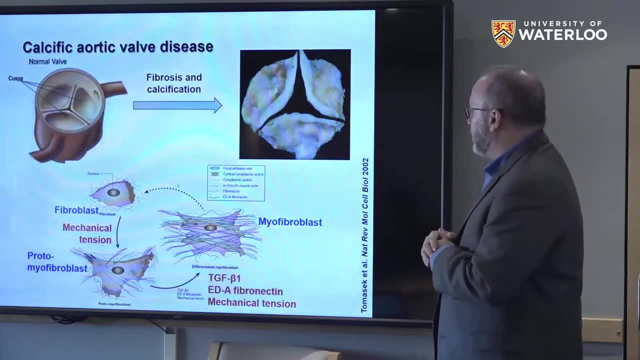 And so here you can see, there's multiple stimuli: a growth factor, biomaterial or matrix factor and a mechanical factor that are all contributing to this differentiation. And so we were interested in how do valve cells, valve fibroblasts, respond to these combinations of factors? 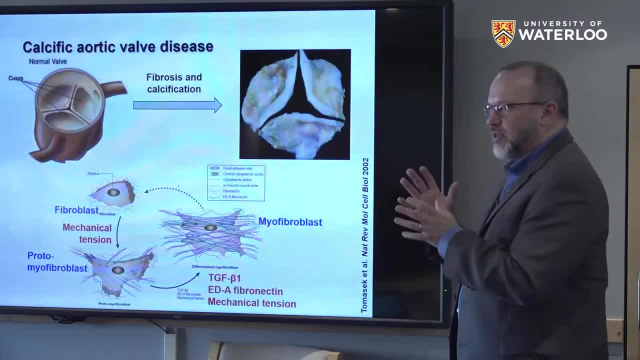 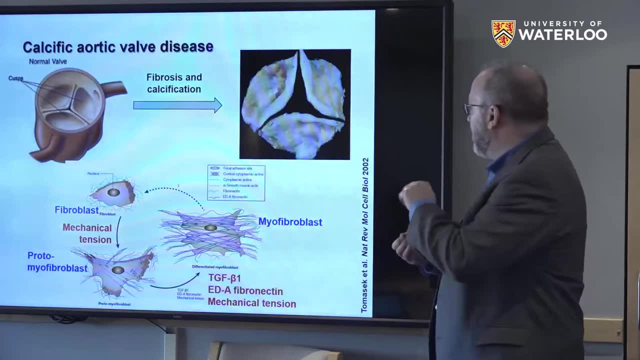 And in this case we're particularly interested in the side-dependent, the thing that I told you about. Remember I said: cells from one side of the valve become calcified and scarred and the other side they're protected. We're asking: 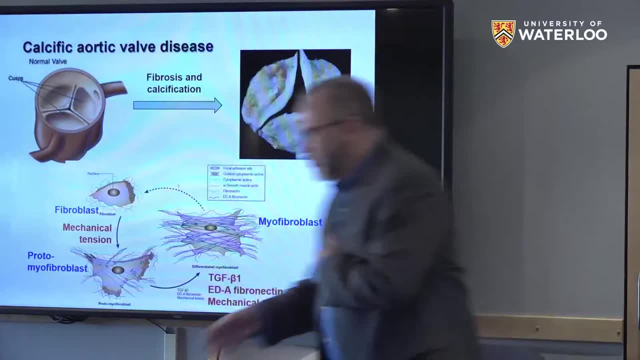 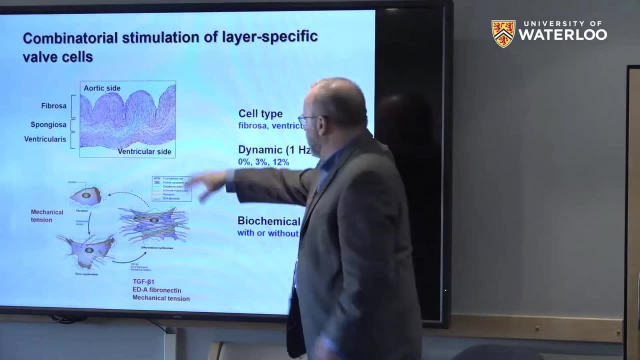 is there a difference in how those cells respond to stretch? And maybe are they. does that explain some of the side dependency? So what we did was we, you know, we knew what some of the factors were involved. We took cells from either the top layer. 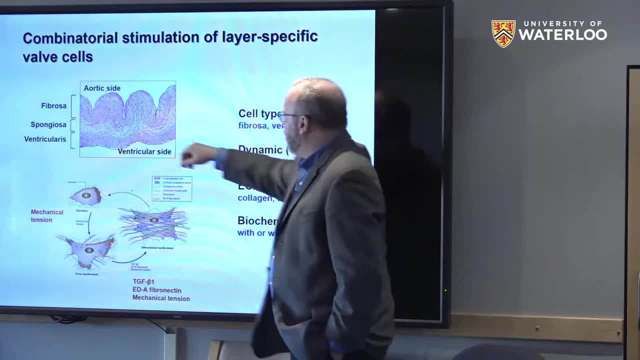 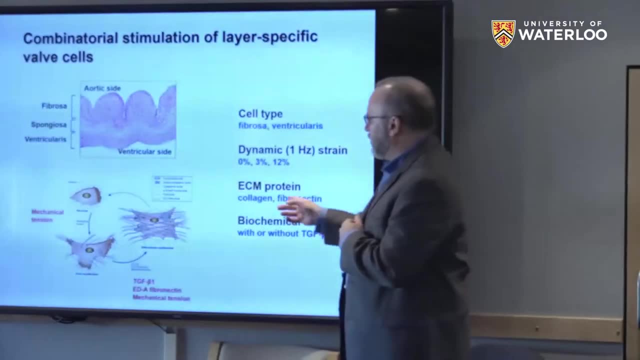 of the valve, called the fibrosa, or the bottom layer, called the ventricularis, and tested them separately. We subjected them to ranges of mechanical strain. We grew them on two different types of extracellular matrix proteins that you find in heart valves. 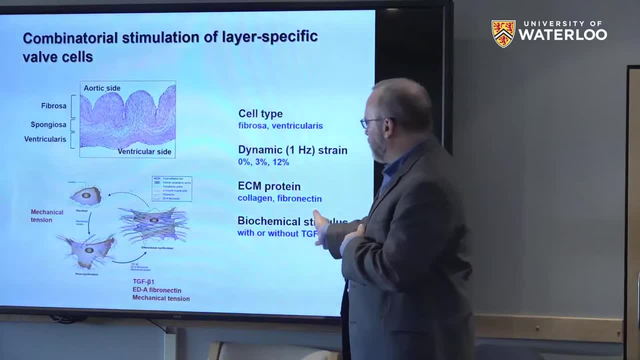 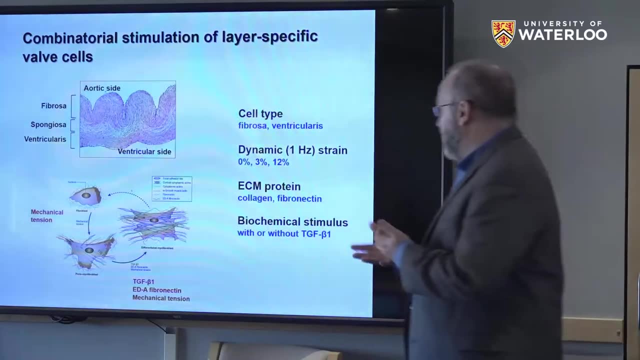 and one that's known to be pro-fibrotic, And we cultured them with or without growth factors. So lots of factors there. I think there's 24 different combinations, And using standard culture methods, these experiments would just they'd be very expensive. 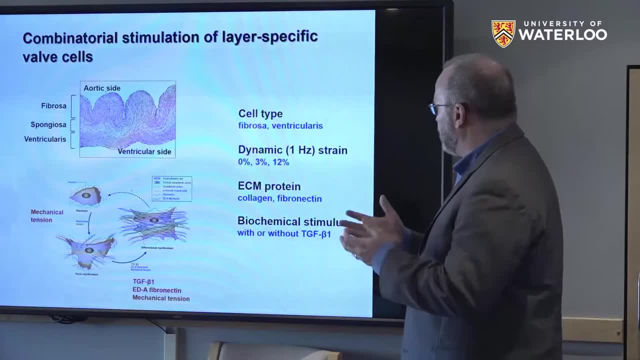 and they would take a long time, Not too expensive because you have a graduate student doing them and graduate students don't get paid that much. But you know, it's just a. it's a challenging problem, right, And if we could speed it up. 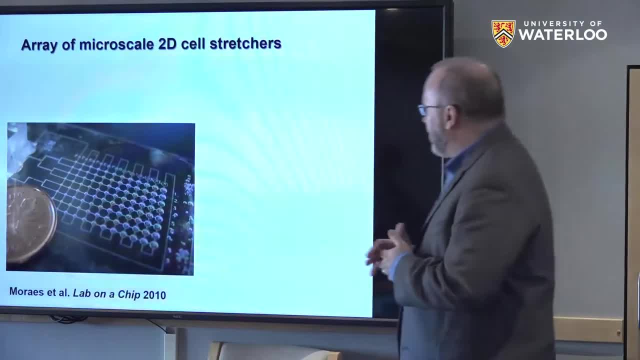 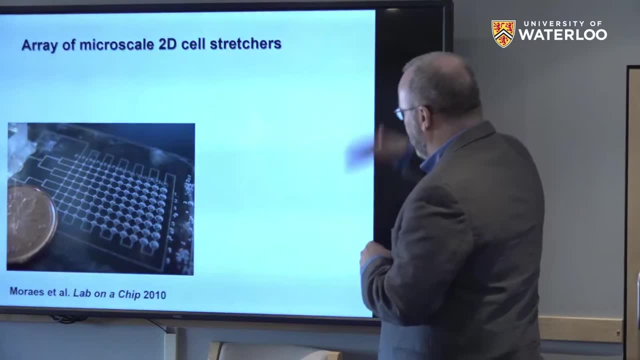 the students would be happier. So Chris Marais, when he was in the lab, again came up with these, these huge arrays of cell stretchers. He kind of went, he shot for the moon and, I think, got there, and then you'll see. 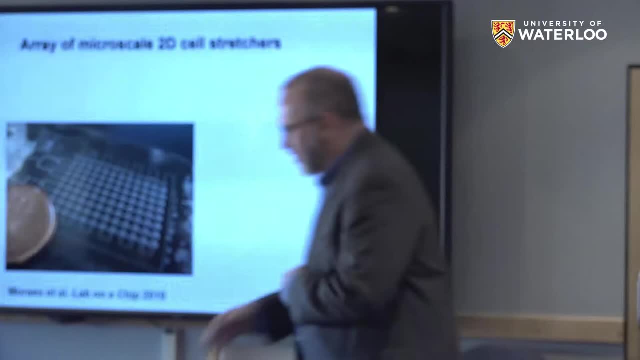 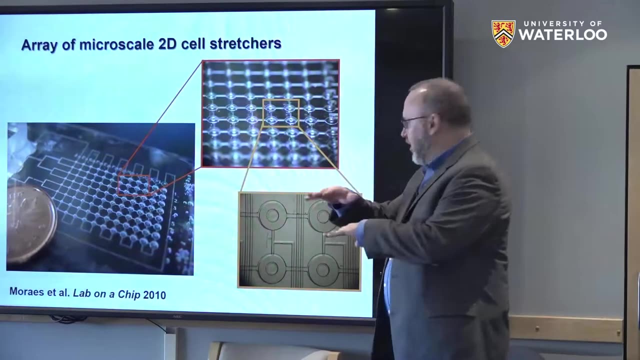 we've backed off since then. But he came up with these array of cell stretchers and you can see, this is these stretchers where basically the idea is there's a post underneath a membrane, and I'll show you that when the post gets pushed up, 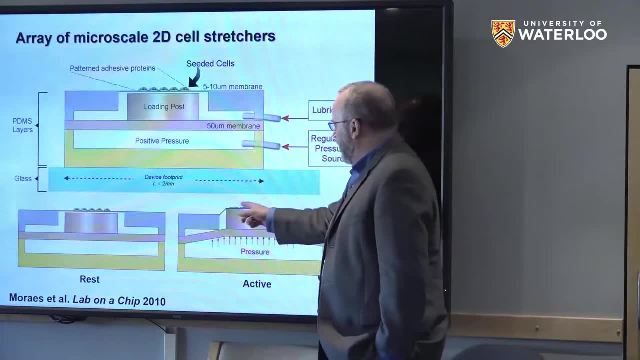 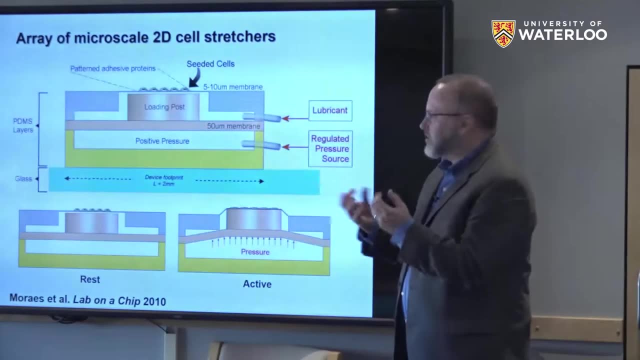 under a pressure it pushes into the membrane and cells that are on the membrane then get stretched. So that's the principle and he had array of these and he had them kind of 96 space like a 96-well plate. 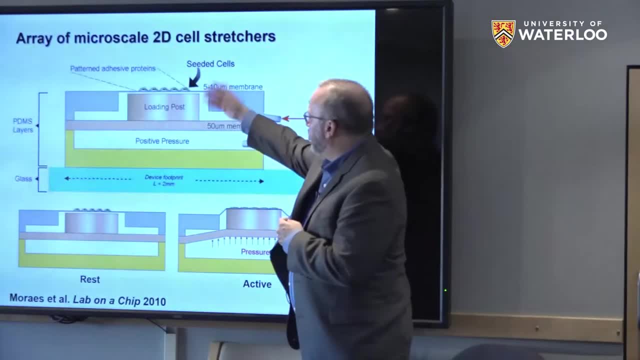 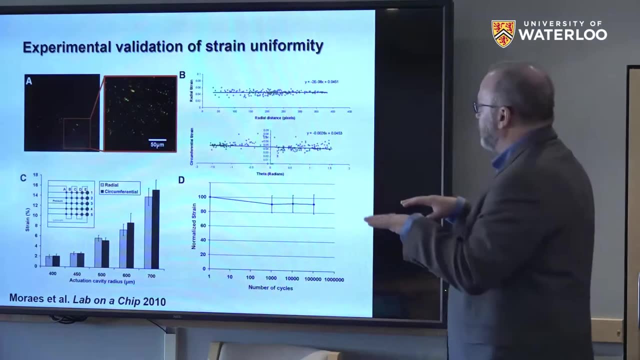 And this was just using air to push up the loading posts into the membranes. So that was the principle and he went on to show that he could get really nice uniform strains, equibioxal strains, over these culture areas and that the 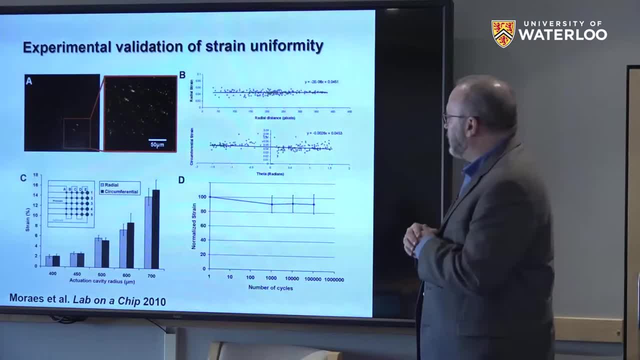 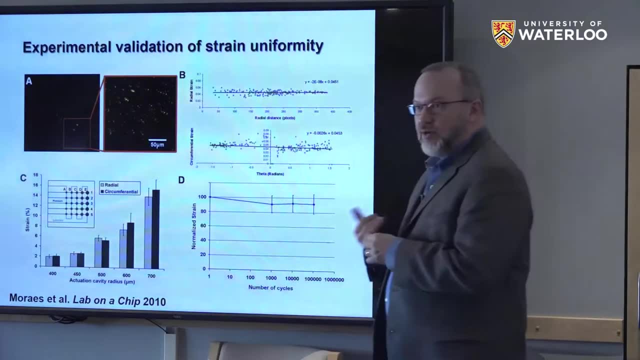 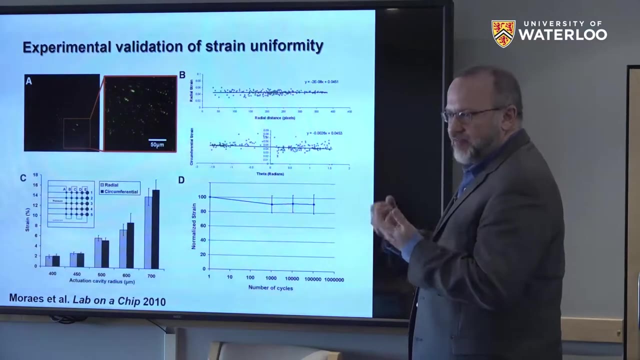 you know that we can maintain the strain over hundreds of thousands of cycles, So nice system. The challenge with it was it was a real challenge to make. one Fabrication was really difficult and the success rate of the fabrication was pretty low. 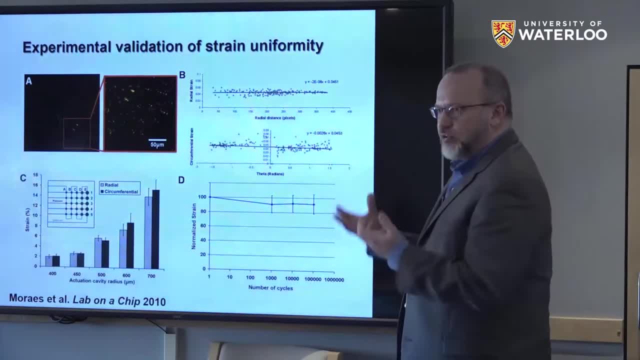 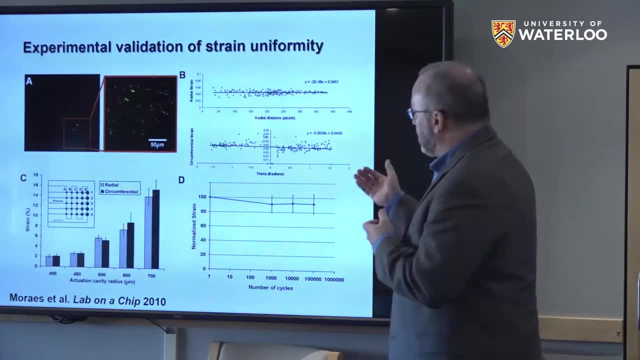 And so, in terms of wanting to use this to actually do experiments, you'd spend a lot of time making devices and you wouldn't have as much time to do experiments. So you know, I think it was. it's a nice and very elegant. 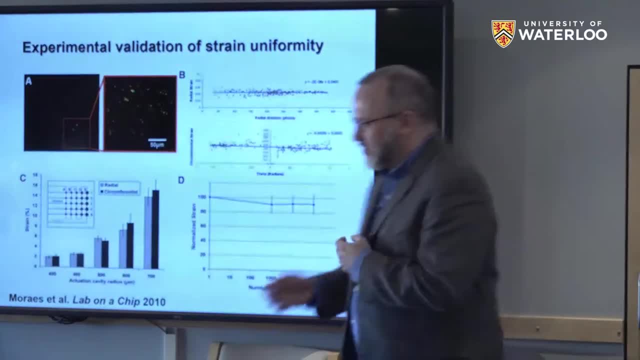 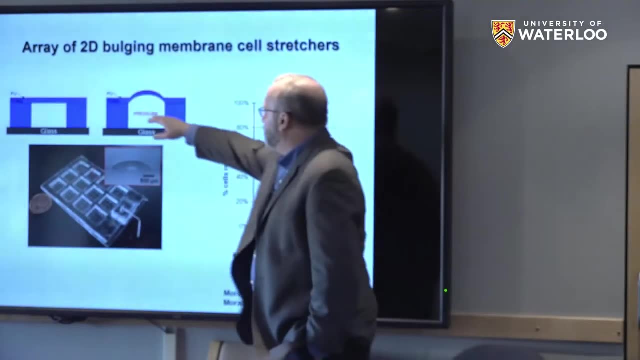 solution Chris came up with, but in the end we decided to back off and come up with a much simpler system where we remove the post and, instead of pushing up with a post, we just bulge a membrane by applying pressure under it. 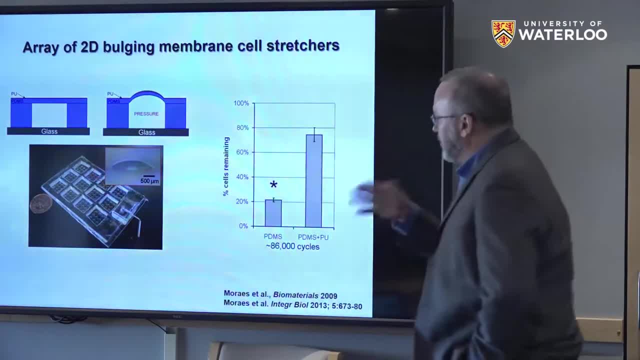 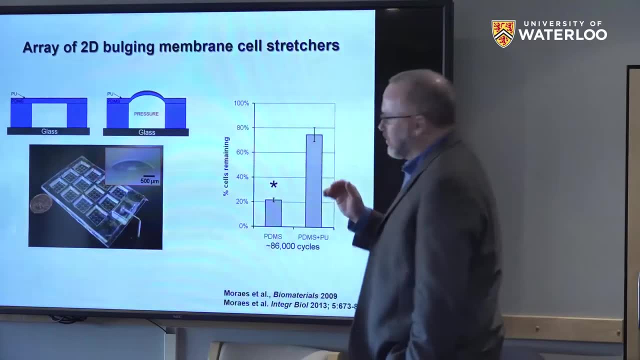 So the this is much easier to make. bulging membrane systems. We can do some material modifications to make the cells more adhesive to them, but the downside of these, or the disadvantage of these, is you don't get a uniform strain. 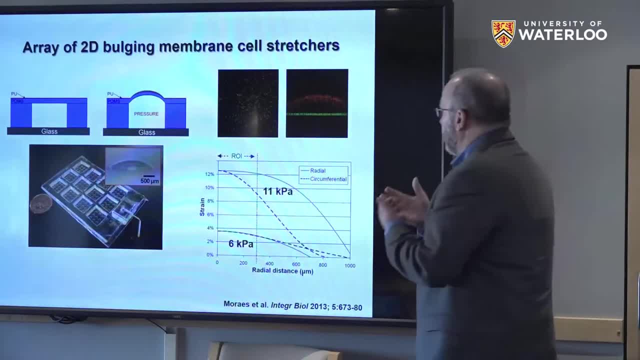 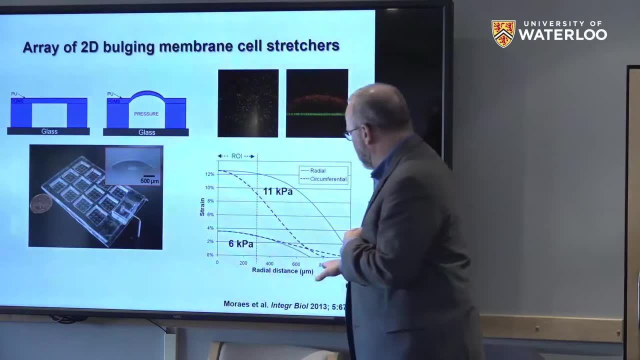 over the whole membrane now because it's bulging up. So we recognize that we allow for that, and what we did was we. this is what the structure is. this is what the. this is the distance from the center of the bulging membrane. 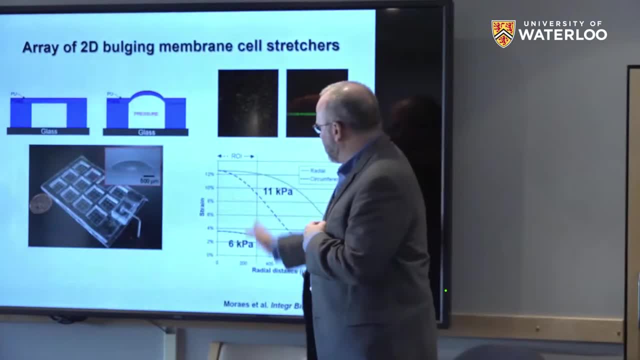 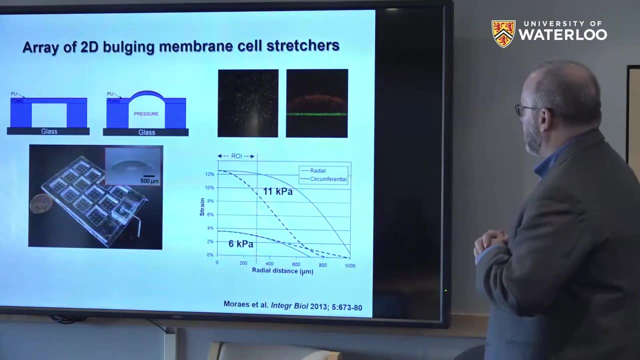 to the periphery, and this is the strain profile. We confine our analysis to this middle range, where the strains are approximately constant, Not quite, of course, but good enough, I think, for our purposes, And this is in contrast to the previous system. 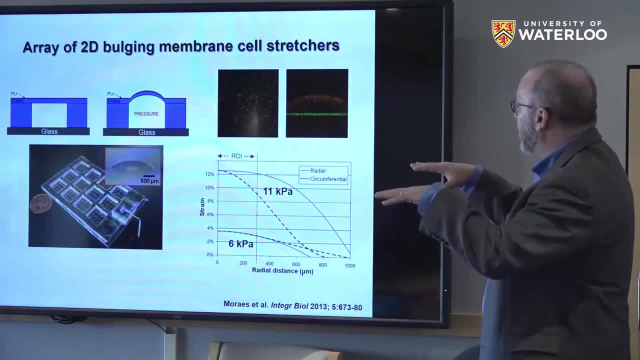 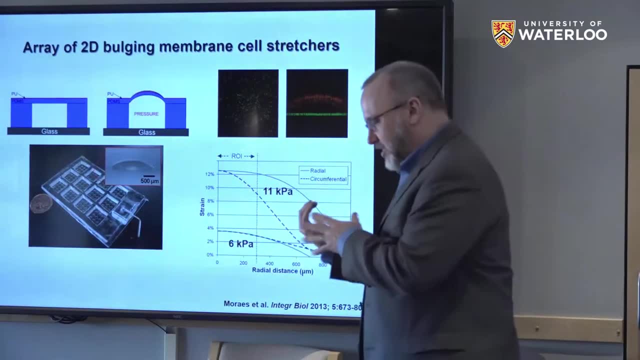 where we had nice uniform strain across the whole, the whole membrane. but again it was just not feasible to make, at least using the fabrication methods we were using. So Chris then used this system, looked at how this system works, how the cells respond. 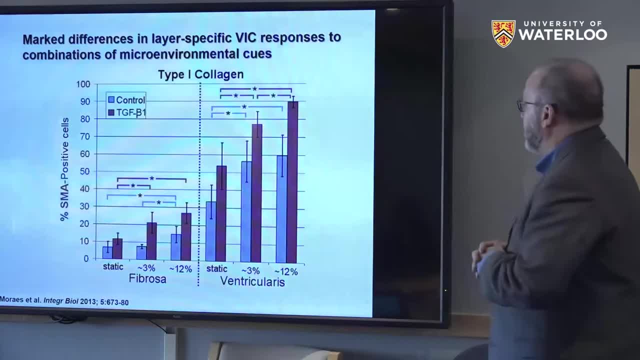 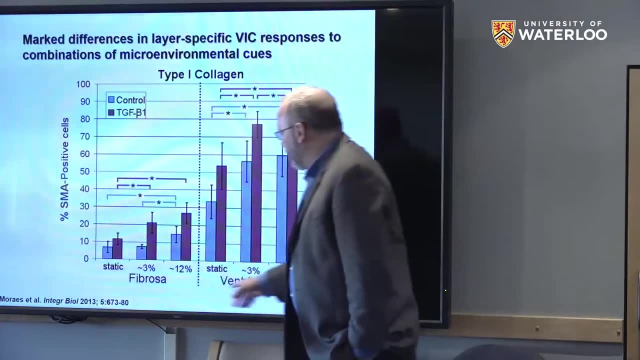 to many combinations of factors and you get, you know, so you get some really rich data sets coming out of this. This, for example, is showing if you grow the cells on collagen from the fibrosis side of the valve or the ventricularis. 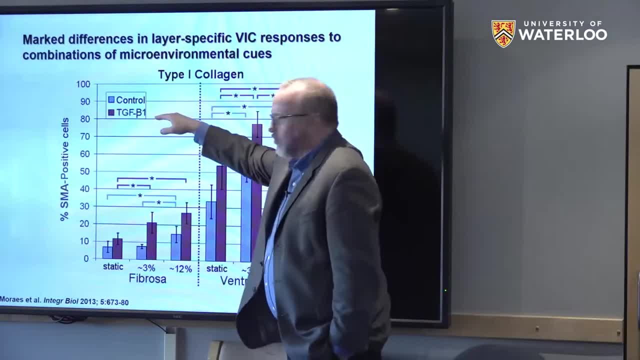 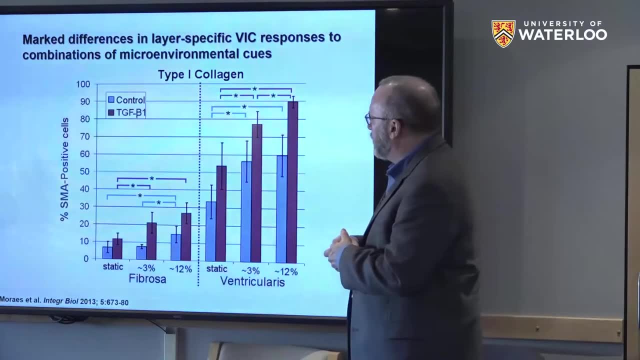 side of the valve at different levels of strain, with and without the growth factor. So all those factors are now incorporated and he was able to do this on a single chip, this experiment on a single chip, and then repeat it at least three times. 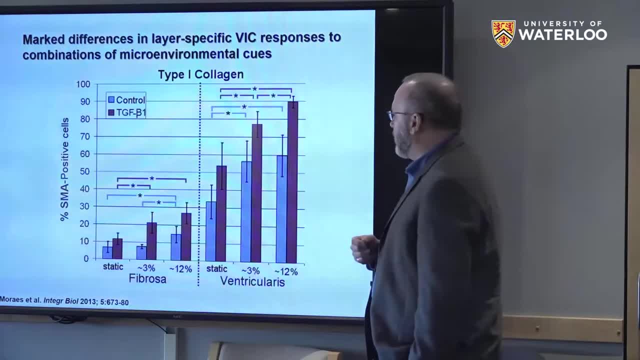 And then he measured what fraction of the cells express this marker in the mouth with smooth muscle actin And you get some interesting results coming out. One: you see: the ventricularis cells- these are the cells on the bottom layer- seem to be much more sensitive. 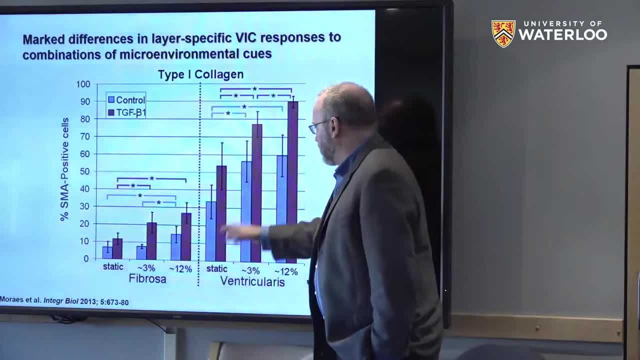 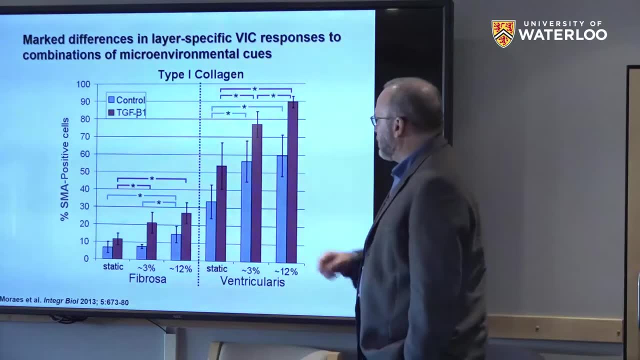 to the strain right. Well, much more sensitive period, much more likely to become myofibrogenic under collagen and much more sensitive to the strain than the fibrosis-level cells and, perhaps you know, equivalently sensitive to the TGF-beta. 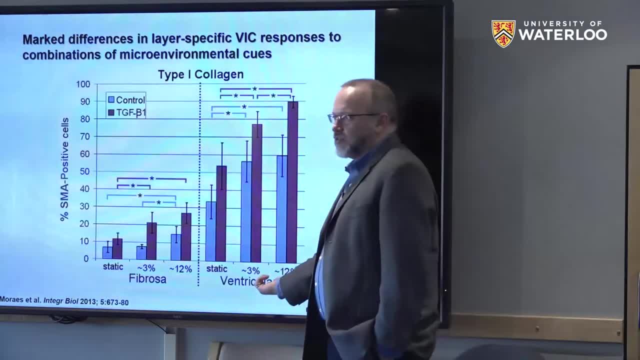 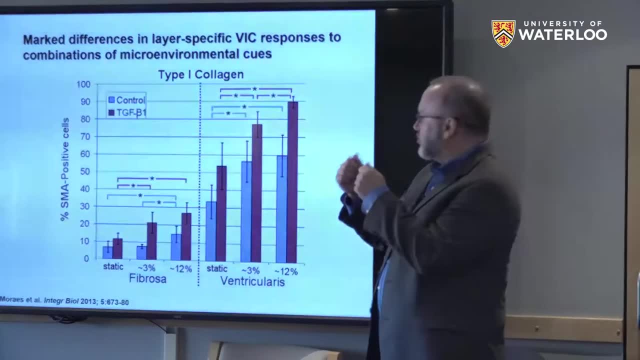 This was a little surprising to us, because these are the cells that don't scar, These are the cells that are in the protected layer. but these cells, in vivo, also don't see the high strains, the same strains that the fibrosis-layer cells do. 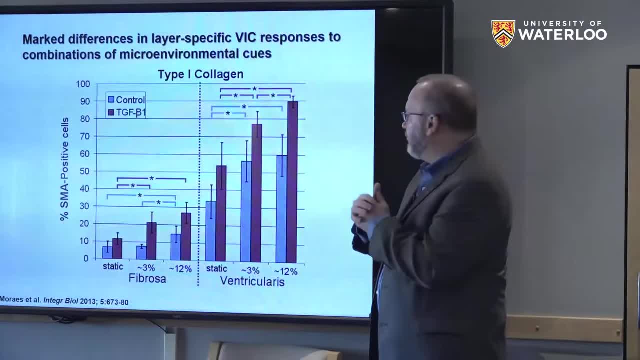 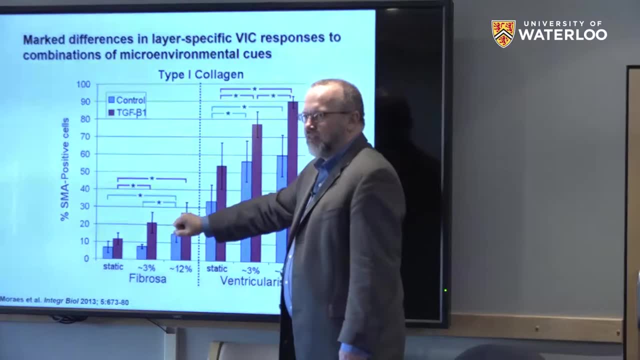 The fibrosis-layer cells are under higher strain just within the heart valve and it's possible that they've adopted or adapted to that high-strain environment and therefore a little more desensitized when we pull them out of the valve, Whereas these cells 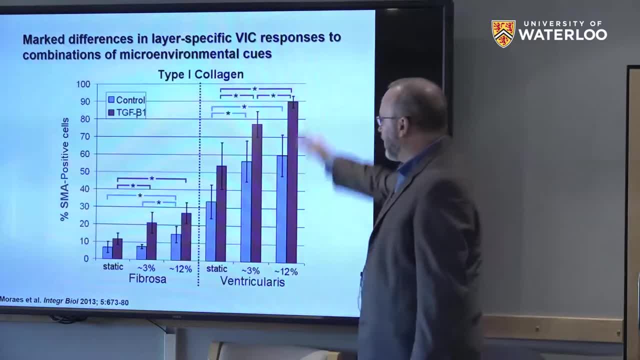 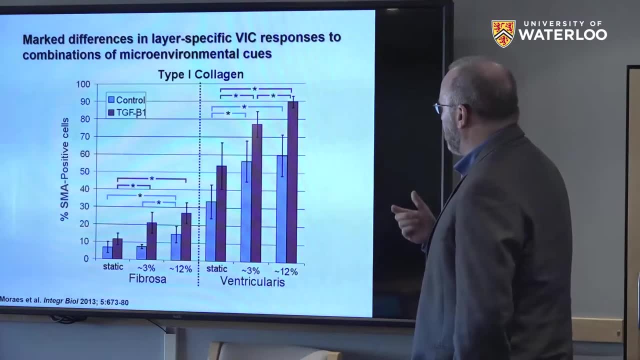 see a less-strain environment, and if you now just really start pulling on them, they get hyperactive. So that was interesting, that we saw a side dependency that had never been considered before or reported before, And then on top of that we saw a dependency. 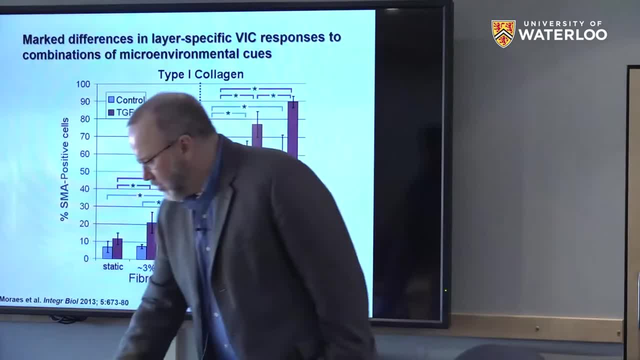 on the type of protein that they were sitting on. So this is on collagen, but you can see, if we put them on fibronectin, everything is turned up. The cells, all many more of the cells, become myofibergenic. 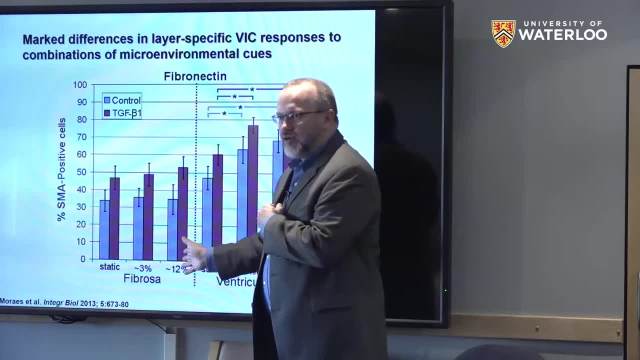 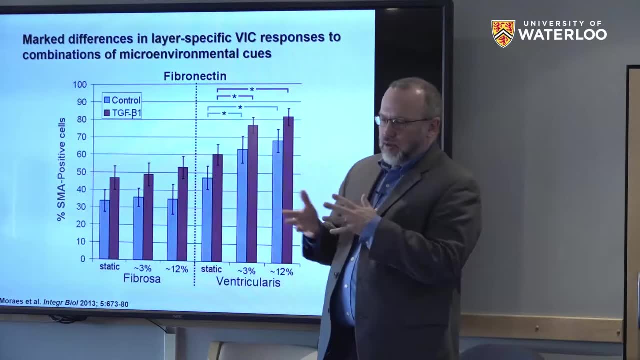 You can see, under the fibrosis they become insensitive to the strain under this condition- Not clear why- And they become less sensitive to the strain under this condition. So we don't understand why this is or why there's these differences or differential responses. 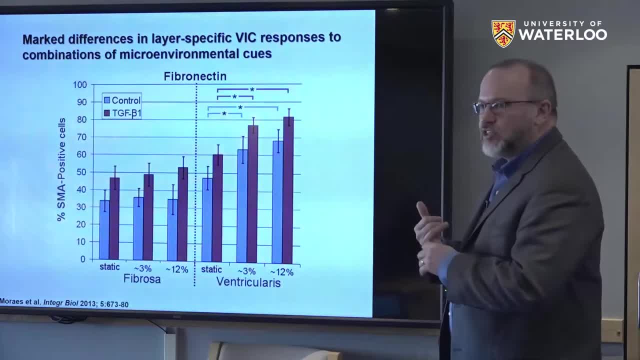 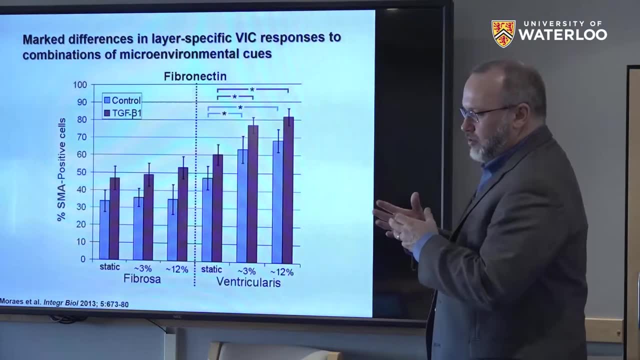 but it does demonstrate that a lot of these factors do matter. The protein you're sitting on matters, the mechanics matter and the soluble environment matters. So the so I think that was confirmation that this type of approach is interesting and that these multiple factors 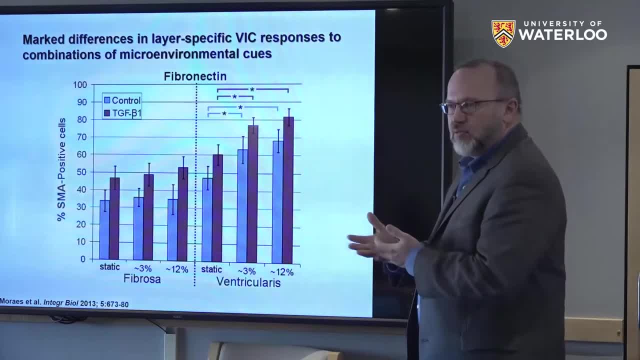 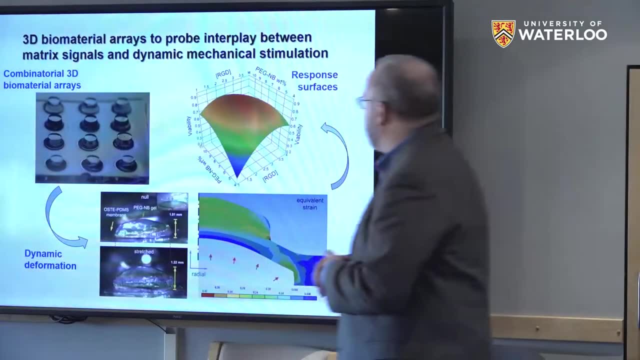 do combine in interesting ways. But this was a 2D system and most of the tissues we work with are three-dimensional tissues, and so now we've taken this approach and moved it to a 3D system. So, again, we use arrays. 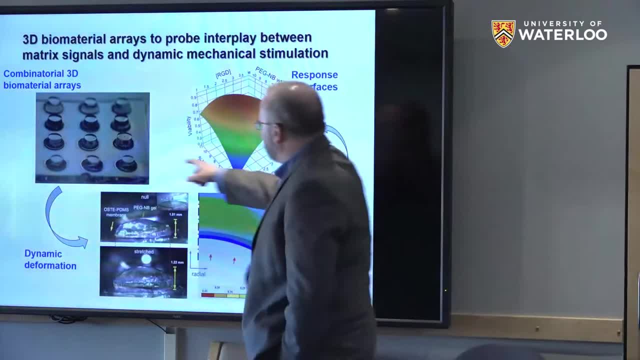 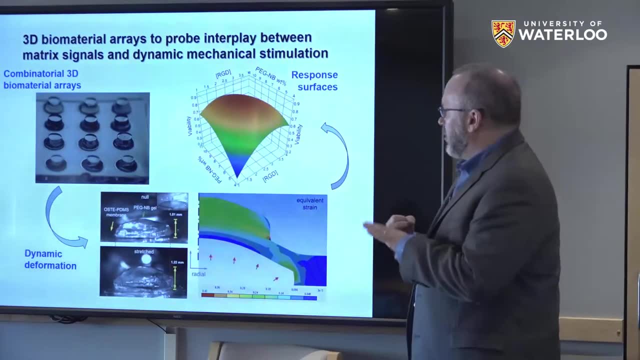 in this case a biomaterial arrays in each one of these little cylinders. we can change the composition of the material, the porosity of the material. we can change the peptides, the adhesion peptides, or the proteins that the cells can adhere to, in many different ways. 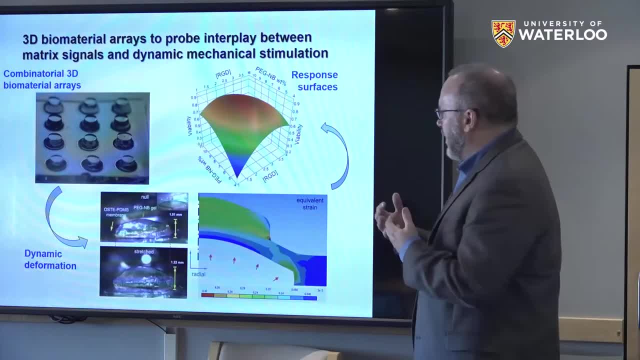 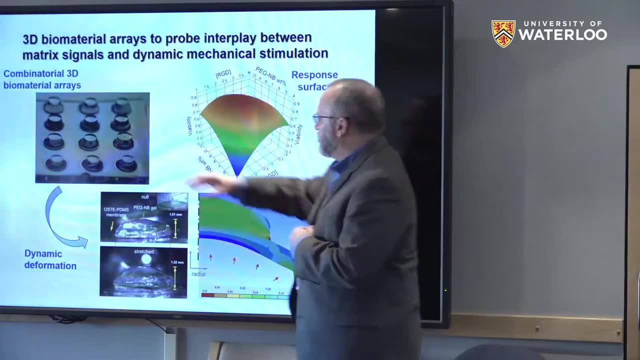 and put in many different mixtures, and then, on top of that, we've engineered systems that allow us now to stretch these gels and apply dynamic mechanical stimulation. So there's a lot of work in this area, but no one's been able to figure out. 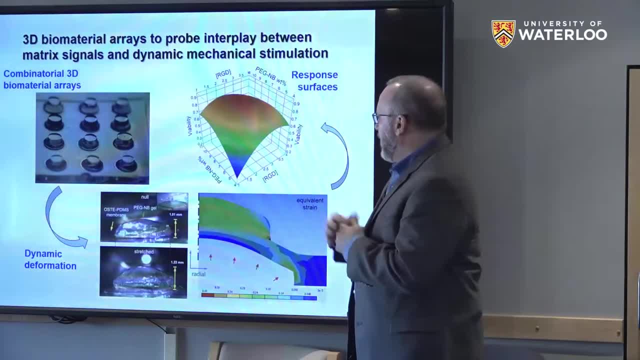 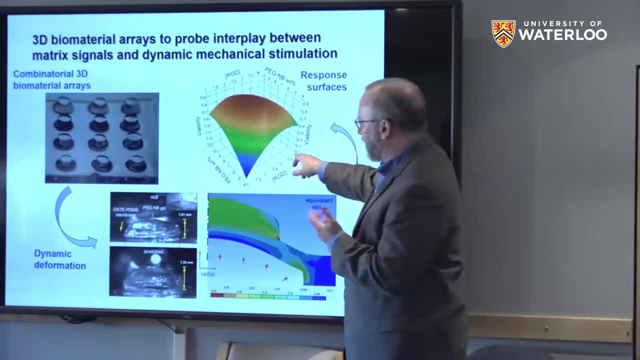 if you superimpose mechanical stretch on those, how does that influence things? And now you can start imagining. we can come up with these complex response surfaces where we can look at the interaction between a peptide for cell adhesion, the weight percentage of the material. 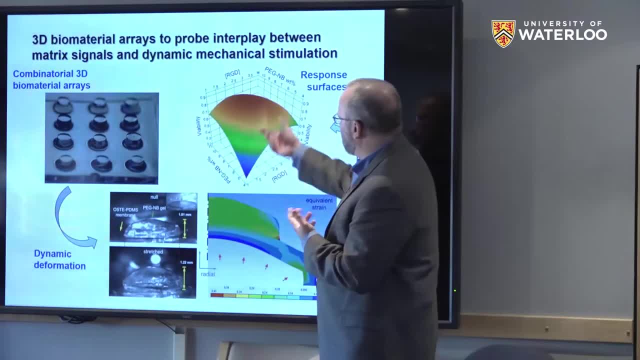 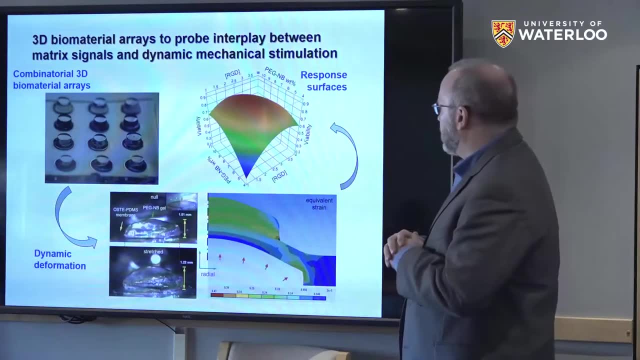 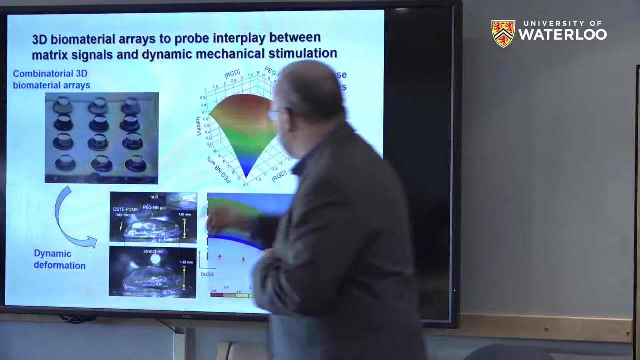 the porosity of the material. this is looking at viability under those conditions and this would be for, say, a certain mechanical stimulus. So you're now getting these multi-dimensional interactions between multiple parameters in this very complex interaction. So I'll just tell you how we do the stretching. 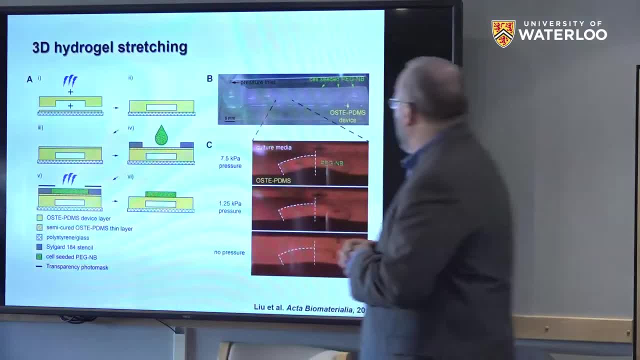 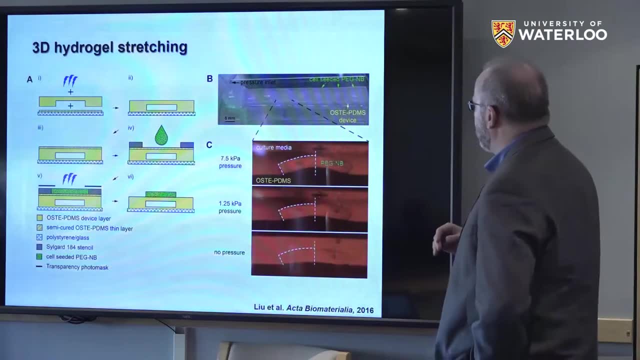 component, because this is really the main innovation, I think. here We use again the same bulging membrane system. We just changed the materials we were working with. where we still use a PDMA, but it's this osteo-PMA. I'll tell you in a minute. 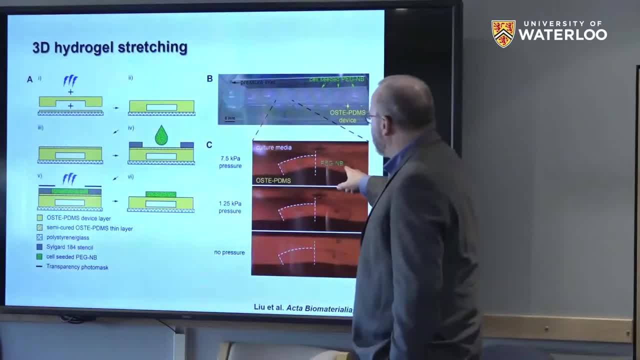 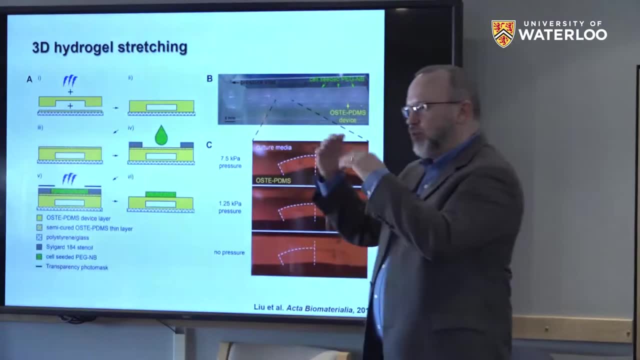 and so what we can do is we can actually get physical adhesion or covalent bonding between our hydrogel and the underlying membrane, and what this does is because the gel is now bound to the membrane. when the membrane bulges, the gel bulges with it. 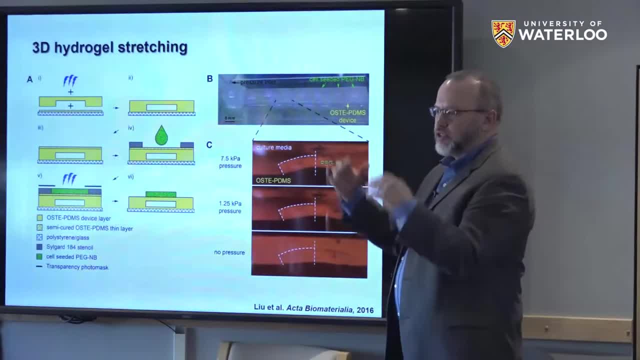 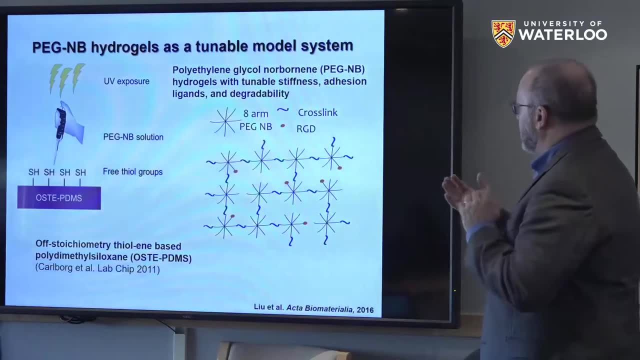 and stretches with it, and so any cells embedded within the gel are now subjected to this cyclic strain, and so the materials we use are here. it's a polyethylene glycol, norbernine, where we can. this is a nice material because we can tune its stiffness. 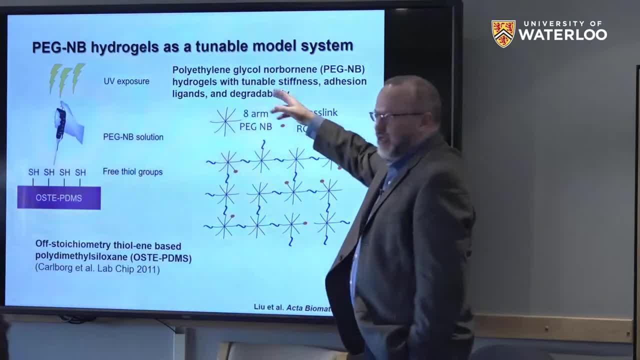 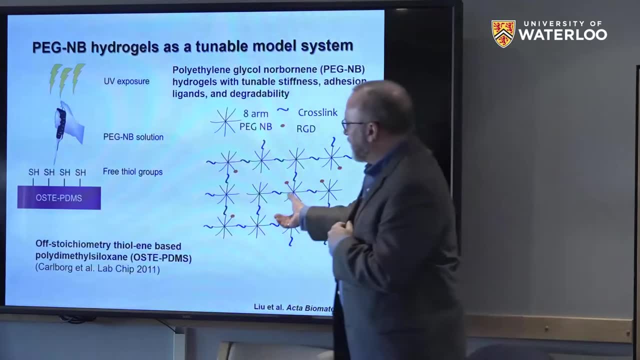 we can put in different adhesion ligands, we can change its degradability. so it's a nice model system for testing all these parameters. and then we can get it to covalently bond to the osteo-PMAs through this thioline based. 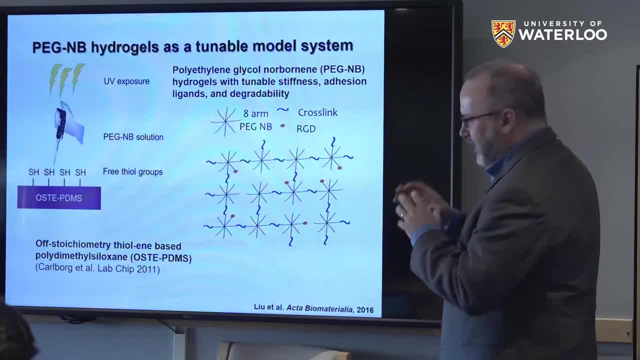 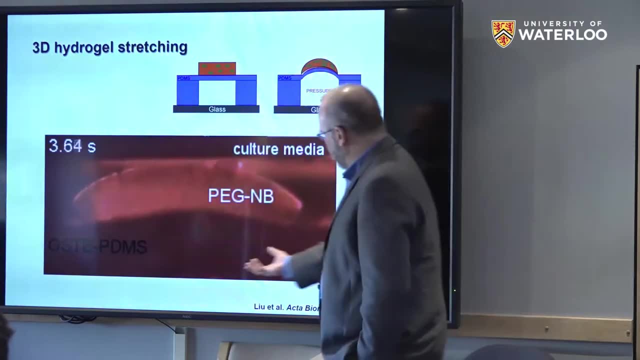 reaction, and so this is a nice model system again to test this and allows us to stretch, and so we get things like this. so you can see, here's a bulging membrane, so we're applying an air pressure down here, bulging the membrane and stretching the gel. 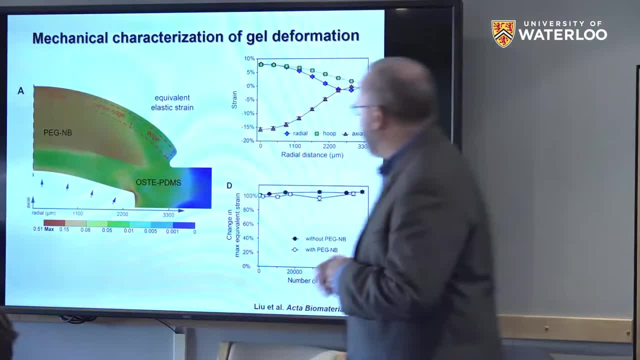 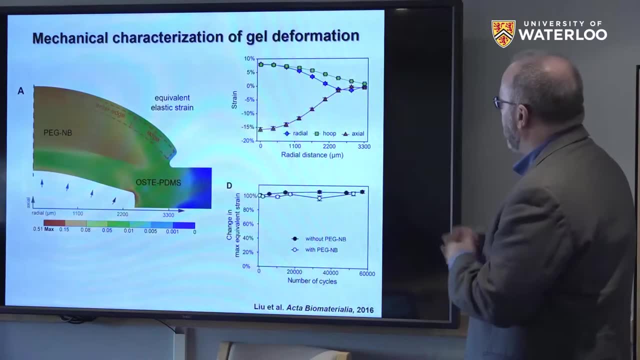 and the cells within the gel feel that stretch and then we can do finite element modeling to look at what are the forces and deformations being exerted in the gel and presumably then the cells see that. you can see that it is quite complex, but there are regions. 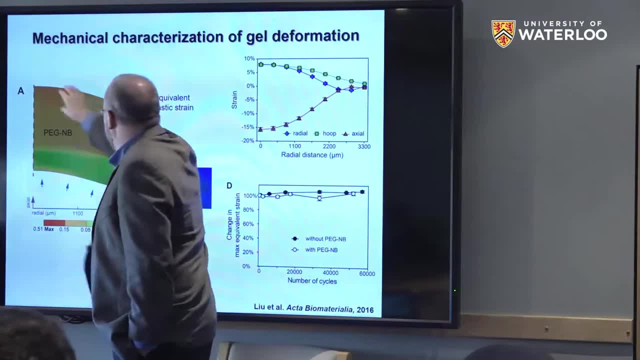 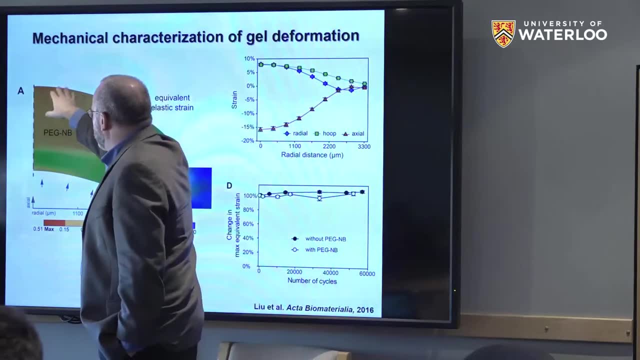 where again, you know, if you look at the different components, there are regions where it's relatively uniform up here and then regions down here where it's really relatively uniform. so what we'll often do is confine our analysis to say that there's a different level. 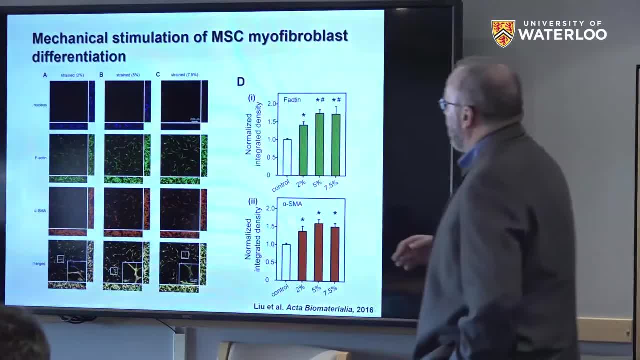 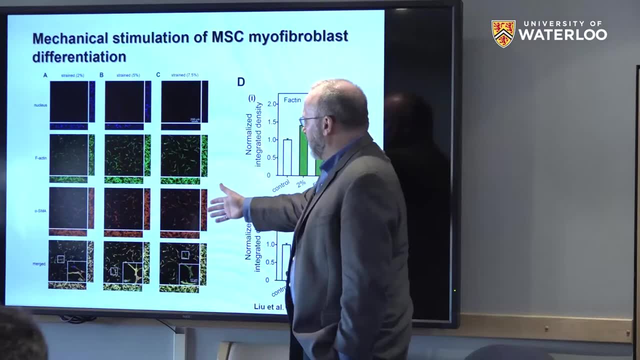 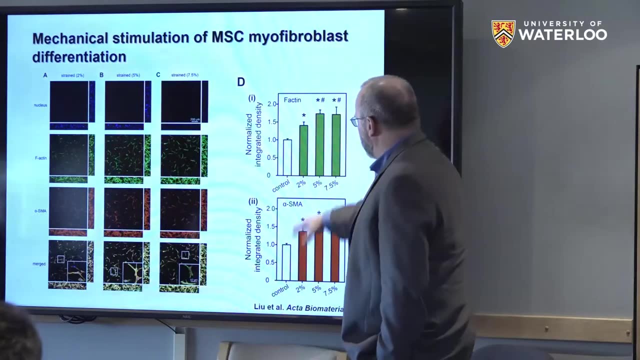 of strain. and this is a busy slide, but it's just to show you that with different levels of strain we get different responses. looking at actin, which is a cytoskeletal protein. looking at alpha smooth muscle actin, which, again, we expect to go up with strain. 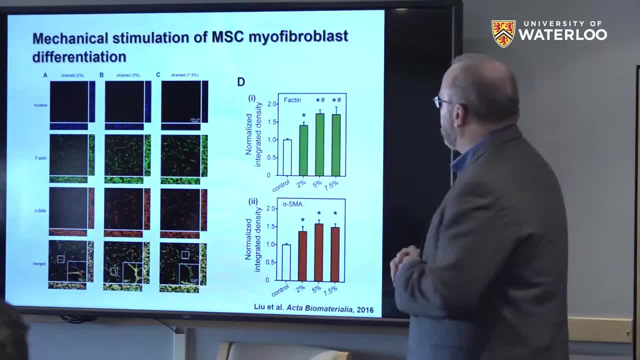 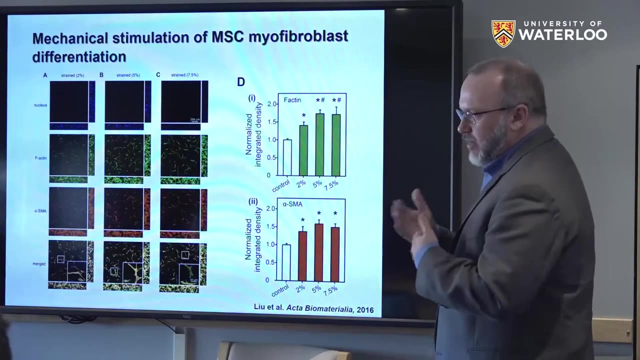 and you can see that we see this increase in F-actin, increase in SMA, with strain versus control in a 3D system. now, these two parameter multi-dimensional analyses now move them to 3D. the other thing we're interested in, though, is not only. 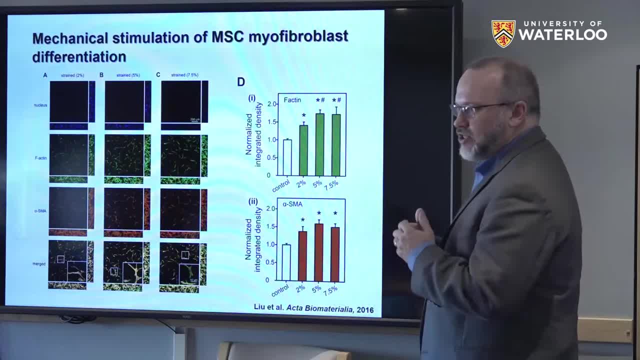 stimulating them, but measuring and looking at cellular level what's happening? but what's happening at the tissue level, are these physical forces we're applying in this stimulation we're applying, actually helping change the mechanical properties, because that's the one of the motivations for all this work. 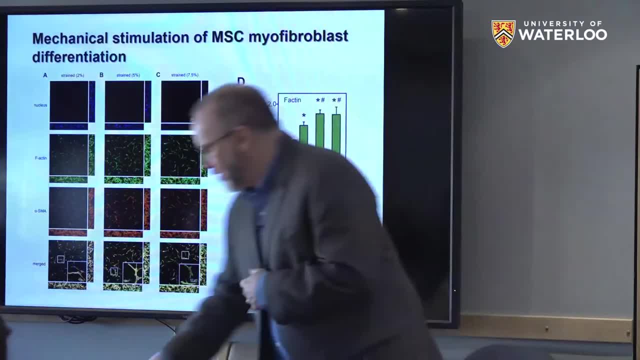 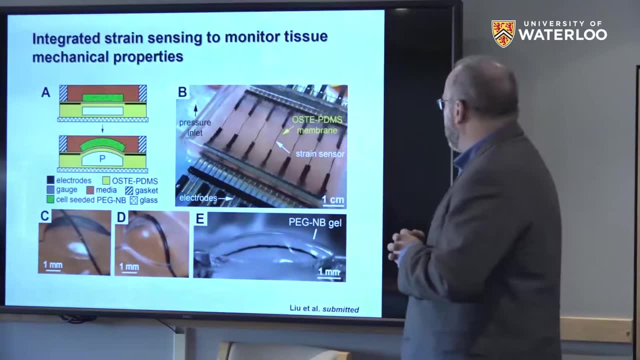 is that it can use mechanical stimulation them. And so what? a postdoc in our group? this is a collaboration with Yu Sun at University of Toronto. Luke McQueen was a postdoc in our group, and then Haijiao Lu, who just graduated, picked this up. What they did is they came up with a way to 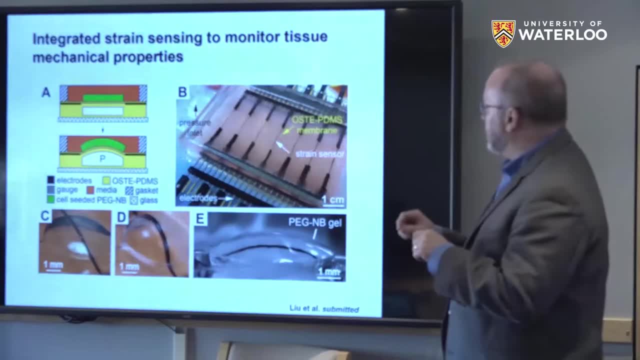 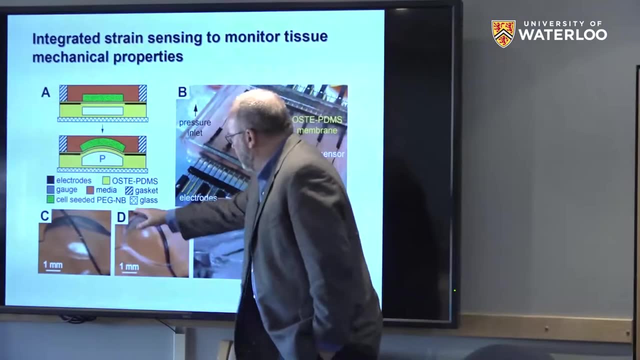 embed carbon nanotube based strain sensors into the PDMS, the bulging membranes, And so the idea here now is: you have these strain sensors and when you bulge the membrane, these strain sensors stretch And then we can. so this will give us a way to monitor the amount of deformation of the membrane. 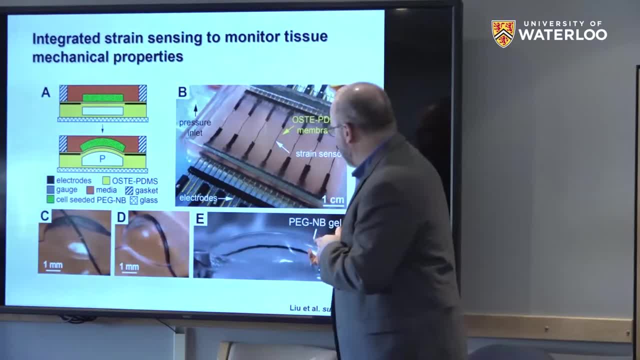 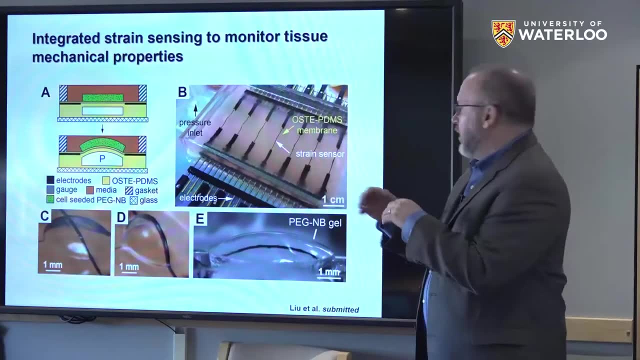 right on the chip, right in situ, And now you can bond these gels to the top of the membranes and as the membrane bulges and the gel bulges, we can measure the amount of deformation. And so if something is softening, for example under 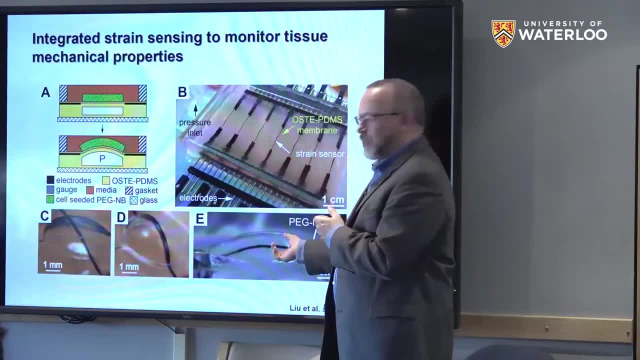 the same pressure, we would expect more deformation. We can then correlate the strain to the properties of the tissue and vice versa. If this is stiffening up, we will expect less deformation and we can monitor that. So this is a way that we can monitor the membrane as the stress potential varies. So today we want to. 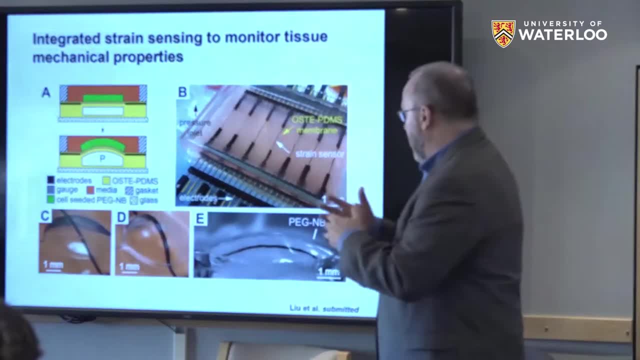 monitor the imagination time-治 göreann. we'd expect less deformation and we can monitor that. so this is a way that we can mostly right on the tissue in a monitored mechanical properties and also mechanically stimulate the tissues and monitor how the properties of the tissue 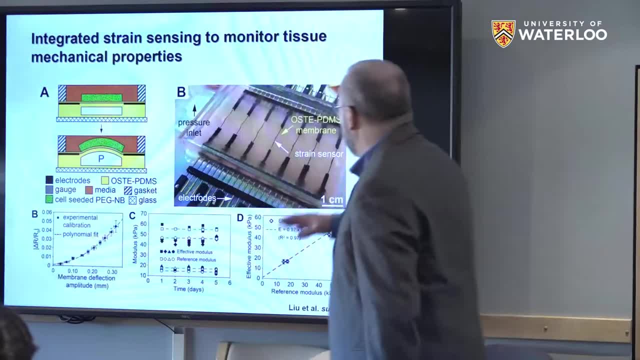 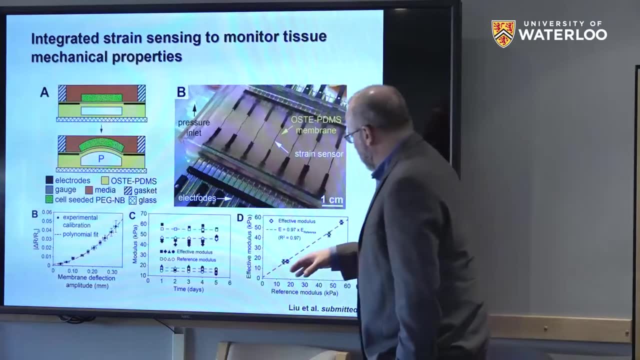 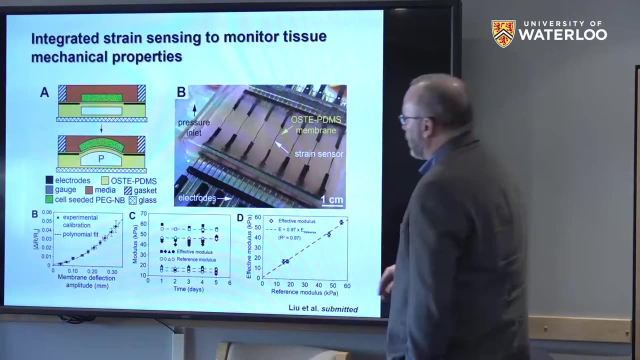 change over time. So Haijiao went and did the sort of necessary calibrations and demonstrated that when you measure tissue properties using this approach, using the using- these are the reference properties and this is what we measured with our strain gauges- we get very good correlation. So the strain gauges are. 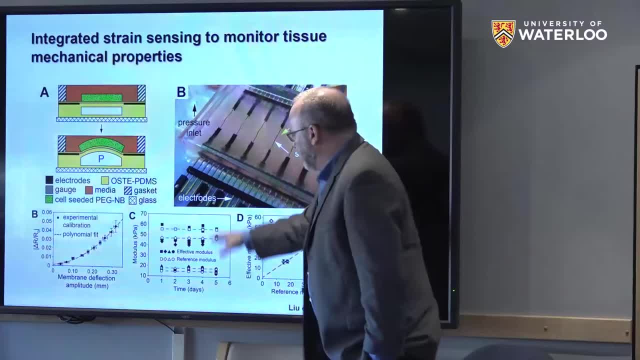 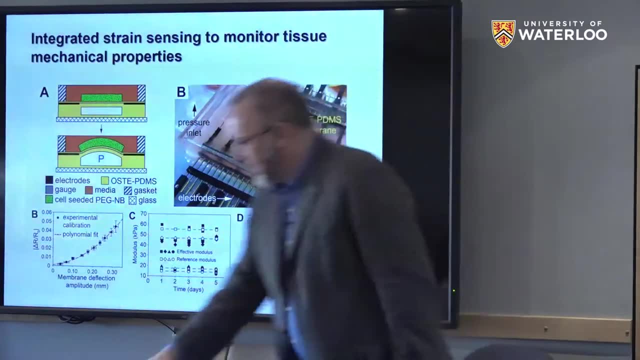 effective at measuring over a wide range of moduli that are of interest for the types of materials we work with, And so we demonstrated this in two ways. One is shown here. In this case, what we did was we, rather than just stretching this gel, 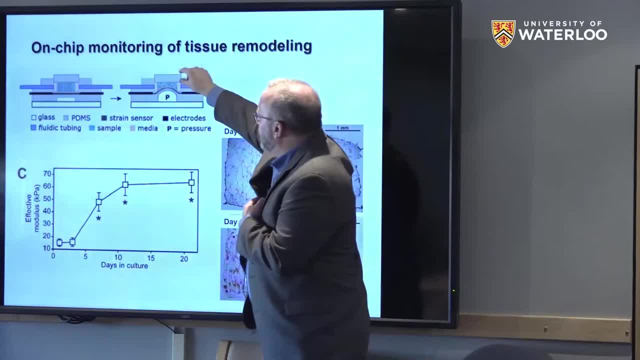 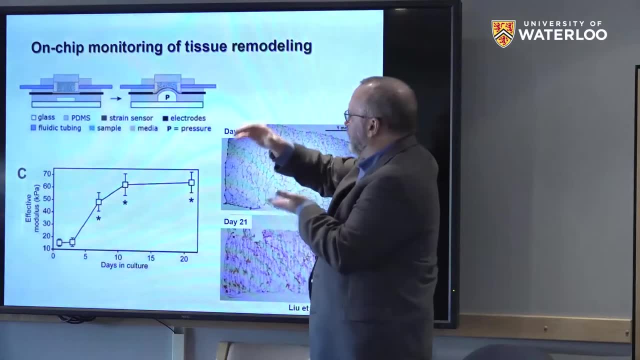 we actually compressed the gel, So we put a top on the on the on here and so as the membrane bulges it up, it squeezes the gel between the bulging membrane and the top And again to get for a given pressure if this stiffens up. 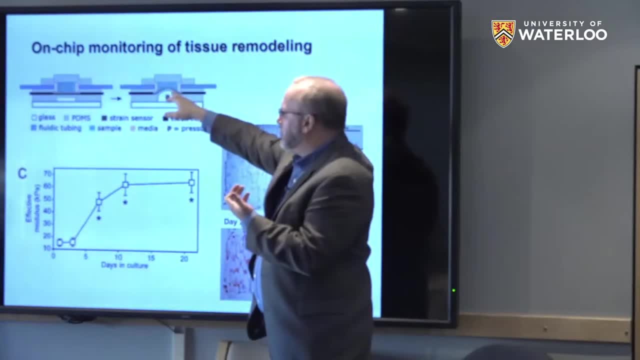 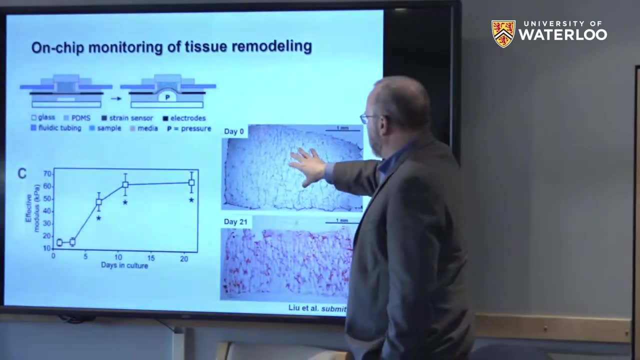 we would see less bulging, and so we can measure that with these strain gauges. So this is an example where this is Luke McQueen's work, where he took stem cells and embedded them in a hydrogel. this is what it looks like at day zero. 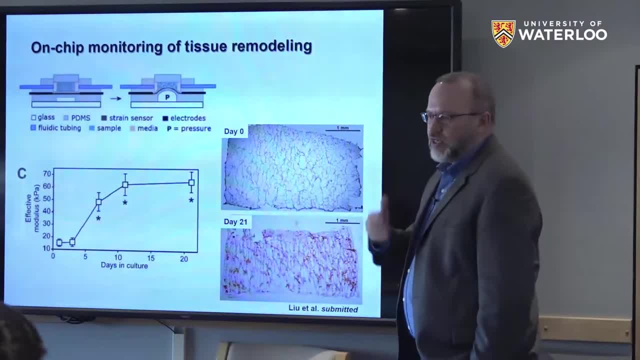 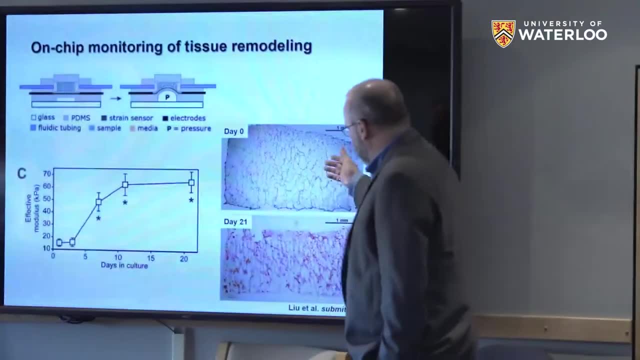 and then grew them for 21 days in a in a culture media that encourages bone growth or bone differentiation, And the red standing here is for alizarin red to show bone And you can see we do get some bone nodules forming within the matrix. 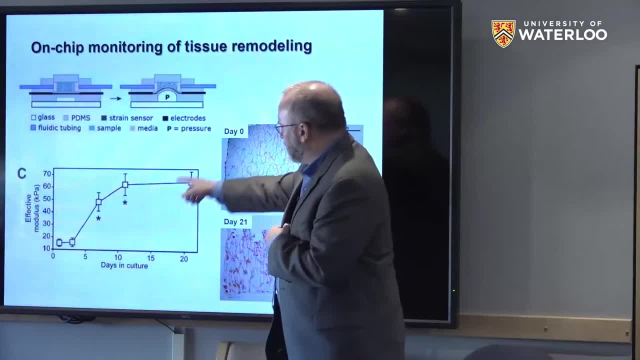 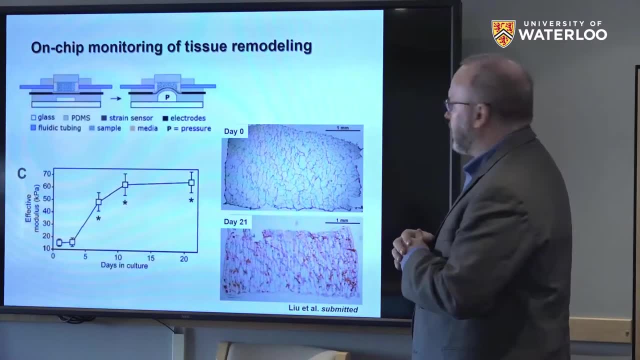 stiffening it up and we pick that up with the strain gauges. You can see this significant increase in the stiffness starts around 15 kilopascals and ends up around 60 kilopascals after three weeks in culture. So in this case, 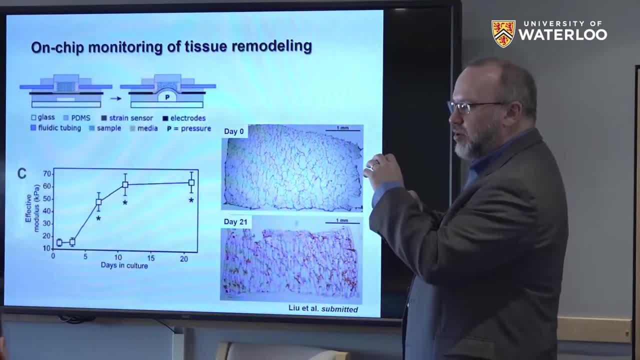 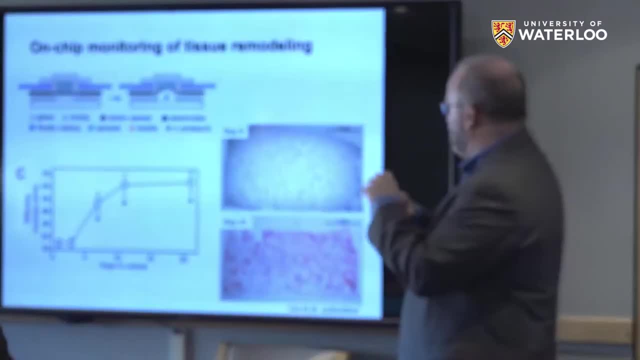 we weren't mechanically stimulating, they're just sitting in there statically and then periodically Luke would test them, Kind of like just a standard mechanical compression test. He would just, you know, at these different days he would do a test and then let them sit statically. And it was nice because he 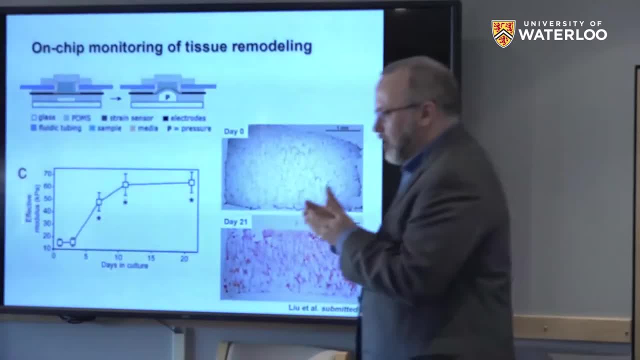 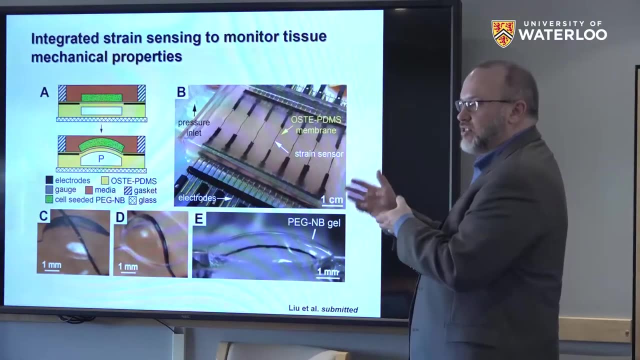 could monitor the change in properties over time. The other experiment that Haijiao has done is to use the fact that we can cyclically deform these tissues over time and ask: how can stimulation change how the tissues grow, And can you then and then? 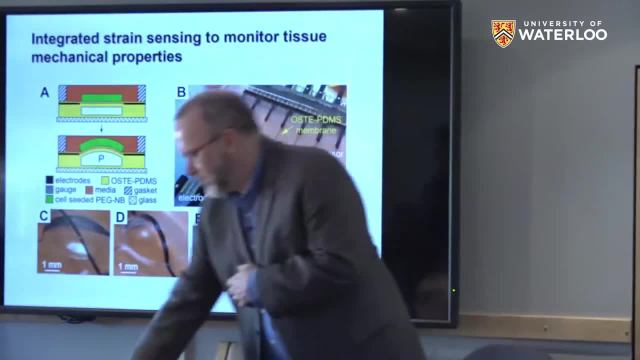 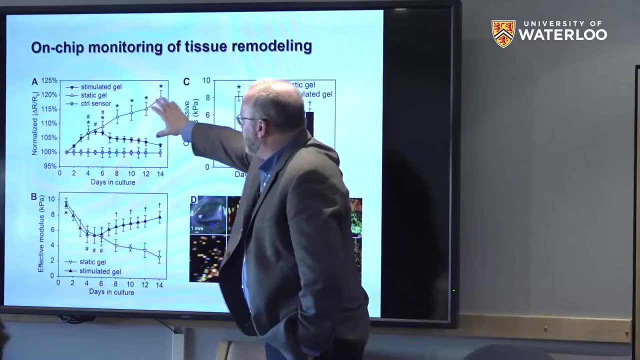 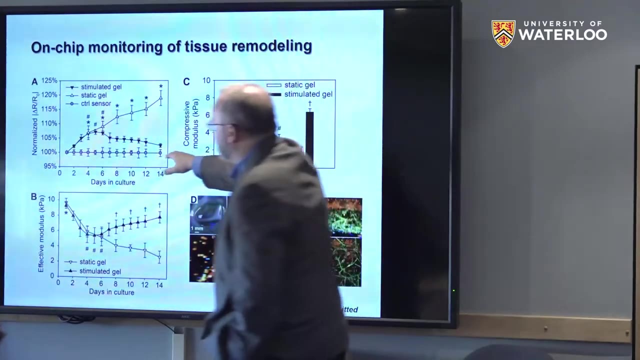 using the strain gauges. you can monitor that change at the same time, And so those experiments are shown here. So let me start here. So this is the sensor output alone. The control sensor is just a sensor sitting without anything growing on it, and you can see this is doesn't really change over two weeks in. 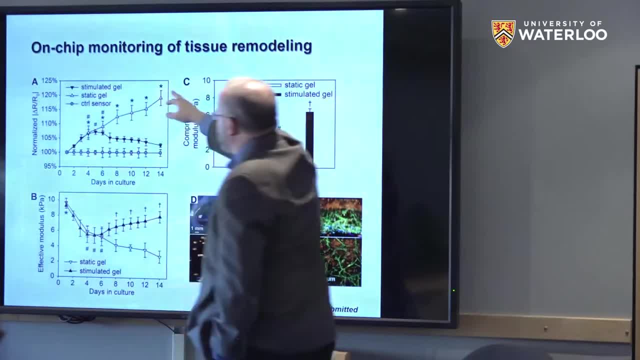 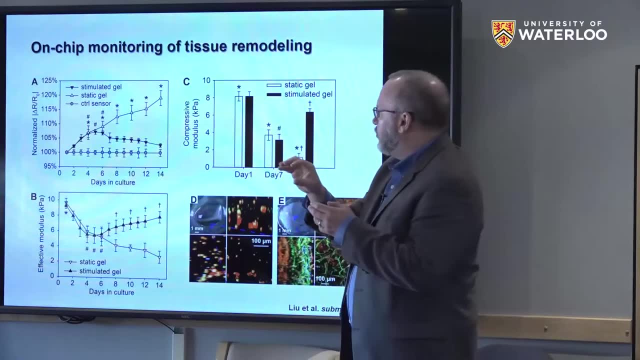 culture. This is a gel that's grown. these are gels that are grown statically. So we take a gel with with stem cells- human mesenchymal stem cells- embedded in it, and let them grow over two weeks, And then we measure the strain and you can. 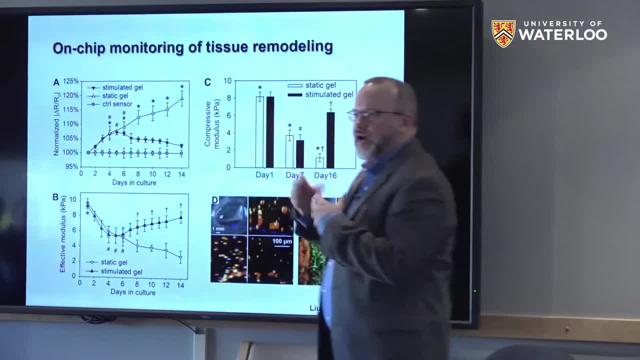 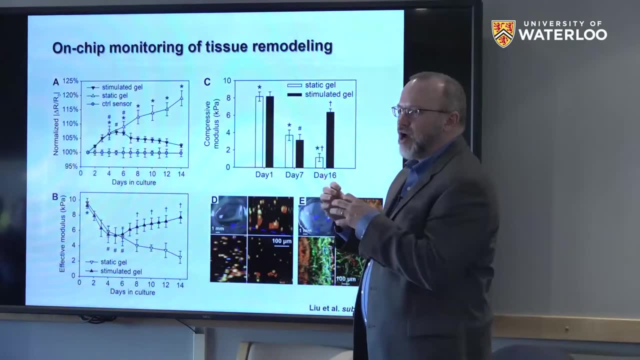 see, the strain goes up consistently. So higher strain is corresponds to softer materials. Remember, these gels are degradable, so the cells can actually chew them up and soften them, And that's what we actually see under static conditions. And then this is the case where he's now mechanically stimulating. 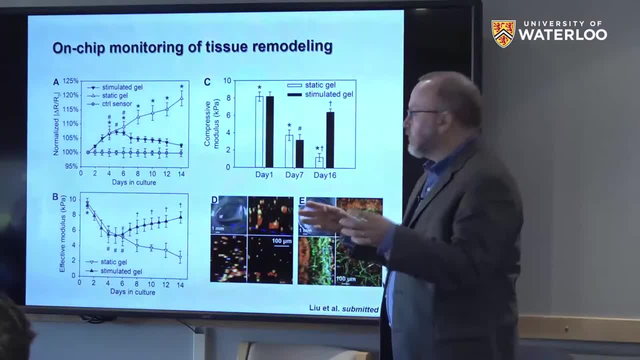 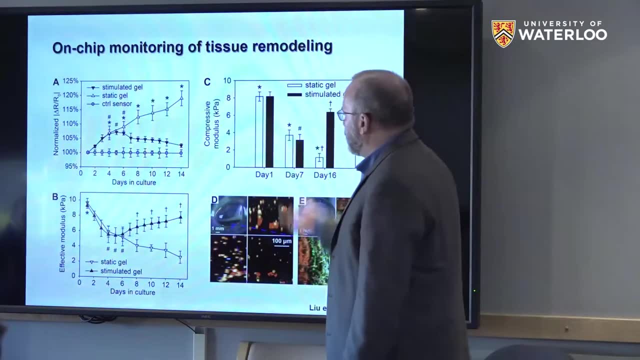 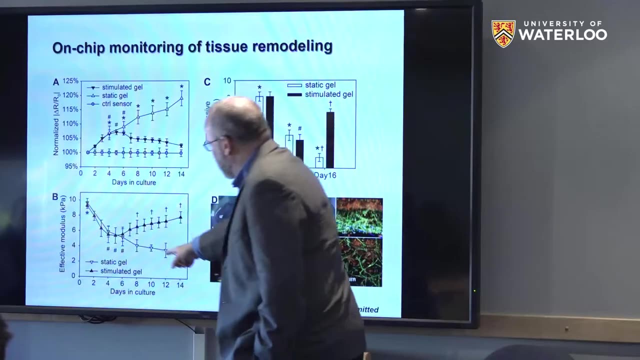 So he periodically stretches them And you can see, initially there's, there's a, there's increased resistance, but then it decreases and returns back to initial levels. So if you convert those resistances to moduli elastic properties, you see the static gels degrade or soften over time, whereas the mechanically 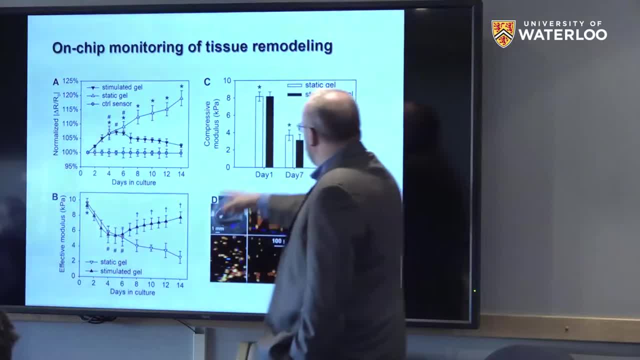 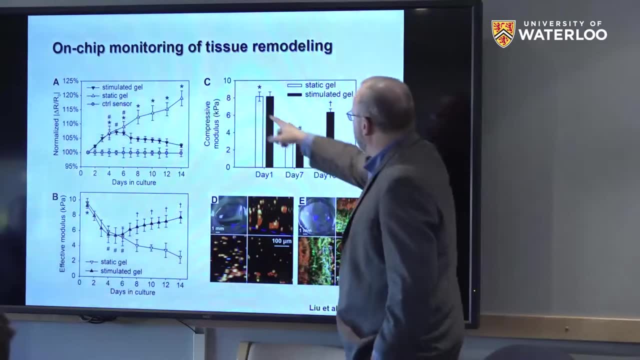 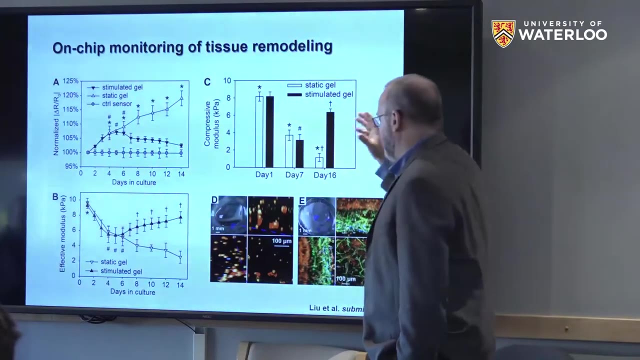 stimulated gels start degrading but then recover, And that corresponds. if we measure compressive modulus outside the system, we see the same pattern. The static gels just degrade as the cells chew up the matrix, whereas the stimulated cells recover their properties over this time period, And this is what they look. 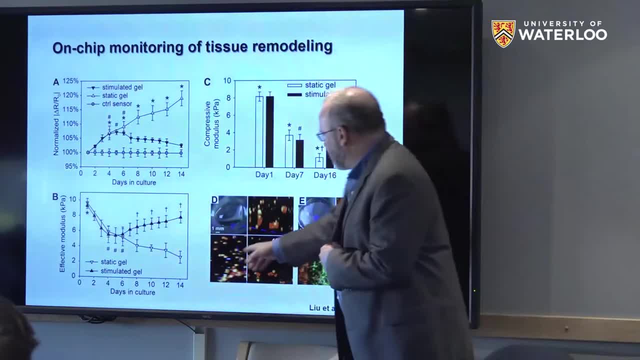 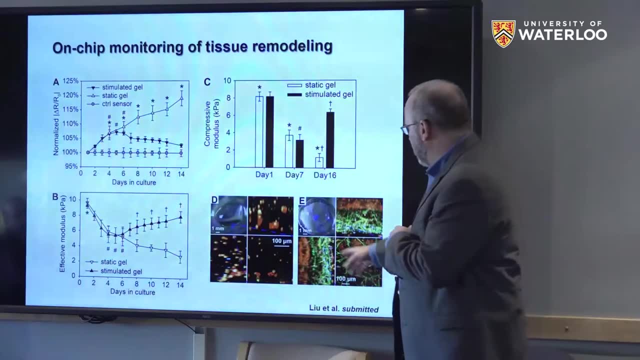 like if you look at the cells in the matrix. This is the static gels, so we can see cells in there, but not much network being formed, Whereas in the mechanically stimulated gels we get lots of collagen in red and lots of cells spreading out. 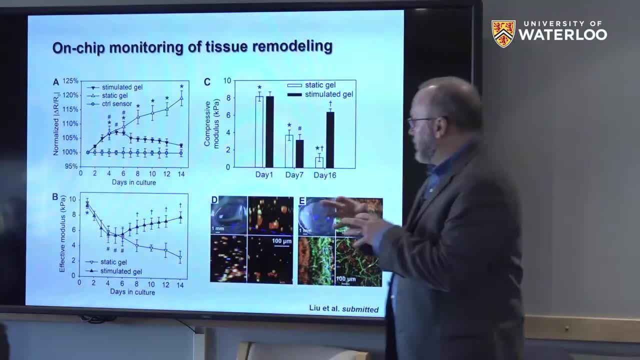 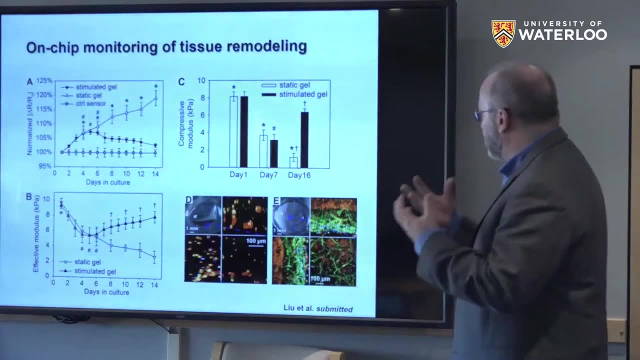 and forming this robust network. So what this suggests is that the mechanical stimulus in this case is aiding in tissue production and formation of these cell networks that strengthen the tissue, And we're able to monitor that in real time. So this type of approach now opens. 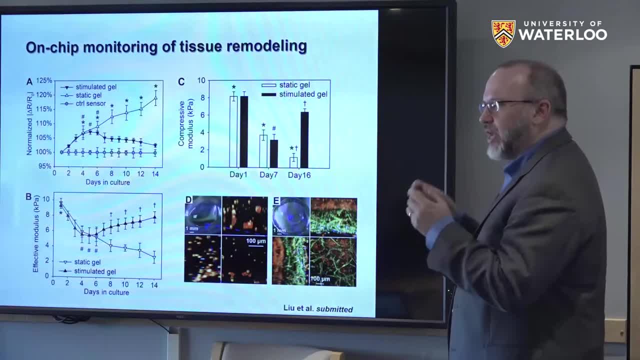 up the possibility, for you could do feedback, for example. right, If you're mechanically stimulating the tissues and you can monitor them in real time, maybe you could adjust the mechanical stimulus to get a better response. So that's something we're interested in exploring. It also allows you to monitor tissue. 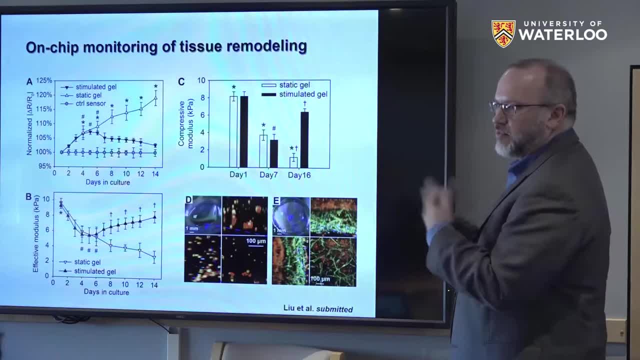 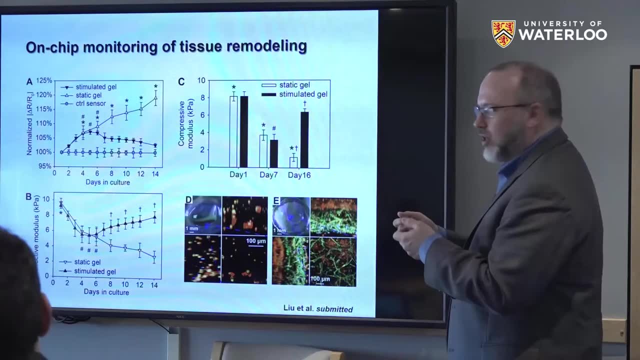 function without pulling the tissue off the system and perhaps damage or destroying the tissue. And so if you want to use mechanical stimulation to help strengthen tissues, for example, you could use mechanical stimulation to help strengthen tissues. for example, you could use mechanical stimulation to help strengthen tissues. for example, you could use: 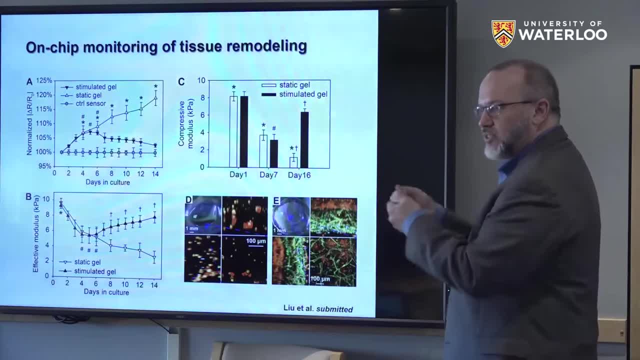 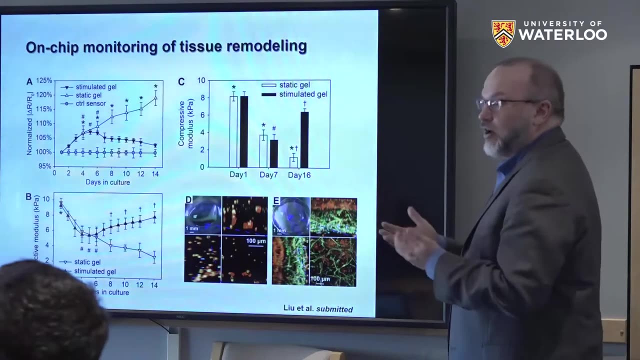 these sensors to determine. okay, we're at a good time point, it's now strong enough, let's pull it off the bioreactor. So I think this ability to monitor tissue properties in situ is a useful one for both basic investigations but also practical applications of when is long enough? when is my tissue got the? 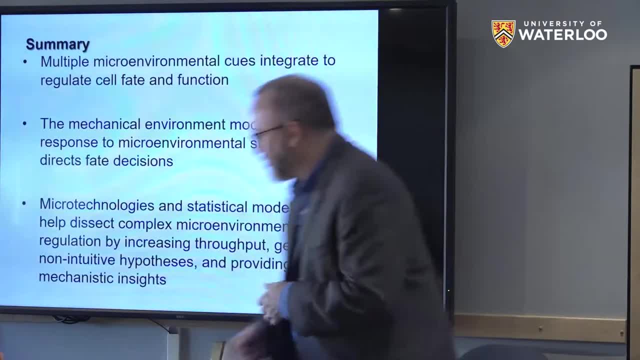 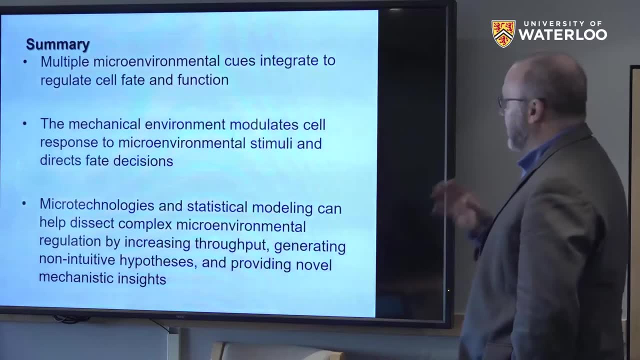 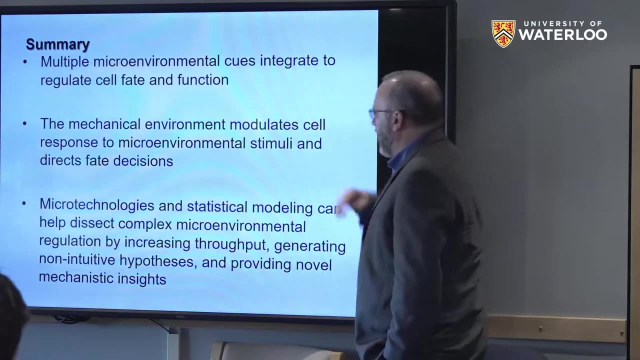 properties that I need. So just to summarize this section, just wrap up, I went a little bit over. but this idea that multiple microenvironmental cues in the environment integrate to regulate how some cells respond, and the mechanical environment plays an important role in that- And we see these technologies, these 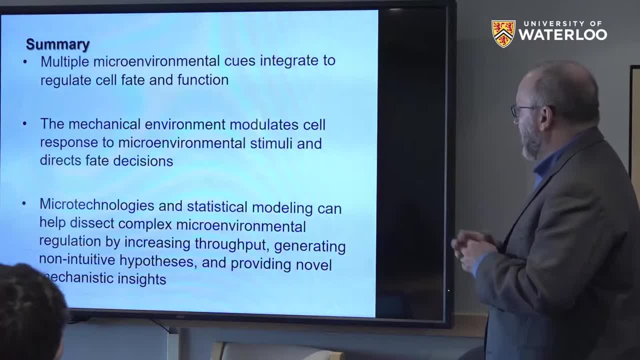 micro technologies and the statistical modeling that we apply with it are useful to help dissect some of these complex interactions. They do so because they increase throughput. you can do more experiments. They generate non-intuitive hypotheses, so things come out of these experiments that you wouldn't. 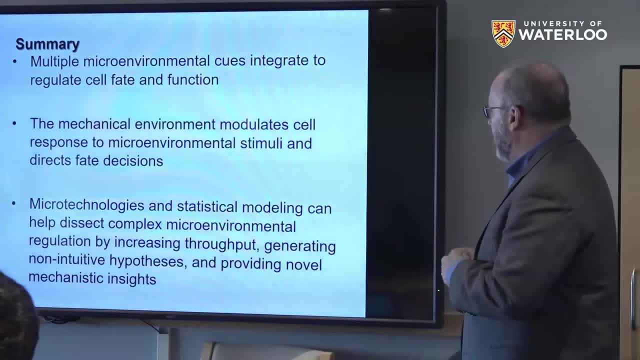 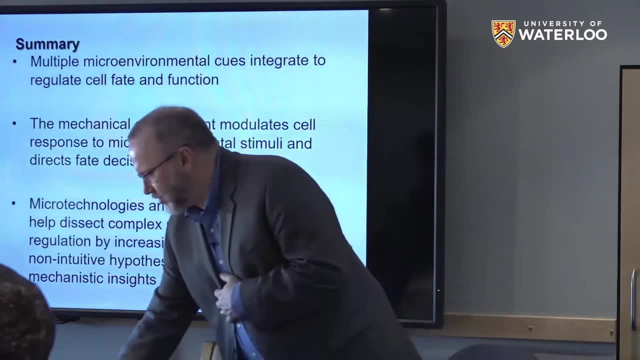 have expected and then you can go and test those specific hypotheses And they provide some mechanistic insights that you probably wouldn't get otherwise or you don't get otherwise. So I'll wrap up there and just acknowledge all the people did the work, kind of this: the six over here on the microfluidic side it. 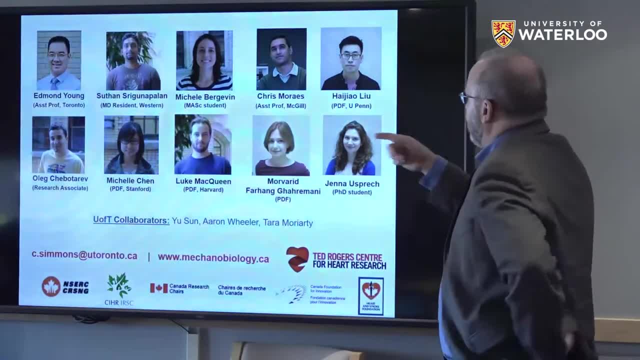 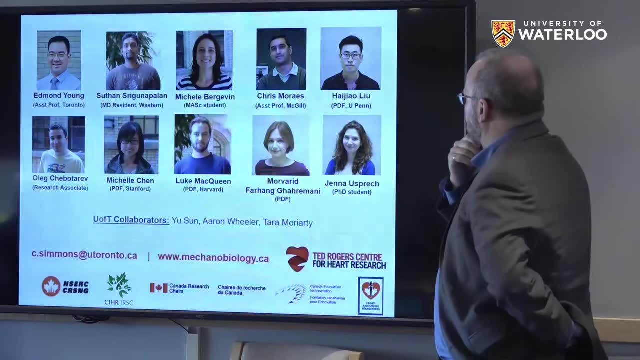 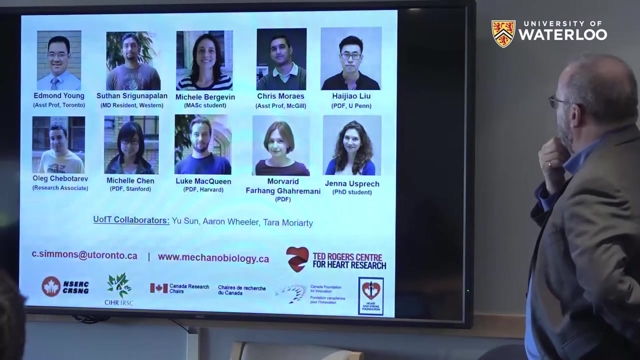 really started with Edmund Young and Sue Then, and Oleg or Alex, who did the early work, and then Michelle Chen did the valve microfluidic work, Luke did the micro the, the carbon nanotubes, initially, and Michelle did the bacterial work, and And then the stretching stuff was done, initially again by Chris, who did most of the groundwork, taken over by Hai Zhao. 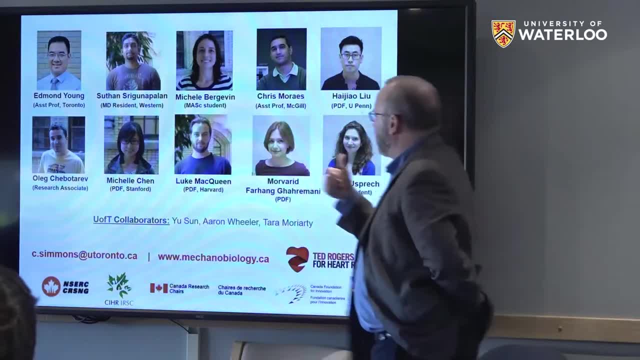 And then I guess Morvid and Luke should be switched here, because Morvid does the liver project and then Jen has been doing a lot of stretching And we collaborate with you- Sun Aaron Wheel and Tara Moriarty- on these projects. 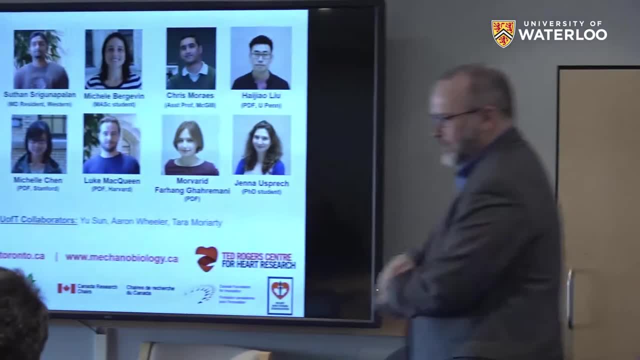 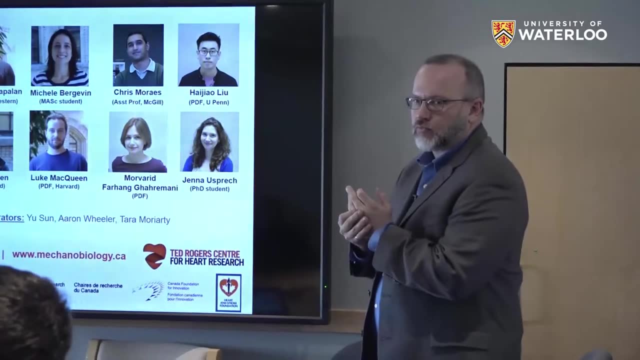 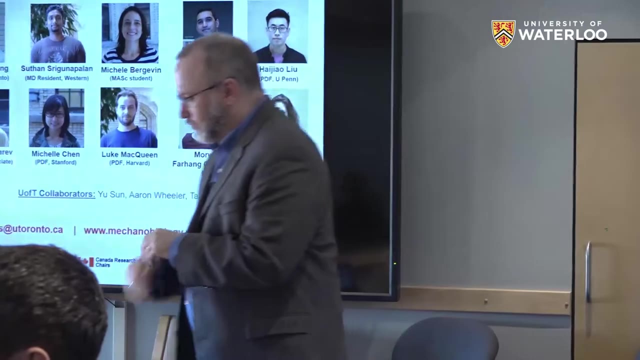 And I'd be happy to answer questions if there's time. Thank you so much, Thanks. Thank you. How was Chris Moriarty making the film with the rod where you said that he could no longer make it because it was so time-consuming? 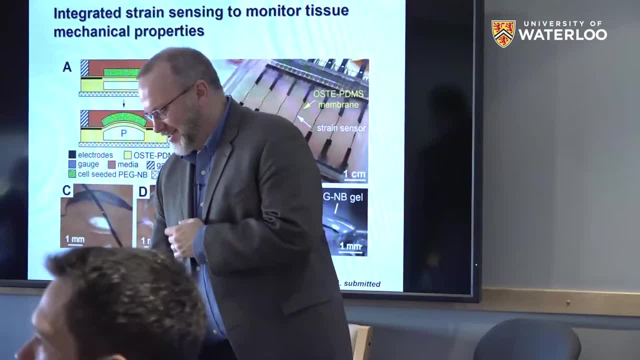 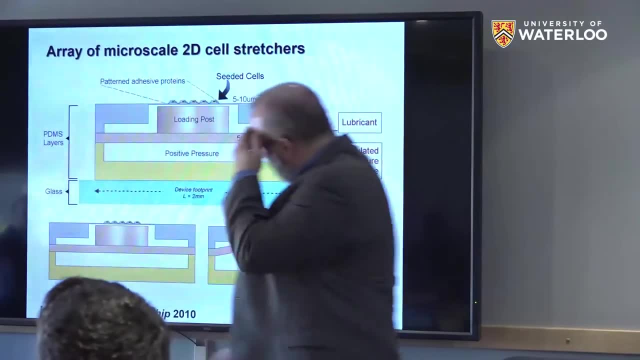 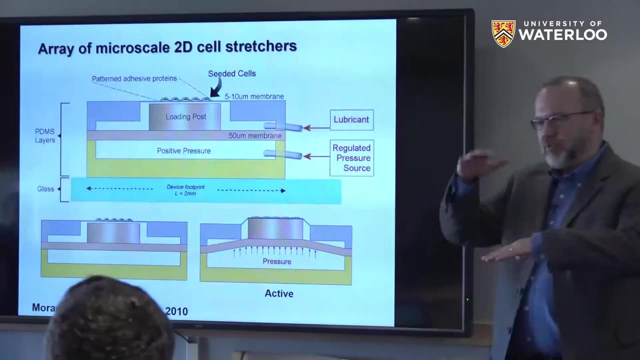 Well, he could make it. yeah, He could make it, but it wasn't worth it, right? Yeah, exactly yeah. How was he making the actual film? Yeah, so there's three layers to the device, And so each layer was fabricated separately. then he'd have to line them all and bond them all together. 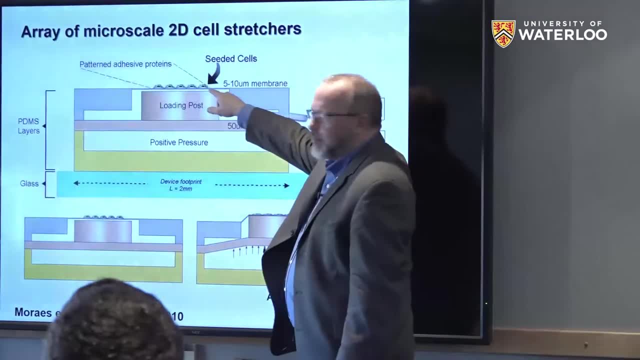 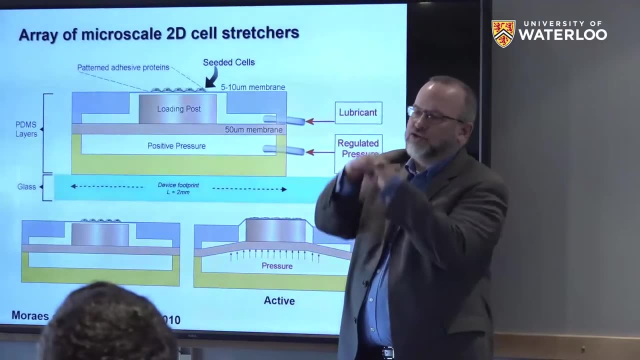 The big challenge we ran into is when you put these two layers together, because this gap is so small that often the membrane would end up binding to the loading post, And then when you stretch it, you don't get a uniform stress percent. 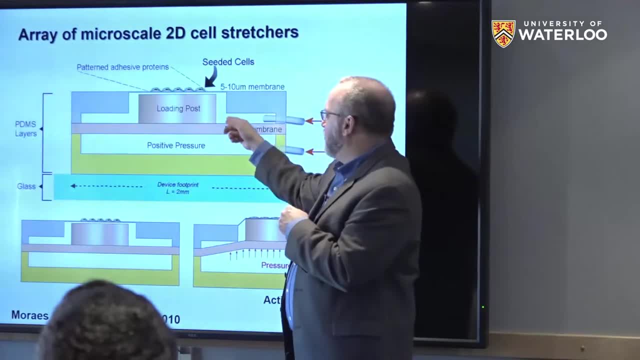 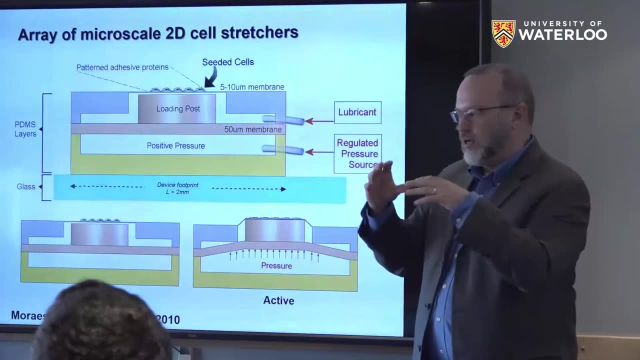 So he would actually have to assemble this with a lubricant in place, which created all sorts of challenges, because it's no longer just stacking devices, but you actually have to either pull this down or put a lubricant in place to prevent them from binding in the first place. 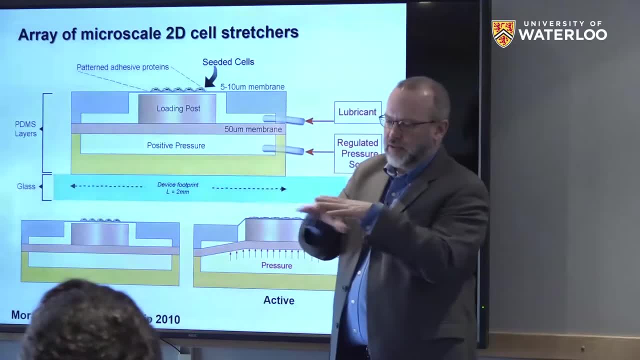 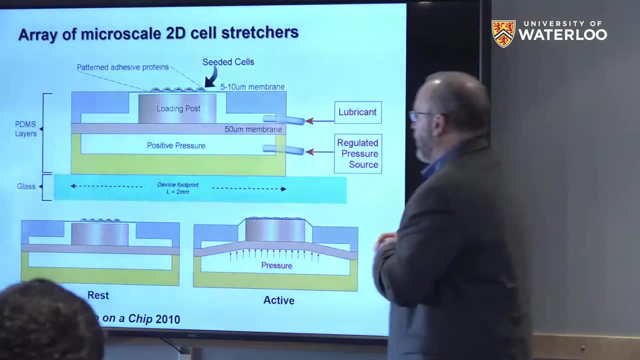 And you needed to operate it with a lubricant. So he had to put a lubricant in here to get the equi-axial profile, which assumes no friction between the loading post and the membrane. So that was one challenge. Otherwise he came up with all these fabrication issues. 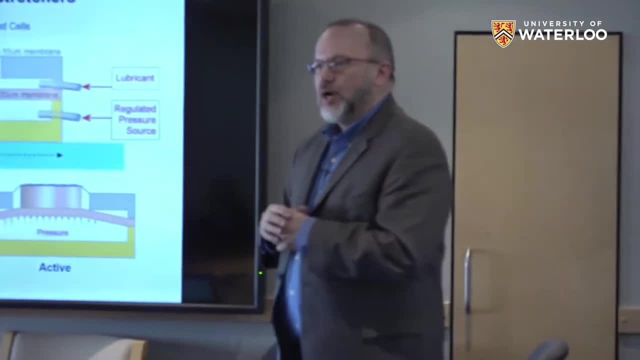 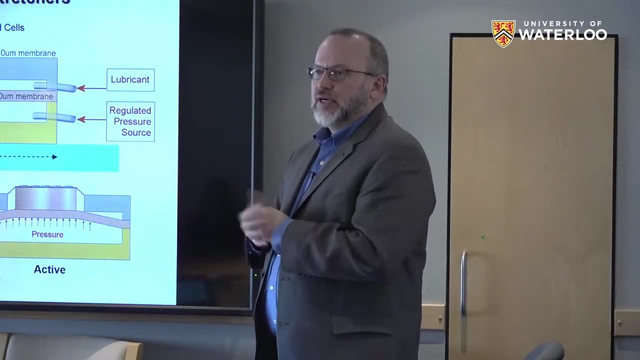 If you have to get precise alignment, it becomes a bit of a challenge. Things shrink and those dimensional changes can throw off your alignment. So there's just some challenges that are manageable. They just increase the complexity. the more layers you have and the more alignment you have. 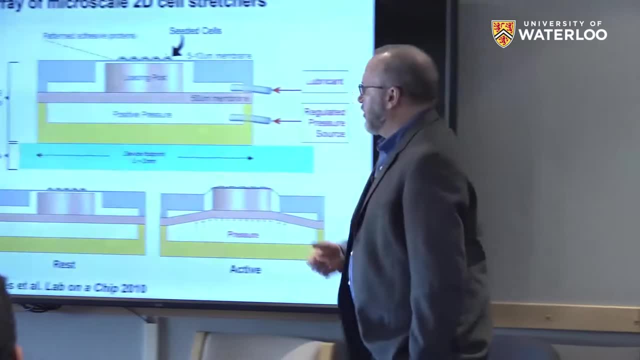 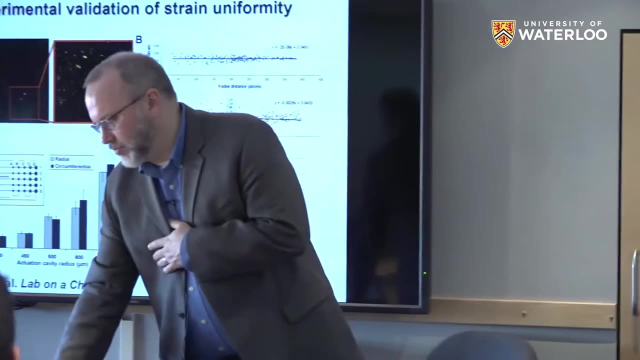 So this had to be fairly precisely aligned. But the main one was this issue that the loading post and the membrane, we had to prevent them from adhering. So the other system, the bulging membrane systems, we don't do the top layer anymore. 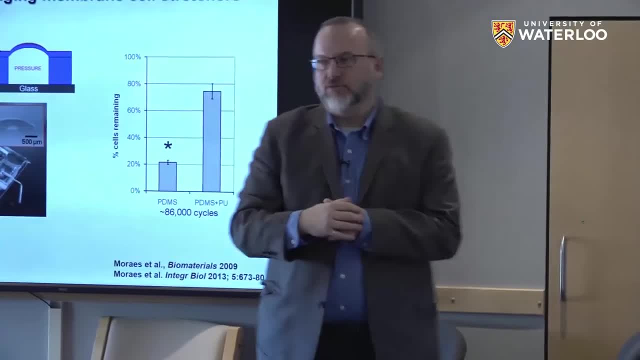 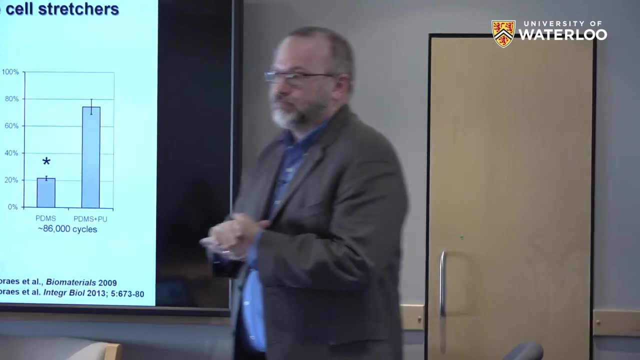 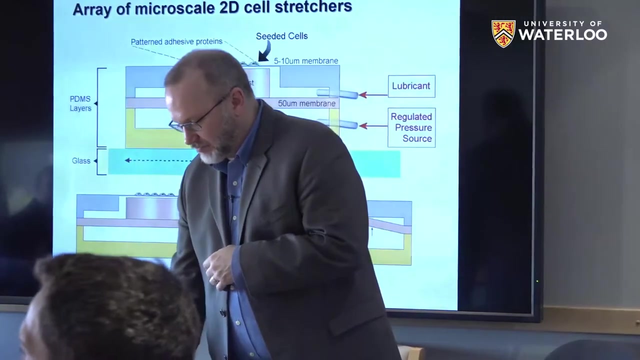 It's just a PDMS layer on a base, so it's much more straightforward. Yeah, Going back to your microfluidic chips, what do you think your next biggest steps are in this further progress? Yeah, So two directions we're taking. I would say 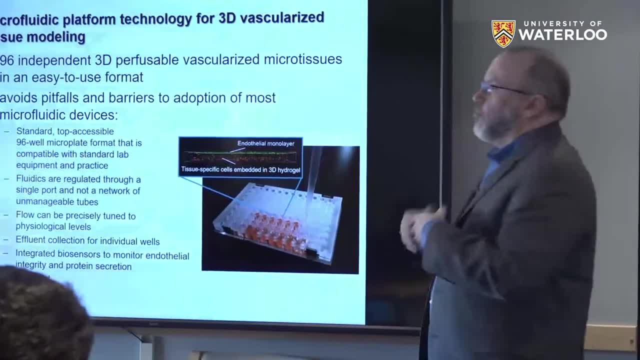 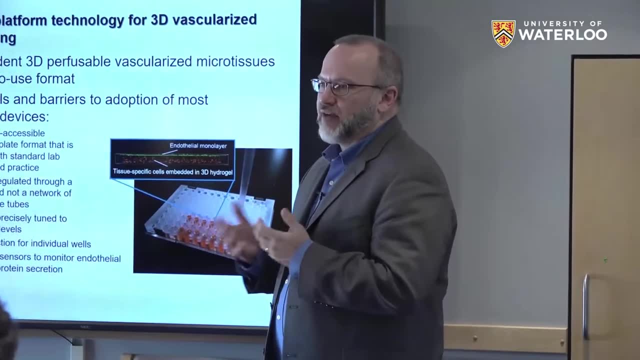 One is to – so I think this is more usable, but it's still not entirely usable, right? So it's – and it's made using things that we can do in the lab, and the fabrication methods aren't necessarily the best for if you want to make this a commercial product. 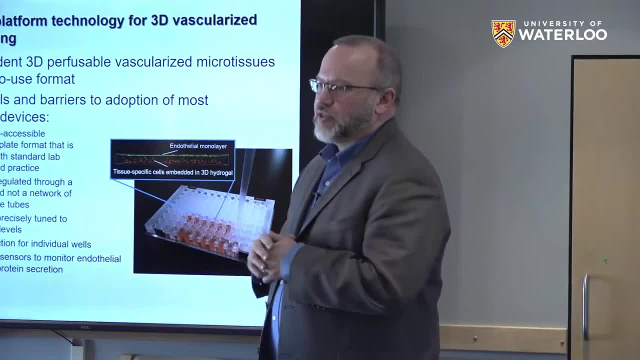 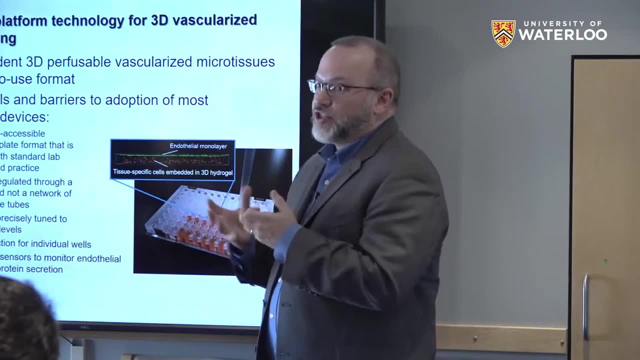 So one is making it more market-ready and commercializable, And we had some interest in partnering with a company in order to do that. so that's one direction. The other is just demonstrating that it works, That we can actually do things with this that you can't do with other systems. 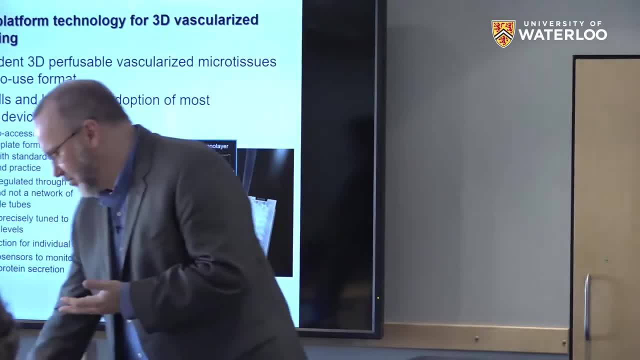 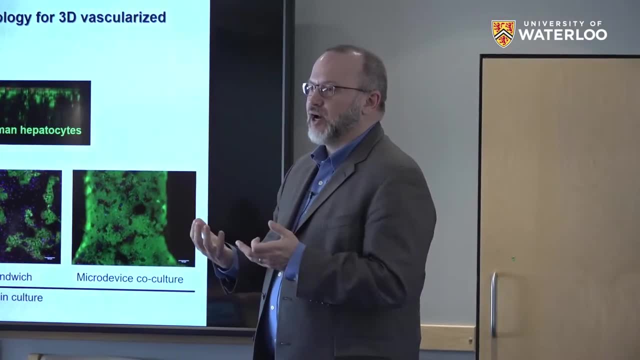 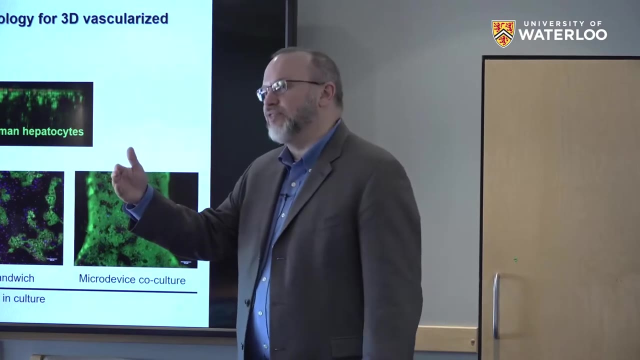 So what is the value added of this system? I think, for example, this data, which is just brand-new data. I think this is really encouraging, Because now we can show we can grow hepatocytes much longer than you can otherwise, And this – and we haven't have – you know, we haven't even have capitalized on the flow aspect, which we think will actually improve things even further. 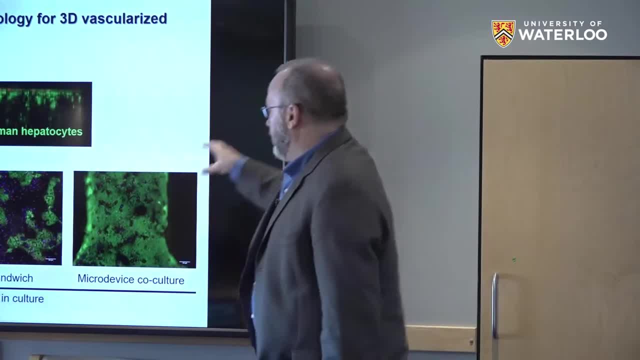 There's some evidence that suggests that. So you know, this is, I think, a nice demonstration, And then putting it in a package that someone could use, I think that calls for a lot of work, And that combination will be really powerful. 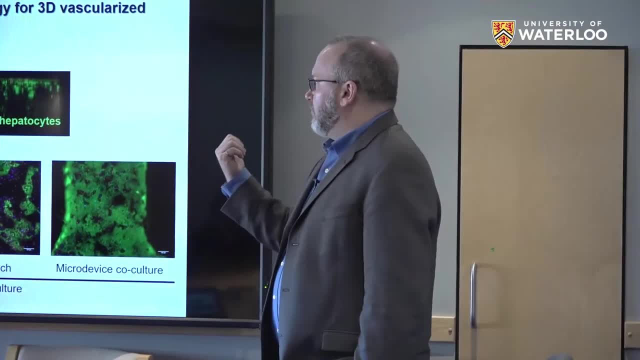 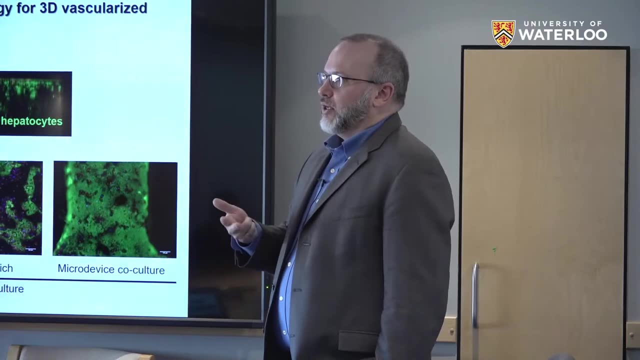 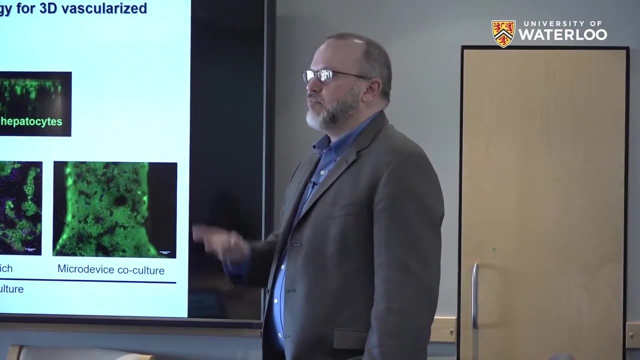 So the plan is: we're continuing to validate liver blood-brain barriers of interest cardiac we're now funded to do as well, Working and then partnering with end users, the pharma companies who will actually use these or other scientists who will use these. get them into their hands, get their feedback. 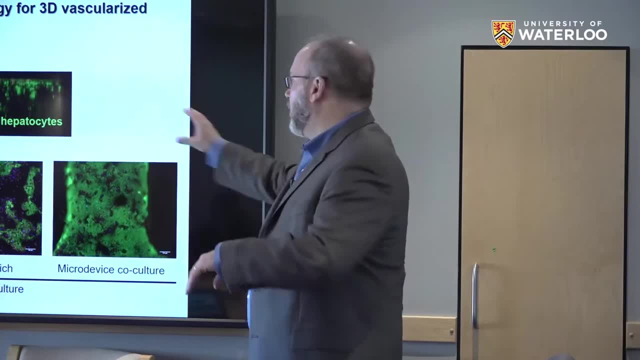 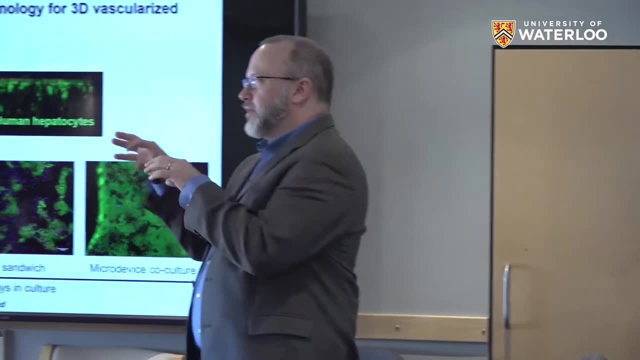 So there's a strong commercialization push and then sort of a strong produce the validation data push. And I think we're – There's a lot of evidence from other studies that if you have endothelium it improves tissue function in many cases. 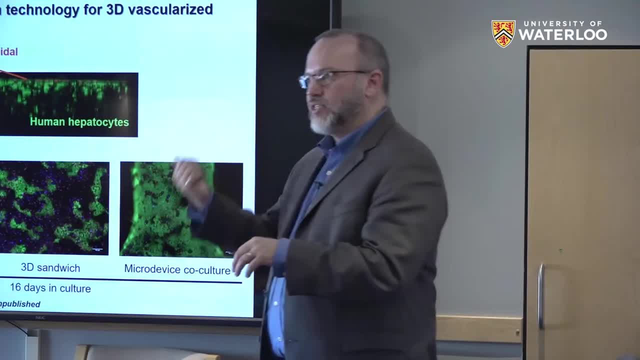 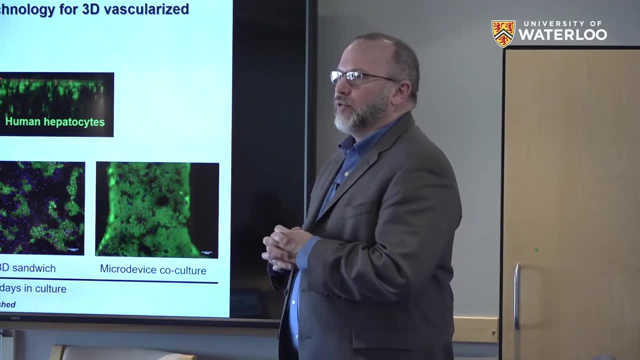 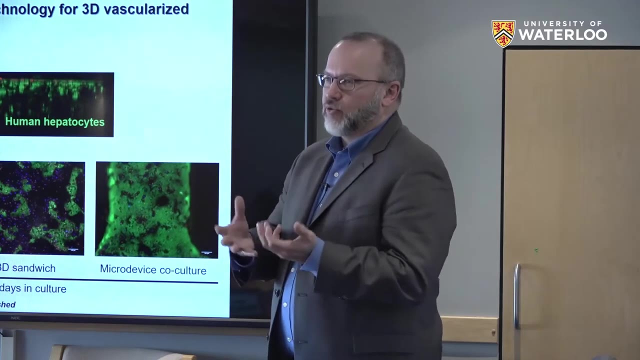 If you have endothelium with flow, it even helps more in hepatocytes or blood-brain barrier and cardiac. But no one's been able to put that in a package that makes – that's easy to use Right. So that's where I think – I'm optimistic- that we'll be able to demonstrate it, because it's been demonstrated before in other systems. 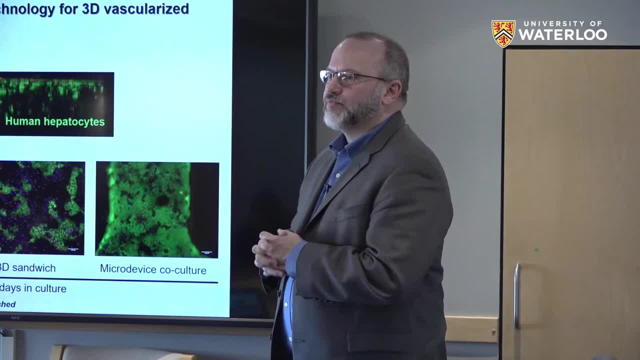 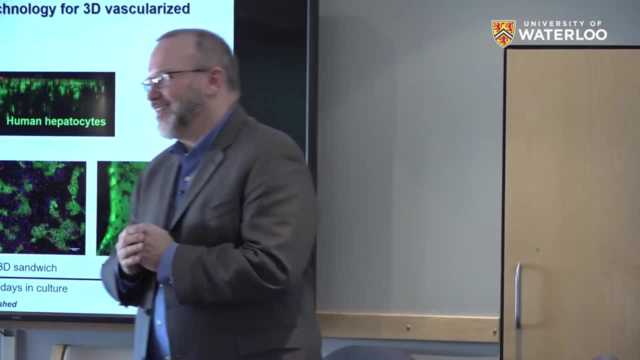 We just have to demonstrate it on our plate and make our plate then usable. Yeah, So yeah, Very interesting getting this out of the lab. Yeah, For your lab on a chip. you mentioned that you were only perfusing it with one tube. 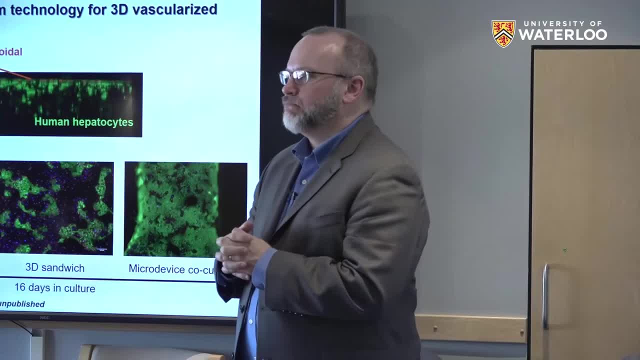 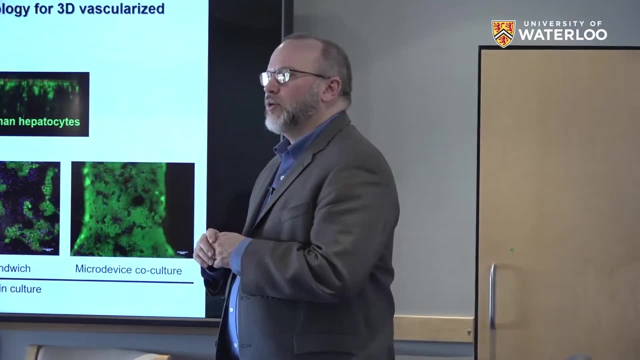 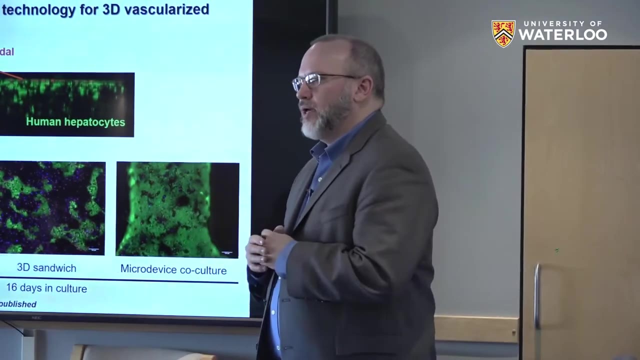 So is there a way to vary the shear stress within that one culture? Yeah, Not currently – well, you could imagine ways to do it by changing channel dimensions and things like that. Currently we actually strive to get uniform shear across all 96 wells and it's designed that way. 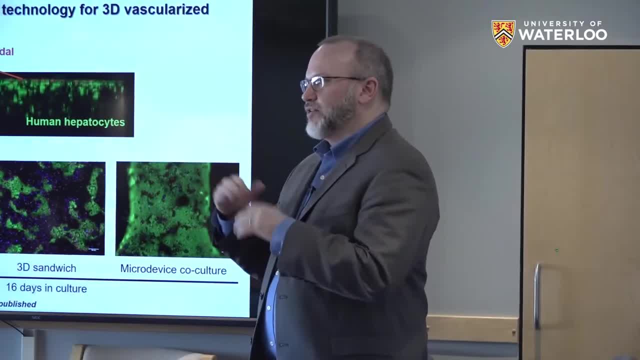 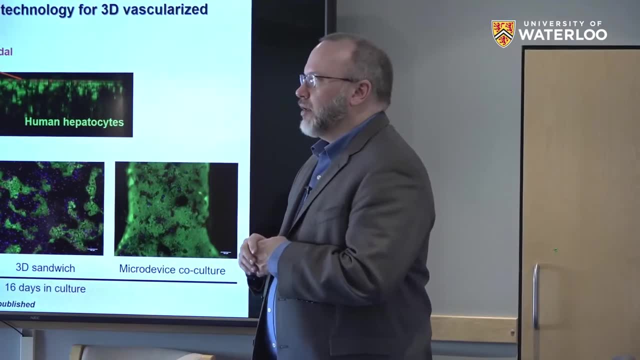 But yeah, if you wanted to, you could imagine having different channel dimensions or putting different resistances in line of different channels to get a variation of shear stress across the channel. In most of the applications that we're working in, the shear stress is set by the physiology. 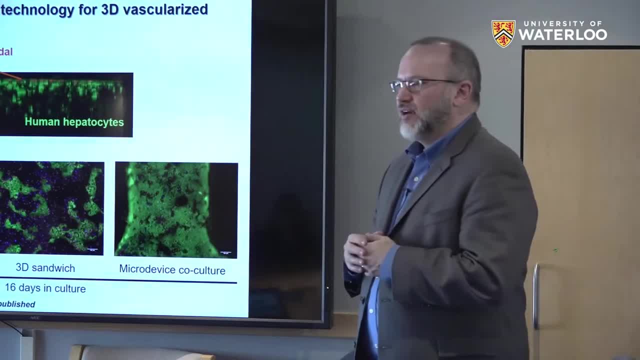 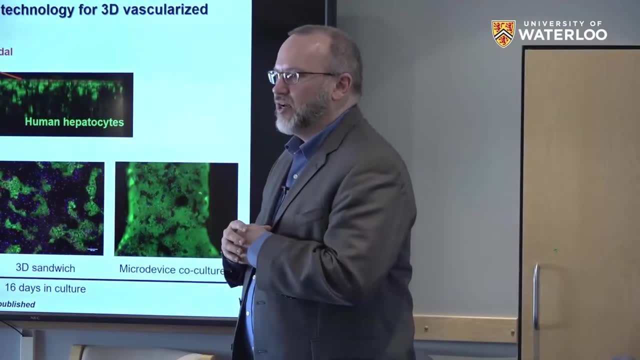 Right, It's not usually the variable that changes. So in the brain, you know, it's 6 dynes per centimeter squared is the typical shear stress and it doesn't wildly change In the liver it's less than that. 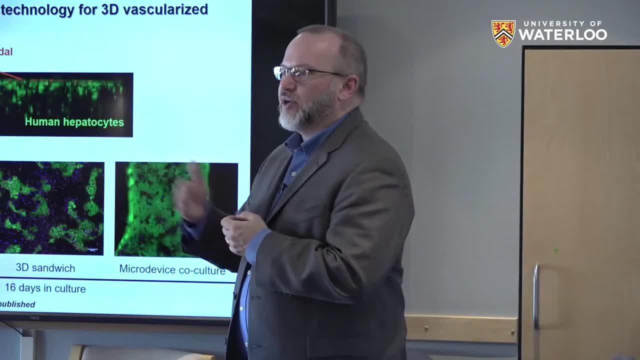 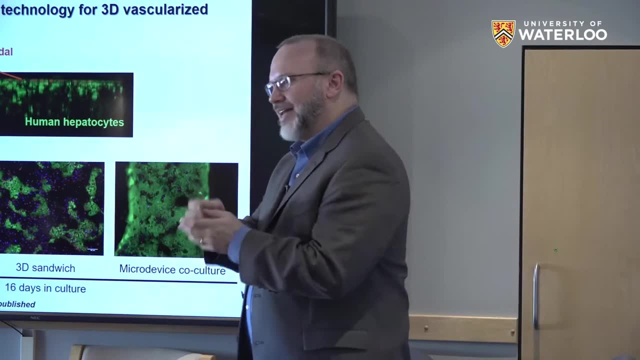 So that is a – we want it there, but we don't necessarily have to vary it for the types of modeling we're doing. But you could imagine ways to do it. Yeah, We've sacrificed that again just to have the single tube. 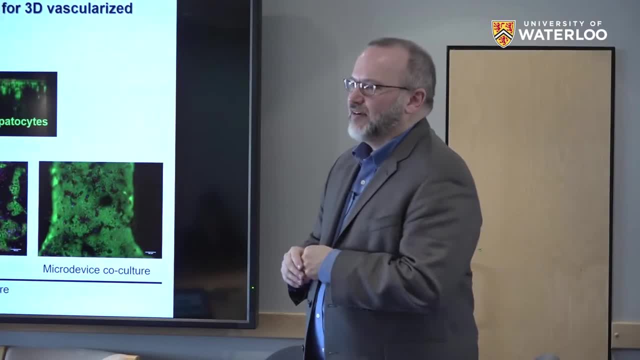 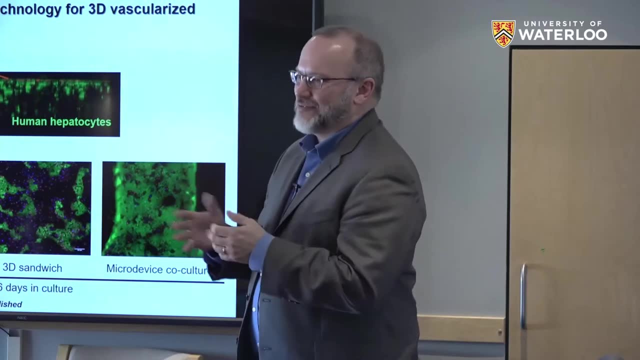 Yeah, We could have multiple tubes, but there are pictures of devices that actually have 96 tubes, 96 out, And you know, that's all you hear of them, Right? You see the picture and it's like a nice whatever paper, but that's about it. 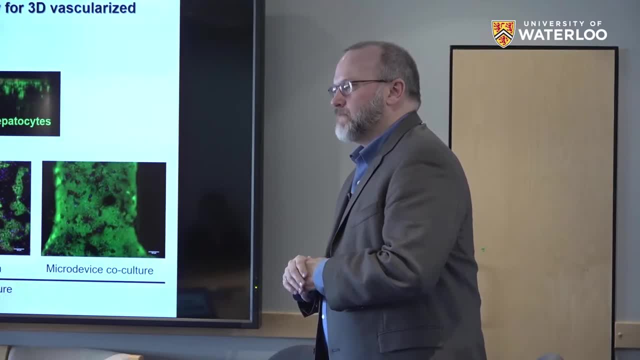 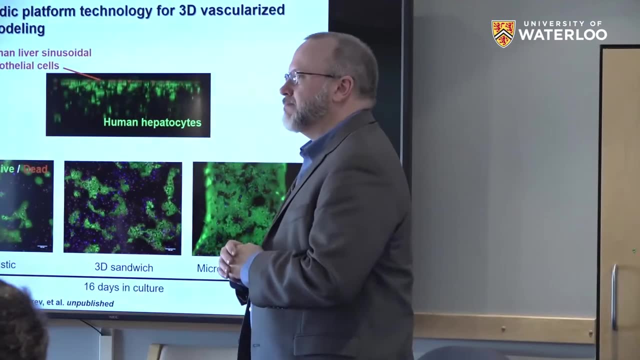 So, yeah, Yeah, You've done a lot of work on exploring the etiology of CABD and calcification of lab diseases. I'm just wondering, I mean from the clinical perspective, with the platform of microplast that is being developed in your lab. 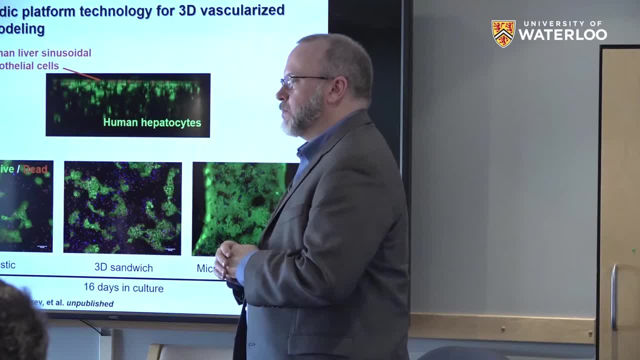 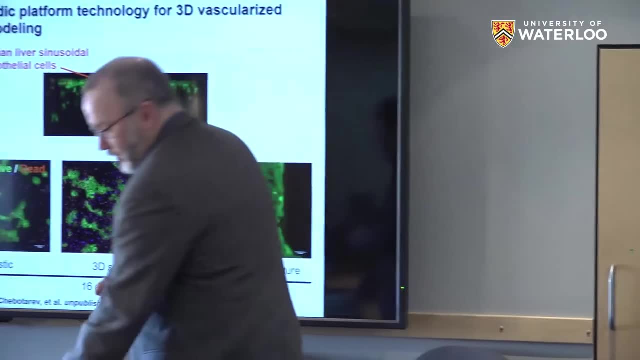 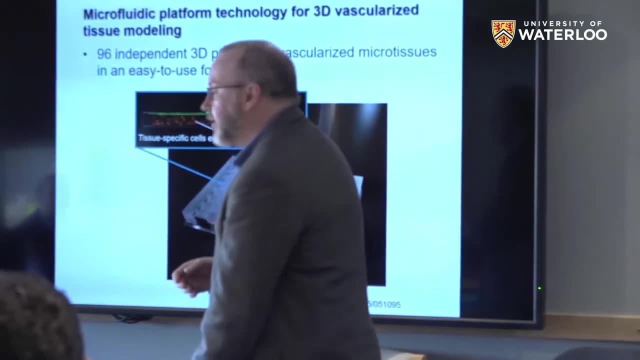 would that be possible to take a look into different risk factors such as- I don't know- aging or smoking, or male versus female? Yeah, Yeah, Great question. So what? I would say that what we are doing right now in the cardiac side is in the cardiac model. these are cardiomyocytes, the muscle cells in the heart. 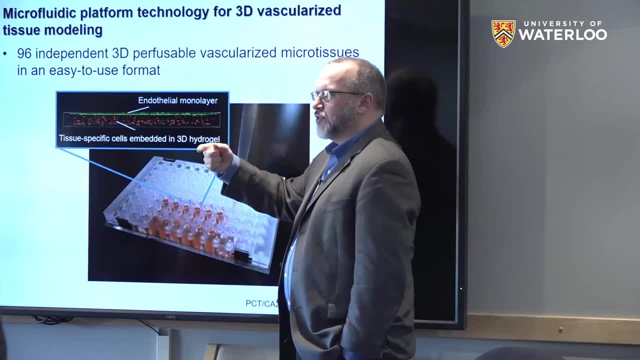 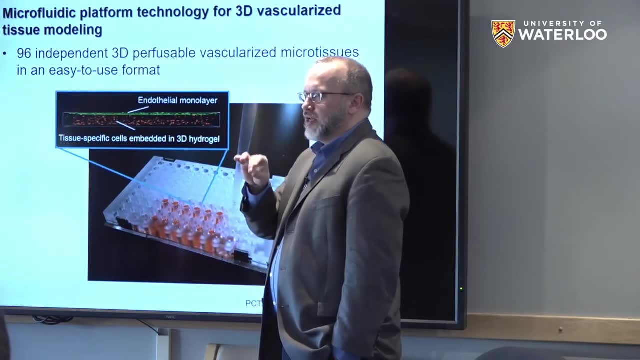 We're in collaboration with a clinician who has patients where there's a family, say, of three people. One person is normal, One person has a genetic mutation and has heart failure, And then the other person has the genetic mutation but doesn't have heart failure. 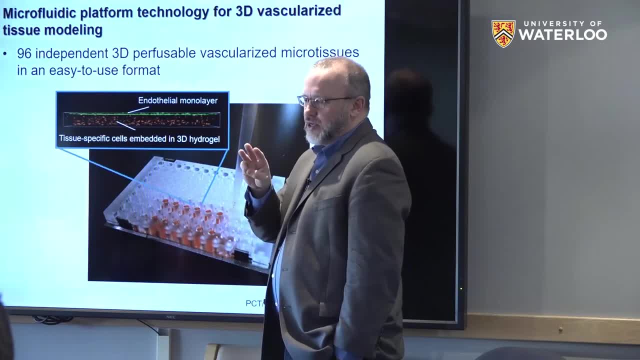 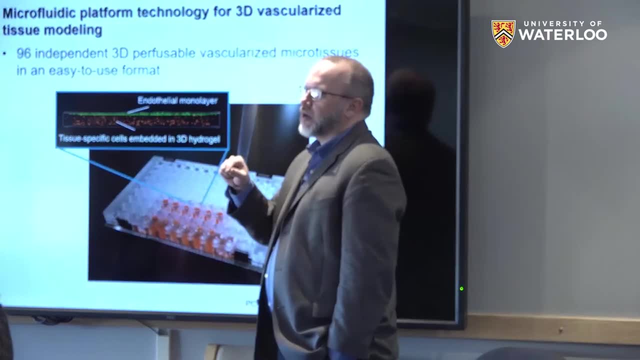 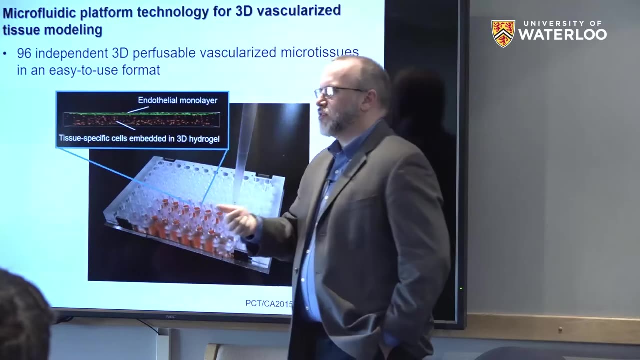 So you have this nice three like well-controlled samples. She's taking blood from those people, making induced pluripotent stem cells out of those and then differentiating those into cardiomyocytes. So the goal now is to now use those cardiomyocytes in the system to do disease modeling, to look at mutations in heart failure. 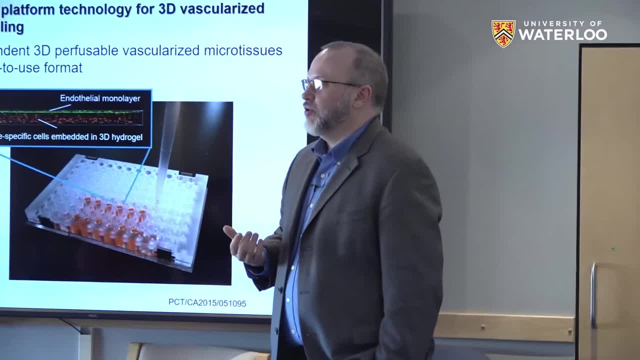 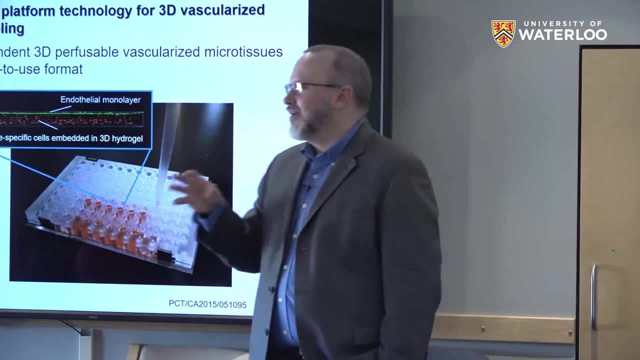 So that's one example. We could do the same with valve cells, for example. right, You could – now no one's done IPS to valve fibroblasts because no one's quite sure what they are, But you could imagine doing that, for example. 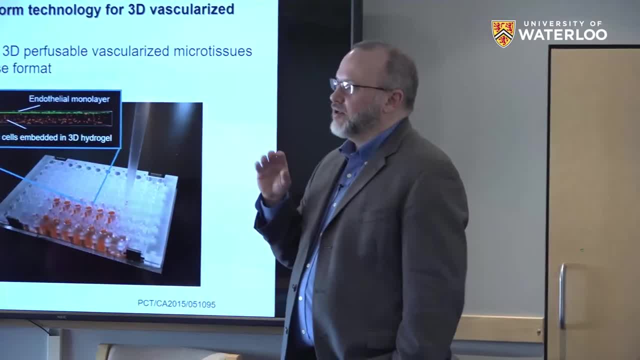 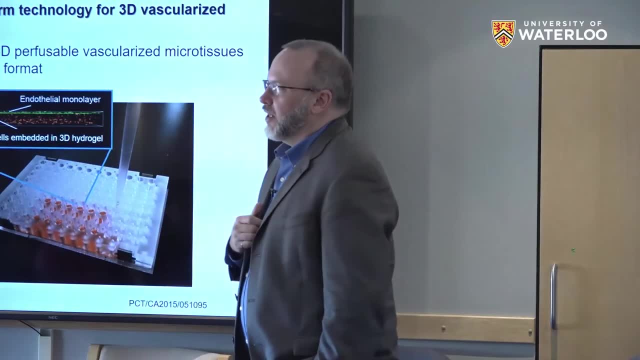 Or what you're suggesting. you could change the environment Right. You could put in, I don't know, higher cholesterol, Or you could use older cells, You could use male versus female cells, And yeah, those are just some of the questions we're starting to ask as well. 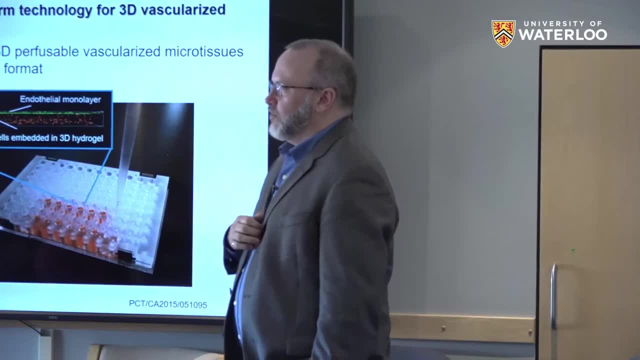 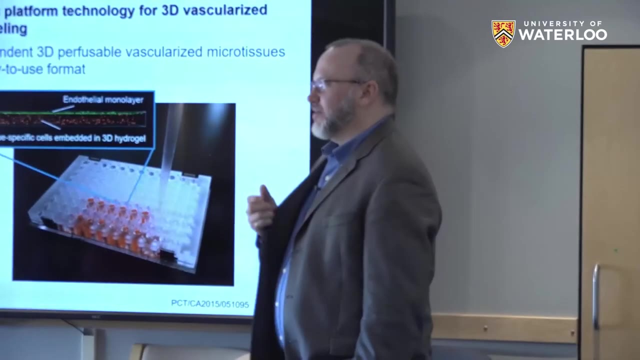 The male-female question is actually really interesting because the factor we look at CMP. Kristen Masters, who's a researcher in this area. she demonstrated that CMP was one of the highest differentially expressed genes in male versus females, So we're now starting to explore whether there's a clinical relationship. 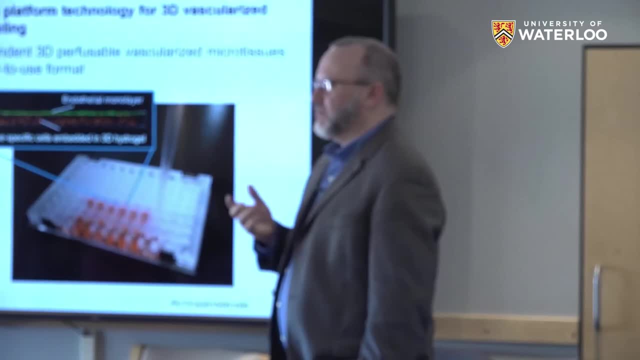 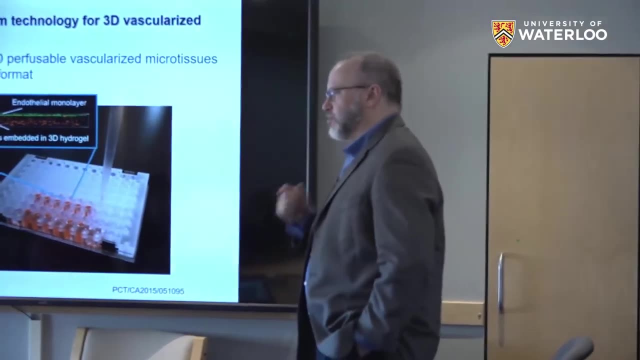 There's a clinical implication of that, because males and females' valves disease differently. So, yeah, it's quite intriguing. So we're actually – the male-female question we're pursuing exactly using co-culture systems and, yeah, Thank you.